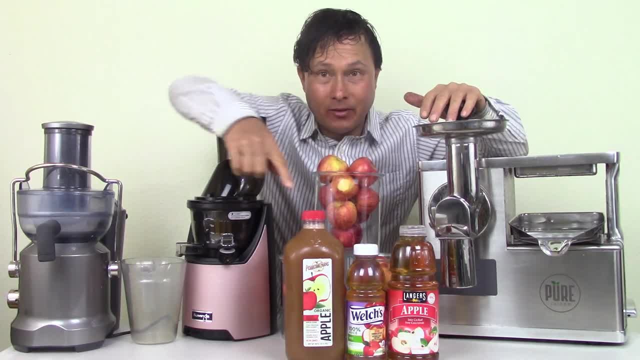 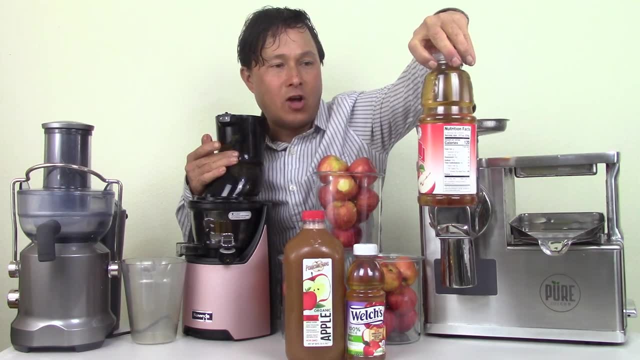 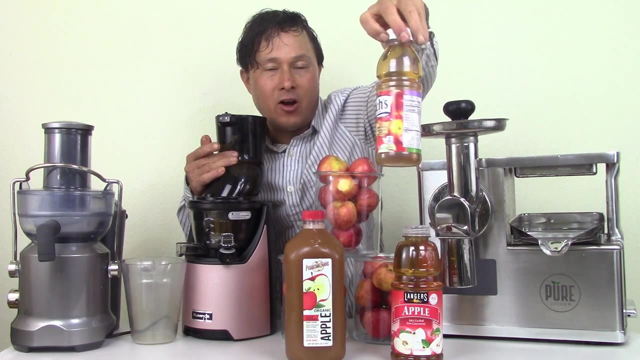 that's actually the healthiest apple juice. So I got a couple of examples here bought at a local store. We got the Langer's right. The Langer's, It says Langer's apple juice cocktail from concentrate. Is this good? Or is the Welch's apple juice? it says 100% juice. 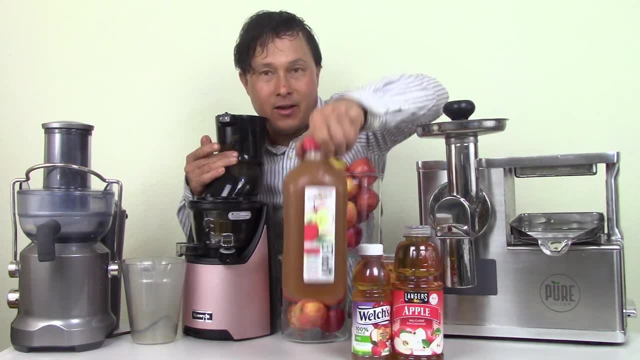 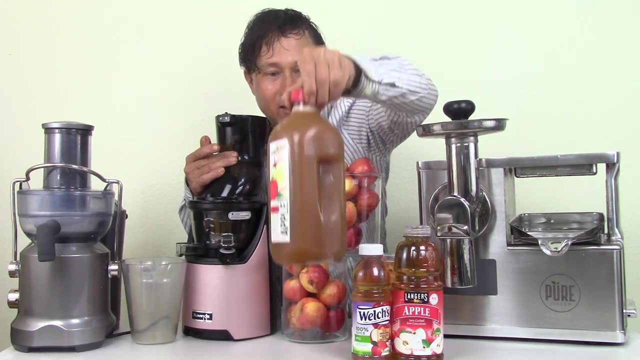 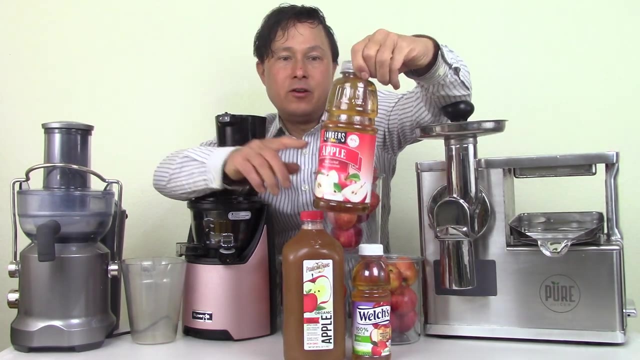 apple. Is that good? Or is this brand the organic one? organic apple cold prep- is this good? I say it's cold press, That must be good, And it's dark. Is that the better one, Right? So, first off, many apple juices sold in the store, such as this one, you know it. 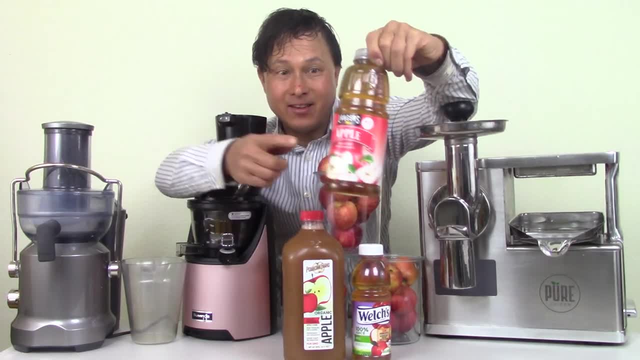 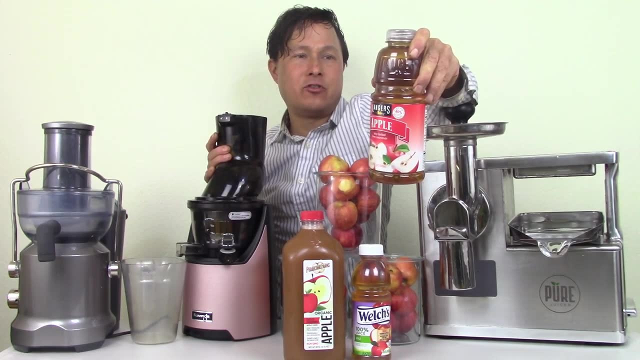 says it contains 30% juice. So wait a second. This is not really juice. It's 30% juice. What's the other 70%? You know well it's ingredients: filtered water, apple juice concentrate, sugar, citric acid, natural flavor, pectin, caramel color and ascorbic acid vitamin. 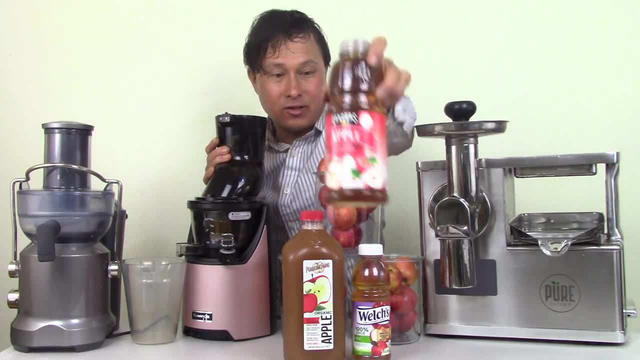 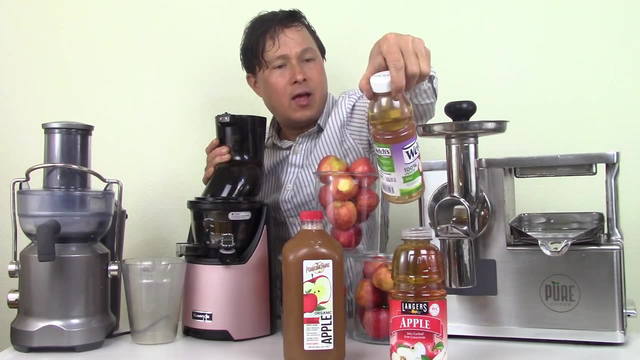 C And this is actually quite clear. You can almost see through it. It looks like kind of some pee. Next in line we have the Welch's. At least this says 100% juice And it is, you know, apple juice from concentrate filtered water, apple juice. 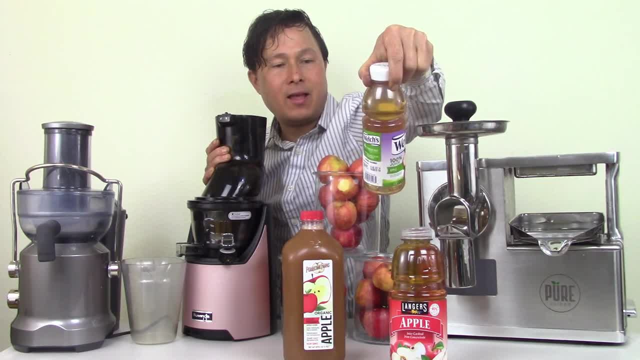 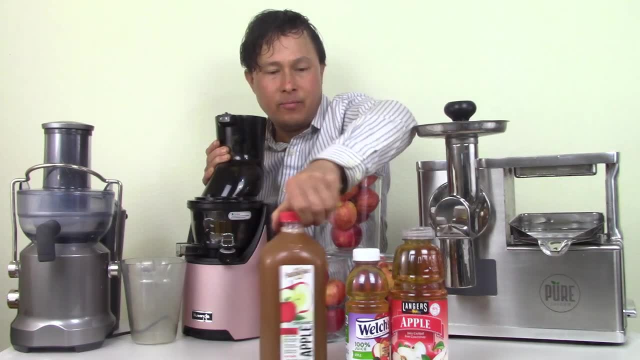 concentrate, ascorbic acid, vitamin C and malic acid for tartness. And then this one over here is 100% juice and the ingredients are simply just apples. So here's the thing, right: The more processing that happens to your juice and the other things added in. 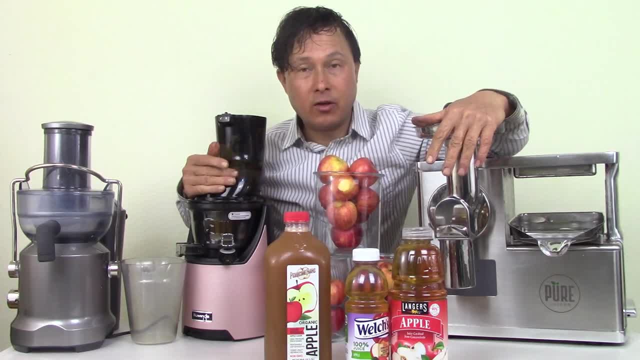 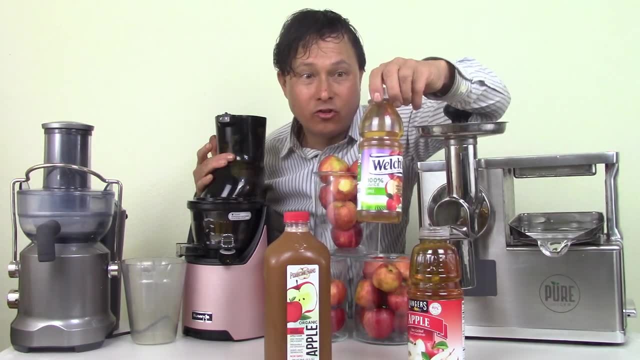 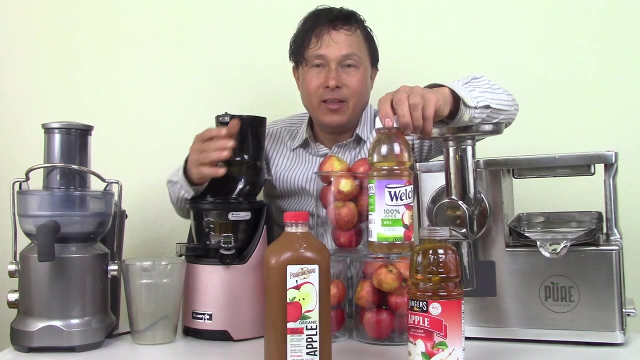 my opinion, lower the nutrition. Okay, I know there's some YouTube videos that say apple juice is worse for you than a Coke, And the 100% juice that's Welch's has gone through a process of being juiced and then concentrated and heated up and then reconstituted into this with other you know. 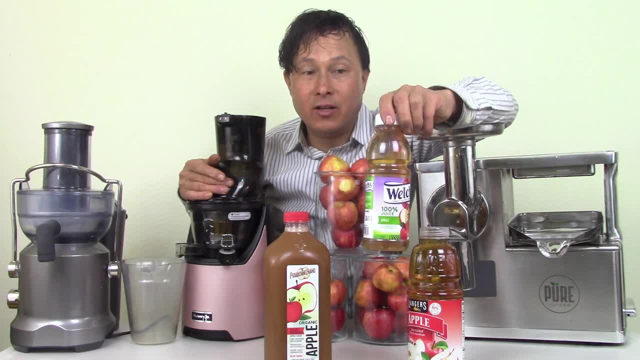 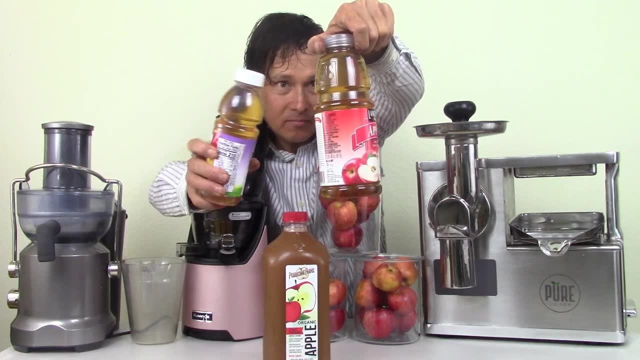 vitamins added, because they're probably missing because of all the processing And also, in addition, micro filtration. So I want you guys to pay attention to the colors of these juices, right? This one's probably the color of the juice. This one's probably the color of the juice. 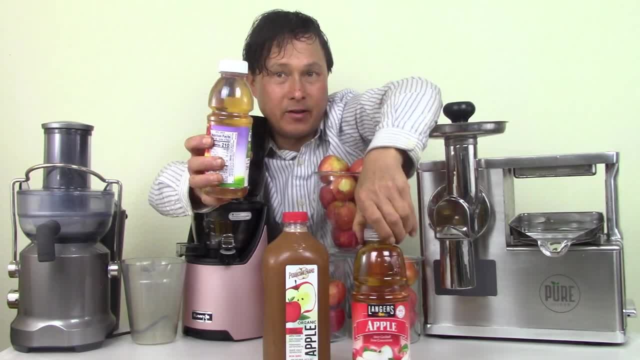 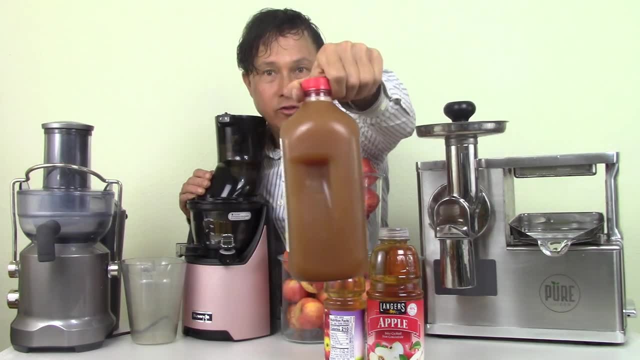 This one's probably the caramel coloring making it this color, But this color is just basically 100% apple juice. If you guys could see that, it's pretty much clear. And if we look at this one, this is the cold press juice- it's nice and dark, So I'll be pulling. 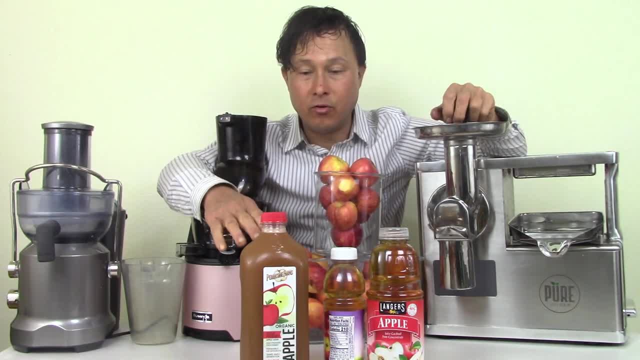 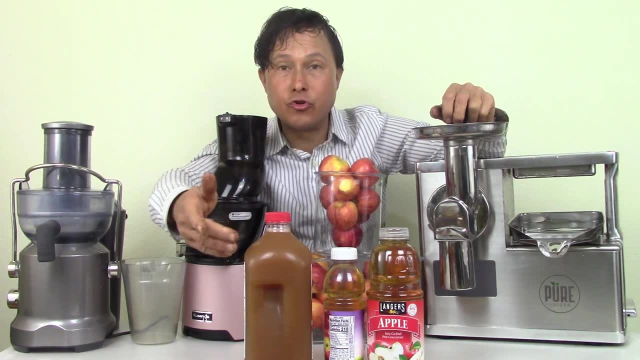 out. you know, basically, some science talking about the. you know how it's much more beneficial to have a more darker, you know unfiltered juice, because there are more nutrients, polyphenols and, more importantly, the fiber, the soluble fiber that dissolves in the water when you. 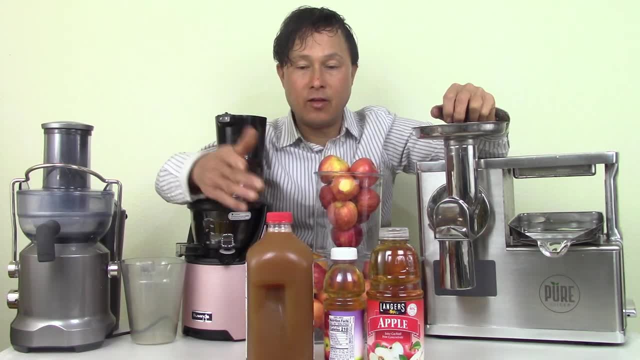 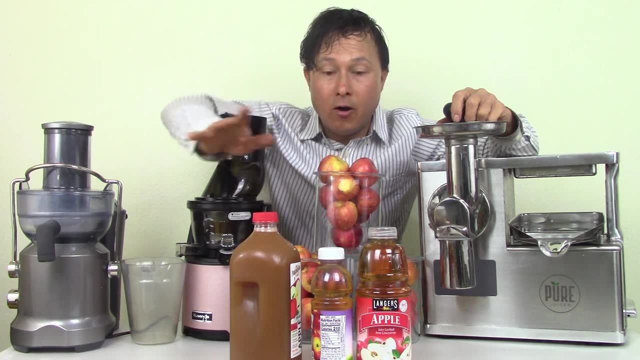 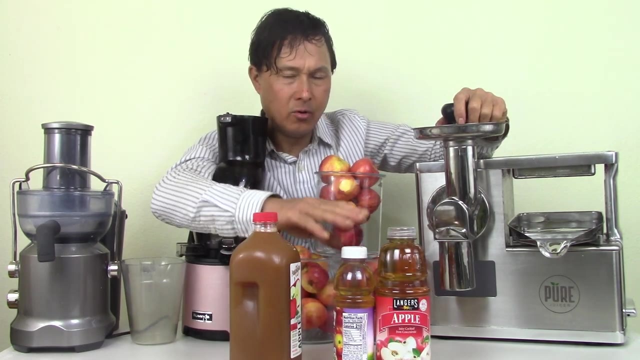 have more of a cloudy juice. So yeah, these are the commercially available ones. But you know what? Here's the thing: A lot of the studies that show apple juice is bad for you are based on juices that you can pre-buy, So these juices are shelf stable, you know. 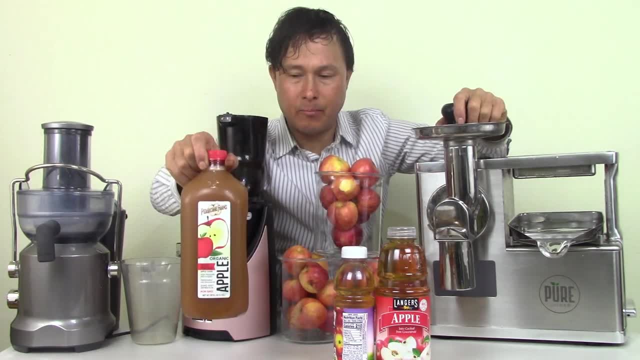 and are heat processed, whereas this one is cold pressed, needs to be kept refrigerated. So I'd definitely say you know if it has to be cold. you know kept cold it's going to have more nutrients than the, you know, cold pressed juice. So you know if you're. 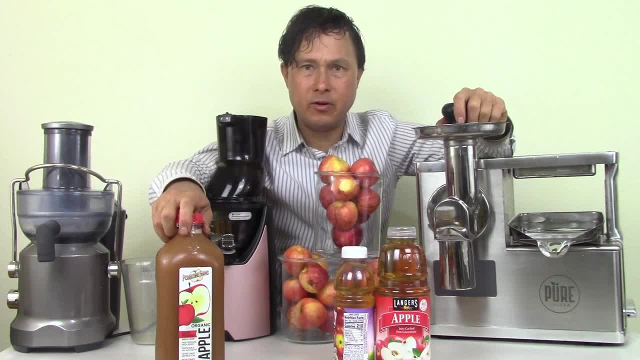 pre-buying this one. you know it's going to have more nutrients than the ones that are shelf stable. This has been HPP- high pressure processed, you know. so it will kill the bacteria and it'll probably, you know, keep some of the enzyme content, because it's. 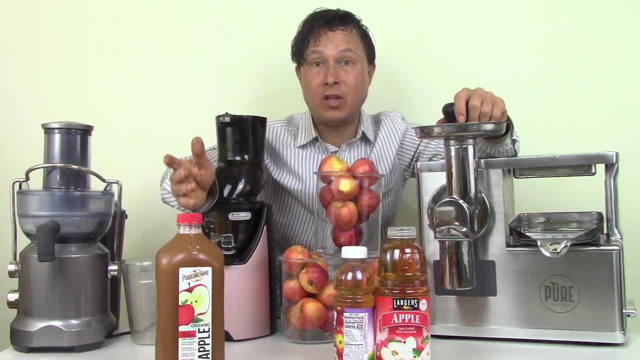 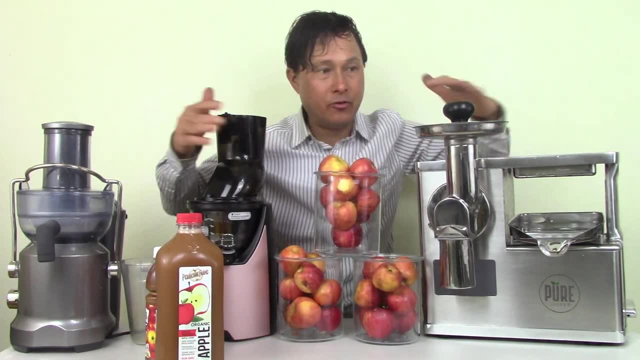 not technically being heated up too hot, although many juices can be pasteurized. That being said, when we're going to juice our own apples right here, right now, using fresh apples, using three different juicers, you know, I basically just wash the apples. These are: raw apples produce, not apple juice. So you know it's going to be a lot easier to use fresh apples than the ones that are shelf stable. This has been HPP- high pressure processed, you know. so it will kill the bacteria and it'll probably, you know, keep some of the enzyme content. 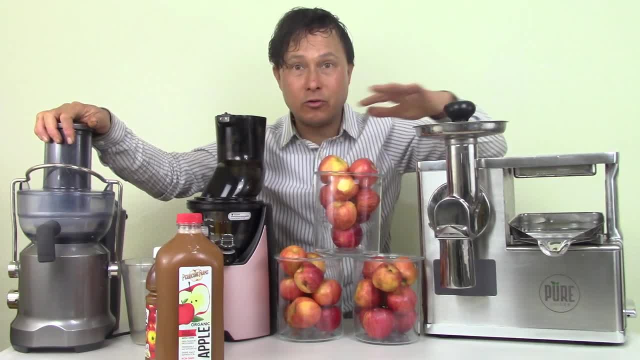 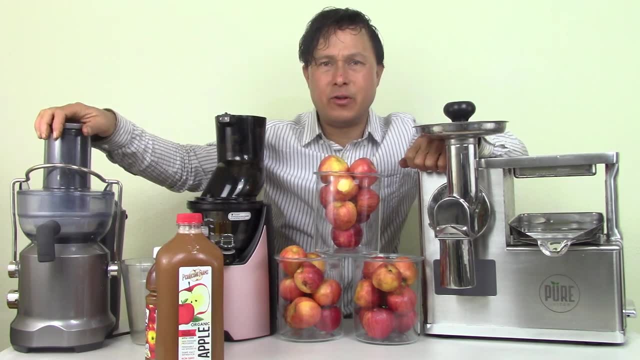 not heat processed. You know I'm not going to do any additional filtering to these juices, So we're going to keep more nutrition, We're going to keep more antioxidant compounds, We're going to keep more vitamin C. Some of these juices will keep more fiber, including 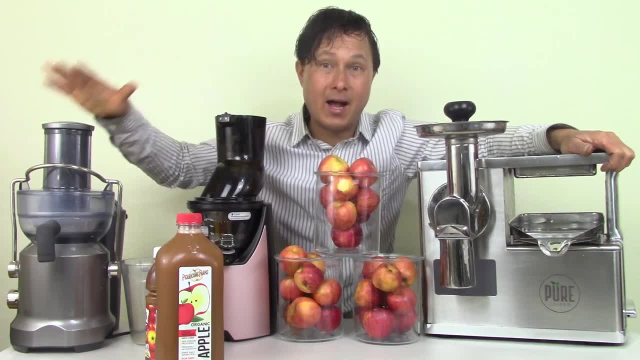 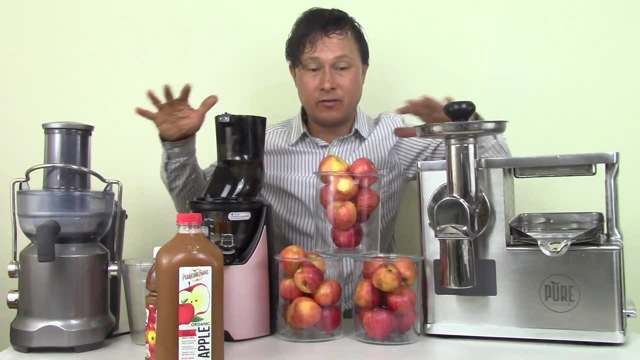 the soluble and insoluble fiber, and some juices will oxidize some of the apples as we create it. So I'm going to bring you guys along in the process and show you guys the process of juicing, More importantly, how long it takes. 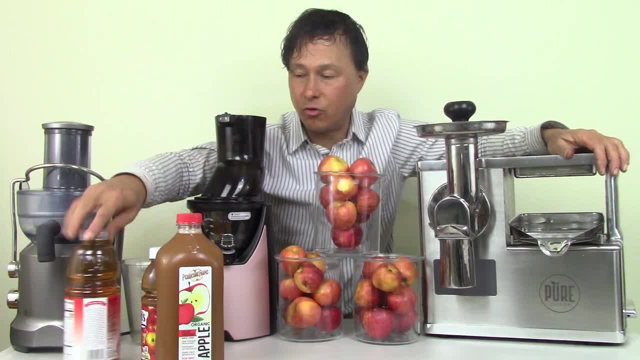 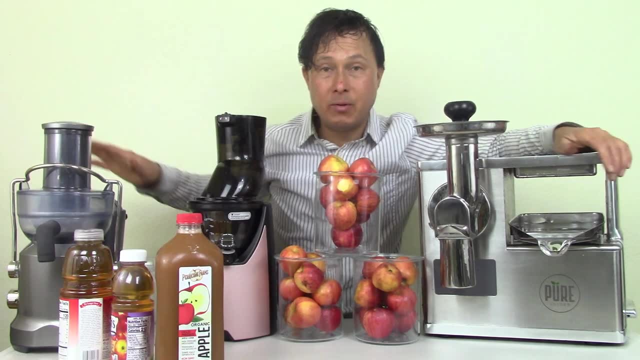 And also compare the results at the end to these store-bought juices that we have right here, so you guys can learn which one of these juicers makes the healthiest apple juice. And I'll be pulling out some science at the end of this episode to basically confirm what. 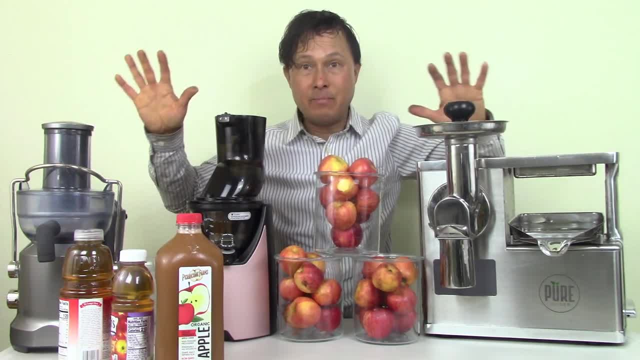 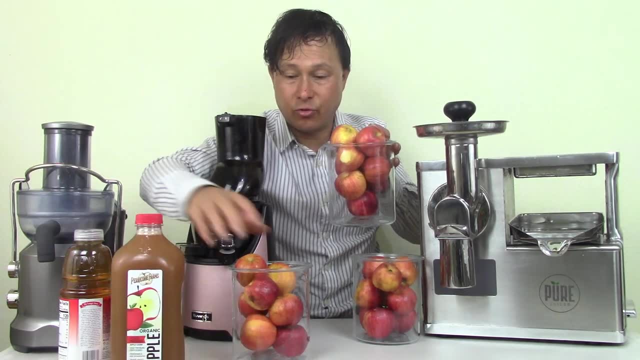 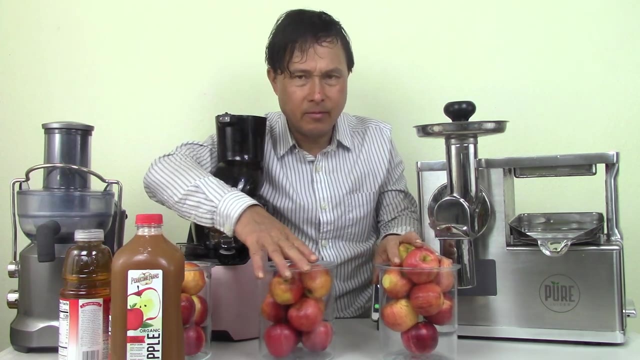 I'm sharing with you. All right. So this is not by any means a yield comparison. although I have pre-weighed out seven hundred and seventy three grams of apples in each one of these jars, You know that I will be juicing each in each one of these machines. 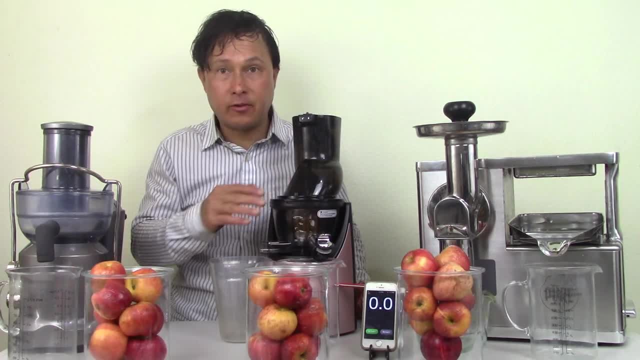 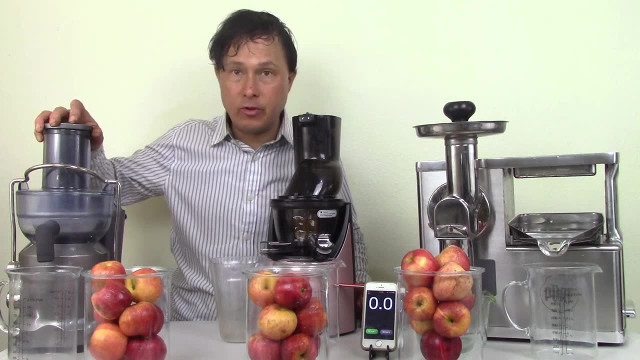 So now we're all set up ready to juice. We got all the collection cups for the juicers all set up ready to go. Let me go ahead and introduce the different juicers I'll be using today. First I'll be using the Breville Juice Fountain Cold, While this is a called cold. 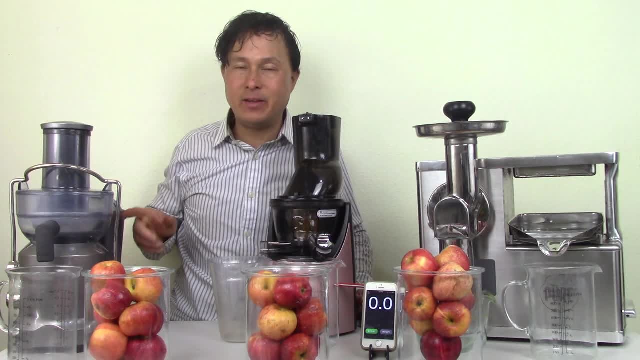 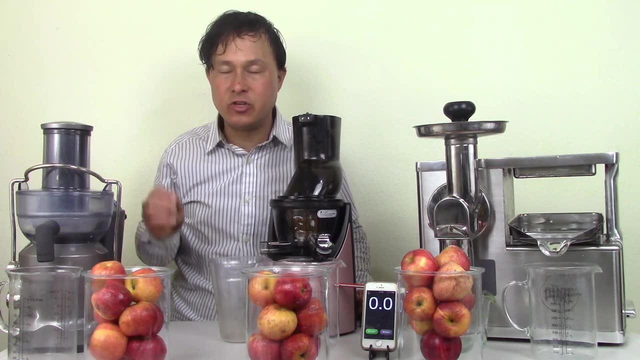 in the title. it is not a cold press. It runs at a high speed and oxidizes phytonutrients as it's coming out. It runs the juice out of the machine, You know. so I'm not a big fan of this style machine. 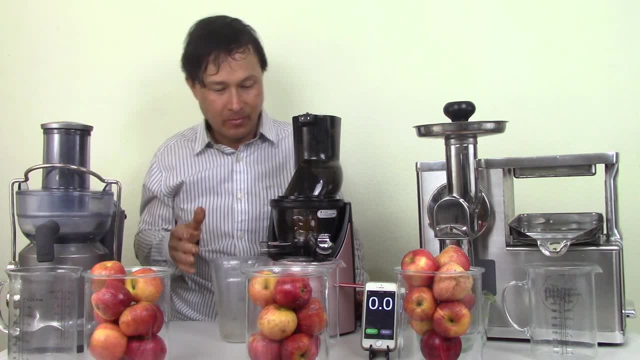 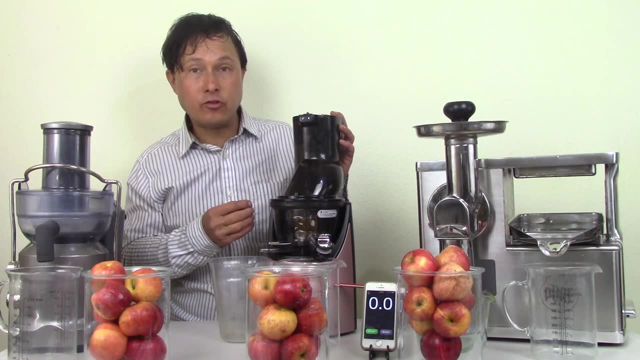 and I only use it when I'm making demonstration videos like this. Next we have the Kuvings EV0820.. This is a slow juicer, cold press juicer, and it is made by Kuvings. It has a wide three inch feed chute, which I like a lot, So I'll be able to just dump the whole. 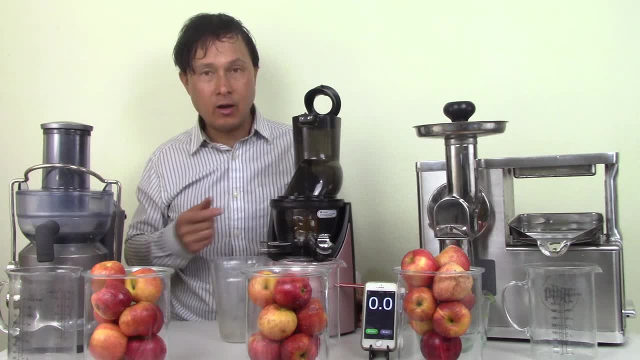 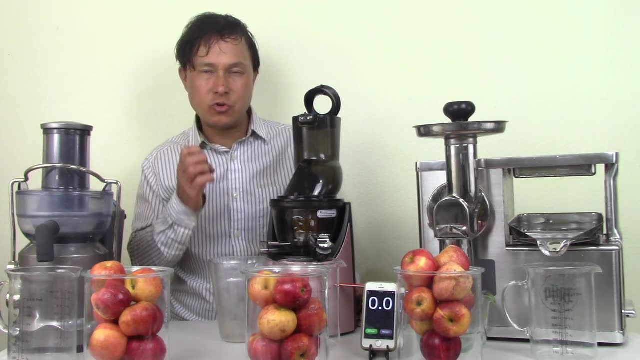 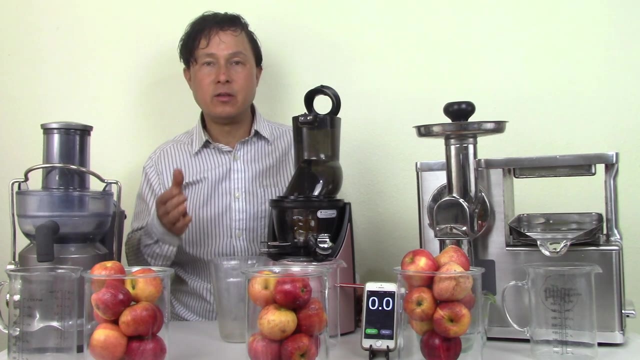 apples in there without any kind of pre-cutting. It runs at a low and slow RPM- I think it's around 60 RPM- So it literally crushes and squeezes out the juice with very little oxidation. It will leave more pulp in the juice being insoluble, as well as the soluble fiber. This 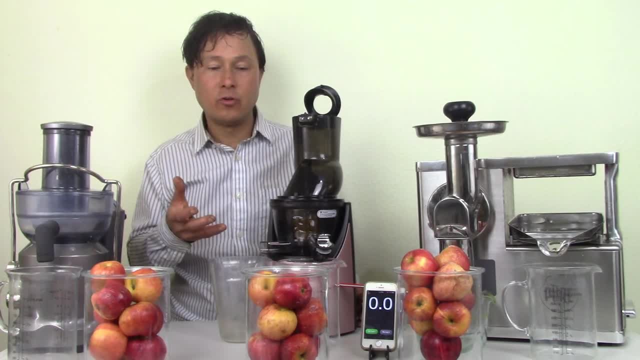 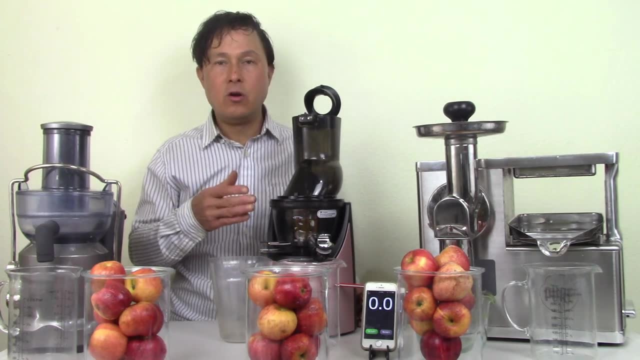 is the style I personally use at home and other slow juicers you know may work similar to this. Although the vertical slow juicers are best if you want to juice straight fruits, other slow juicers such as the horizontal or the twin gears can literally run up to. 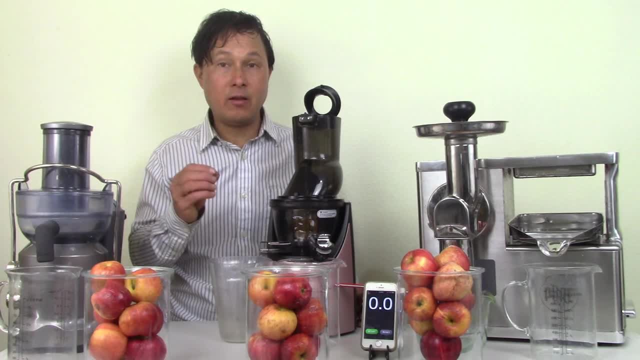 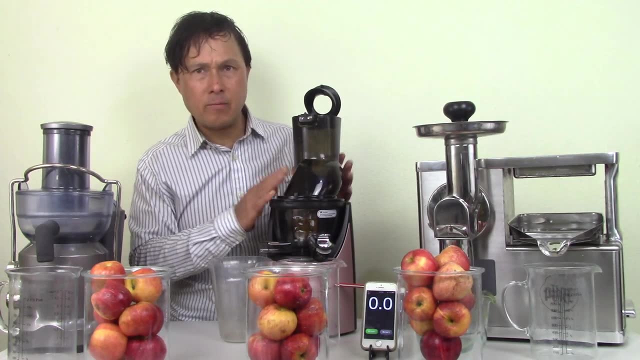 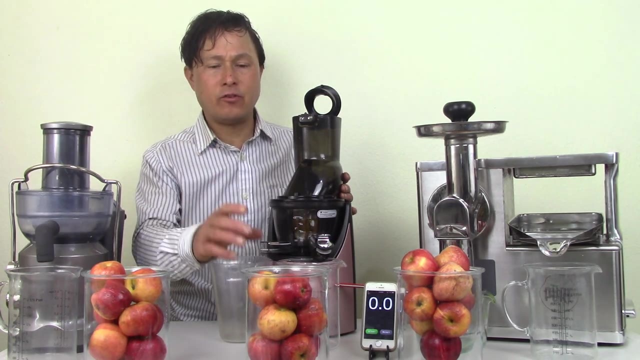 the juice. I personally choke on juicing straight fruits because the fruits can be too soft, All right. Also very important when using any slow juicer. always very important to select the most hard and firm apples as possible. If you select soft apples, mealy apples, old apples to juice. 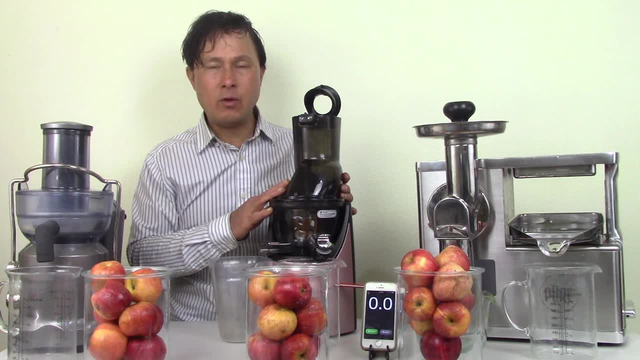 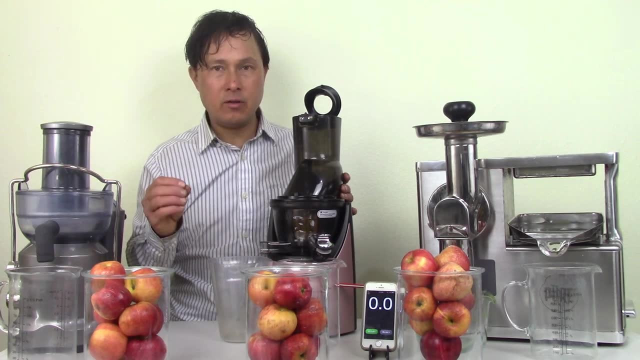 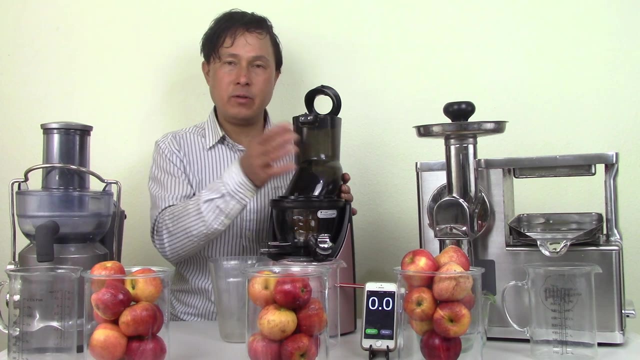 in a slow juicer, specifically any type, it will result in more of an applesauce consistency. This can be an issue when you're buying apples about now, you know, being it, you know, February or March or April. Apples were harvested last year in September, being being, you know, sitting in cold storage. 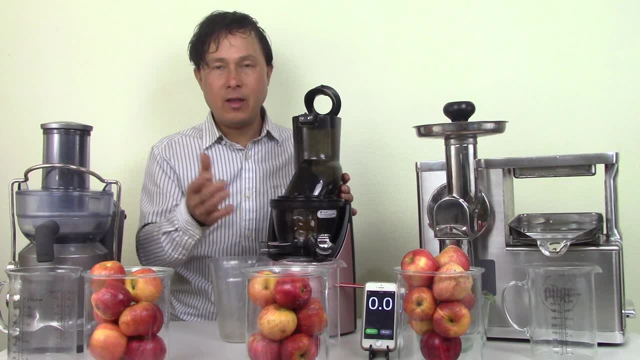 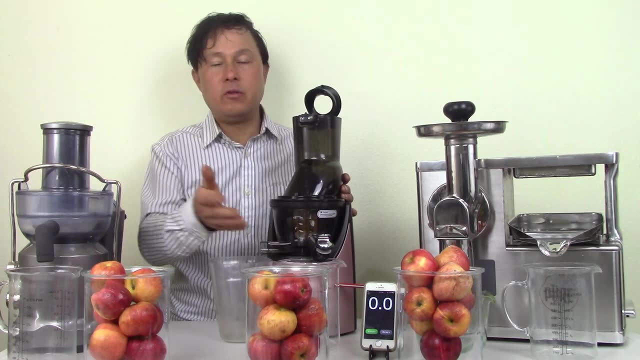 in an oxygen deprived environment and they sell it to you now and they they basically they're old so they don't juice as well. So, if you like, my performance is going down on my juicer. John, you know, it's probably the produce that you're juicing, If you're. 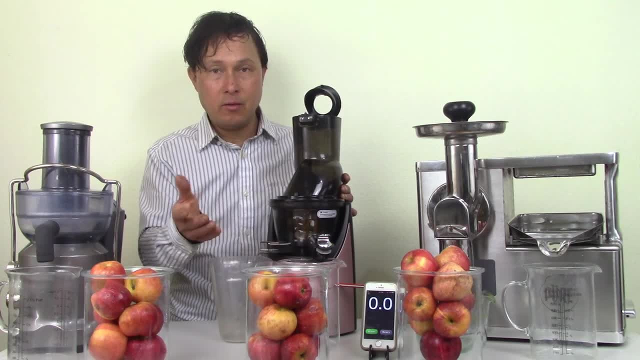 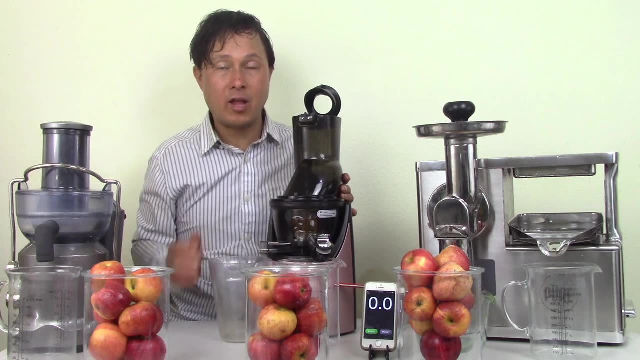 juicing apples. it will get more, you know, thick because of the older, softer apples you're using. So make sure you use Granny Smith. that will minimize that issue, but still can be problematic. Alright, And finally, over here we have the Pure Cold Pressed Juicer. This is the best. 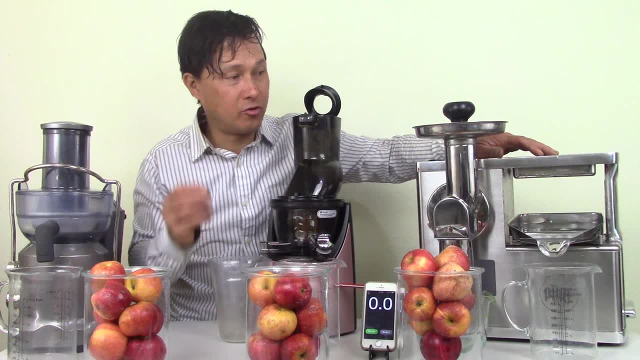 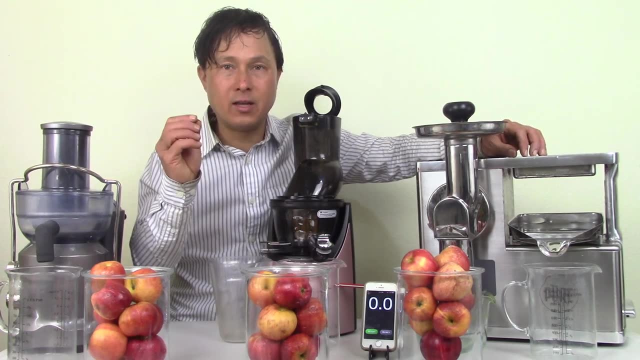 two stage hydraulic cold pressed juicer that literally presses out the juice. So if you think about, like how do they make apple cider or how do they make apple juice in the olden days? Well, they ground up the apples and then basically they used a, a a jack or a a screw. 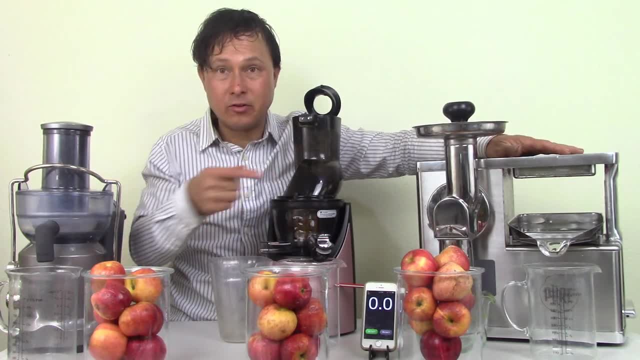 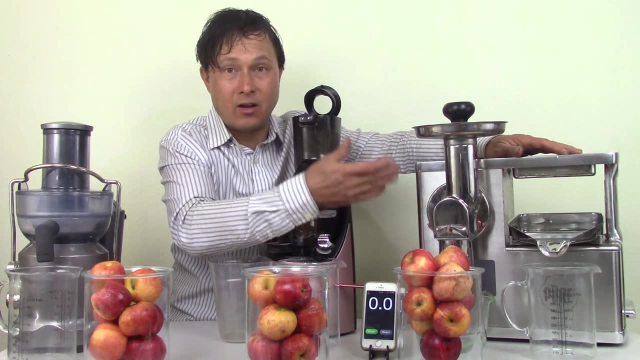 that basically pressed out the juice. So this is a a process similar to the to probably all the juices that I've. I've showed you guys. the commercial ones are made in a you know, press, a grinding and pressing style process, with probably additional steps. 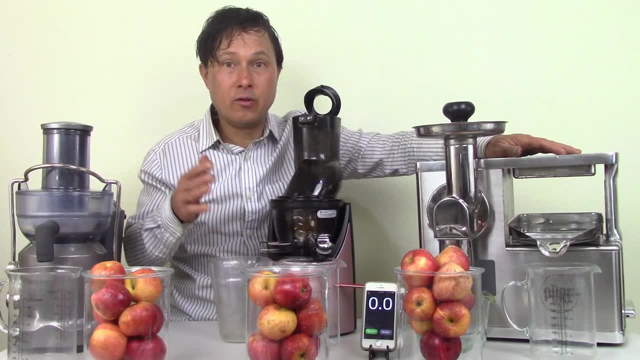 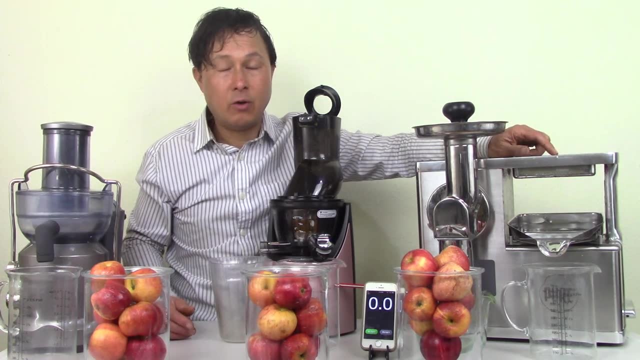 Whether that's HPP, you know concentration or you know extra filtration. I'm just going to be using the standard press cloths that come with the Pure machine And I want to say right now: this will get the highest yield and this is the best machine if you have soft. 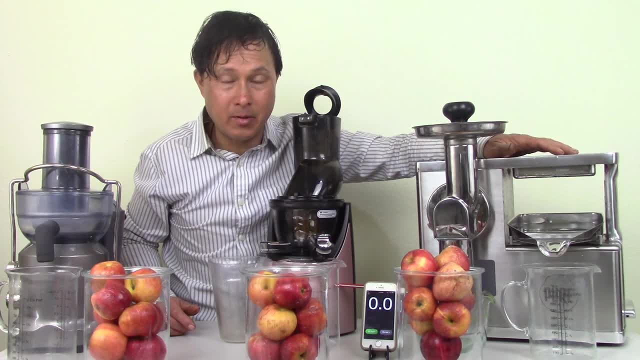 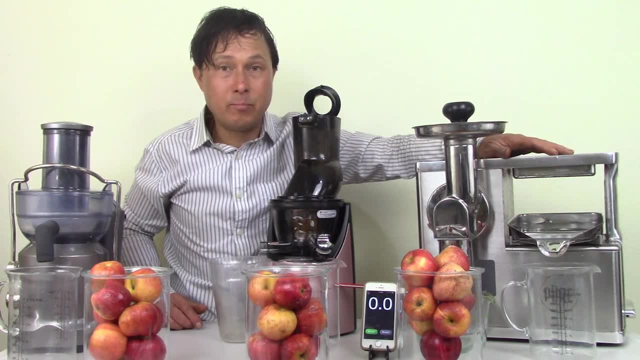 actually had about 200 caps of the Pure that were over-ripe and I would not dare juice them in any other machine aside from the Pure. So every different juicer has its pros and cons And while you will see that the Pure has a really good pro, because it probably 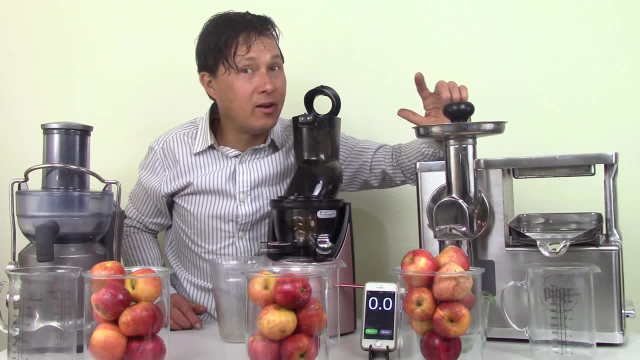 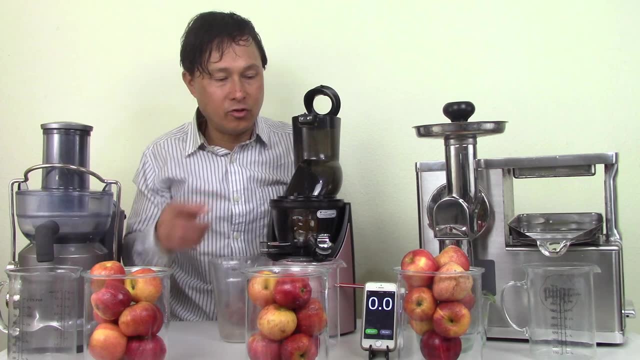 is going to make the highest yield. There will also be a con that you're going to have to stick to the end of the episode to learn about, Alright? So, any case, I've introduced the juicers. next step is we're going to get juicing. So we're going to ahead and use a 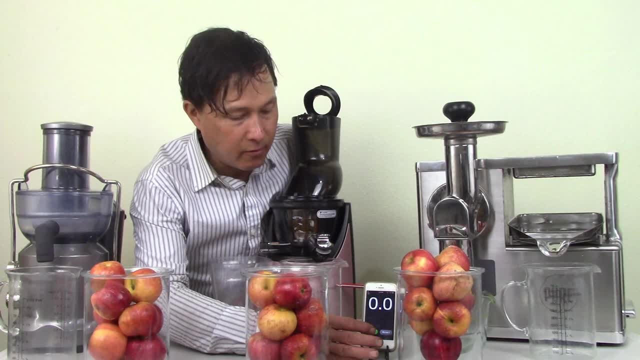 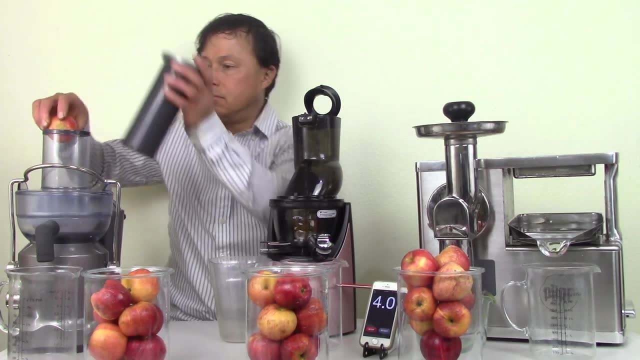 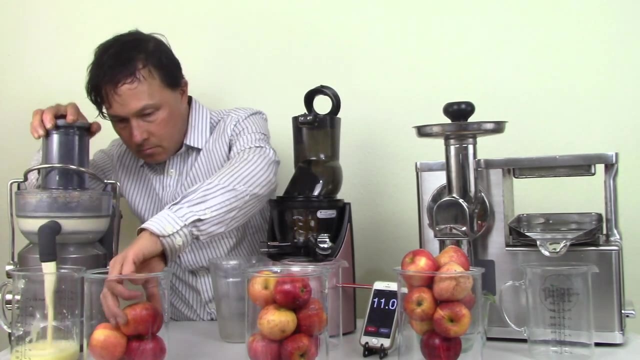 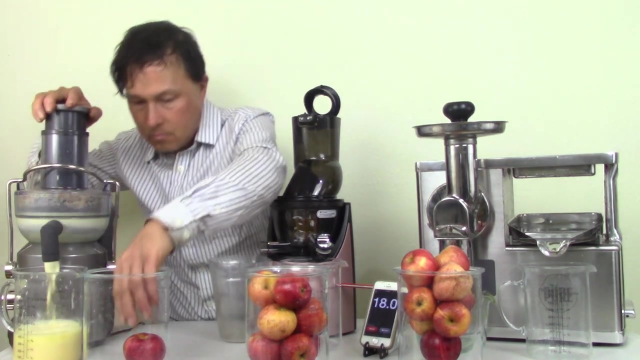 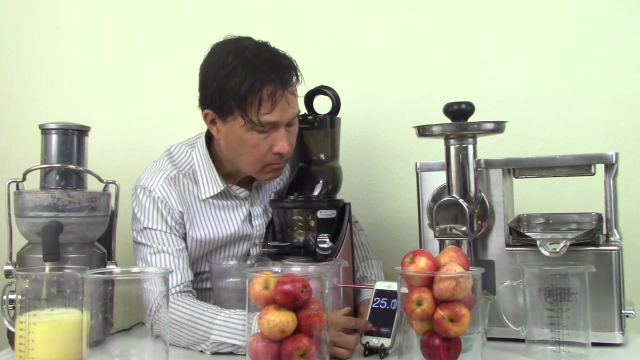 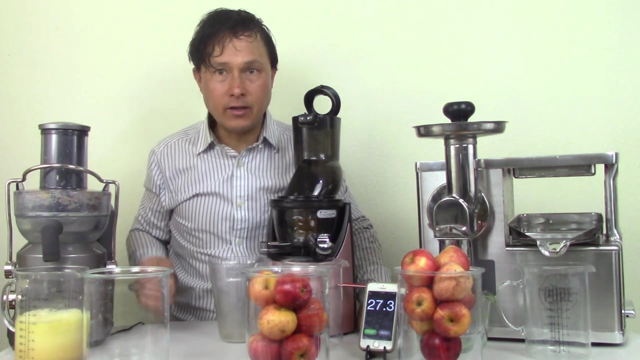 stopwatch and time this. We're going to go ahead and start with the Breville first and I'll probably speed this up to save you guys some time. time Alright, so I'm all done. I don't know if you guys can see the time on there, but it's. 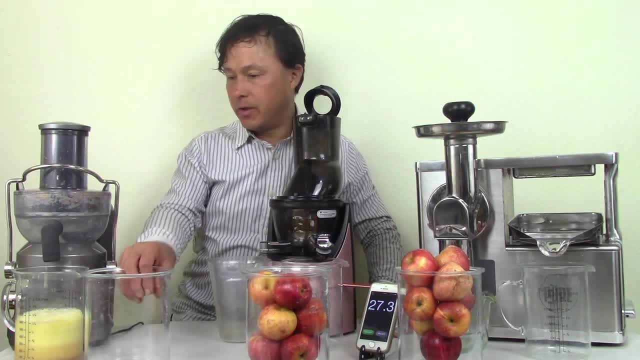 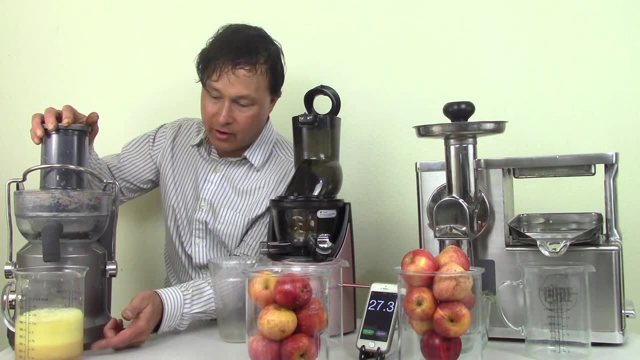 basically 27.3 on. there happened really fast and look what we got. we got you know, in my opinion it's a highly aerated juice. we have basically lots of froth. there's more froth, actually, than the juice that was created and I'll hold this up because this will change. 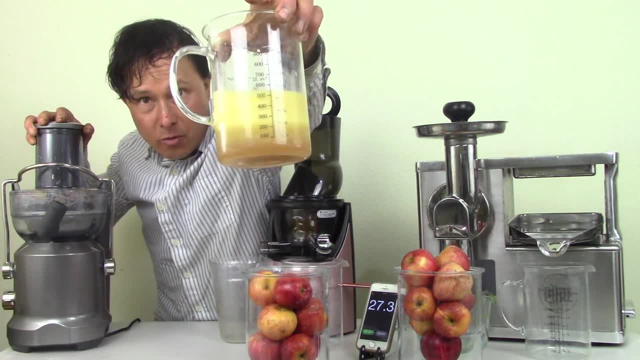 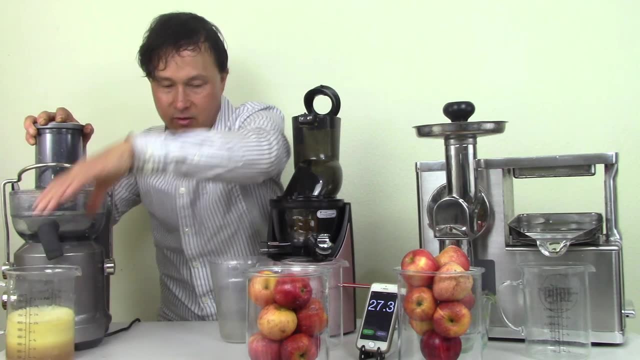 over time. the juice that we just created was almost see-through, kind of similar to the, you know, commercial juices. alright, But it took about 30 seconds to juice this much and I don't know how much is in there because, honestly, I can't tell, because it's a lot of foam, alright, 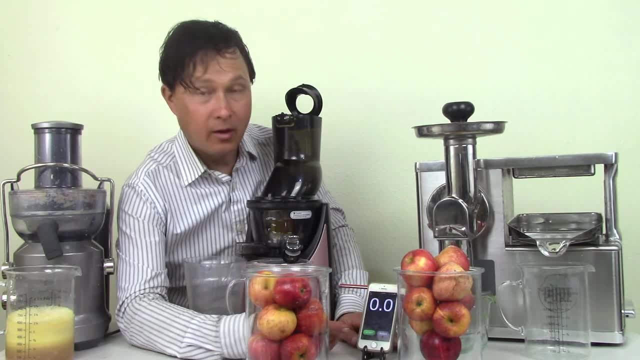 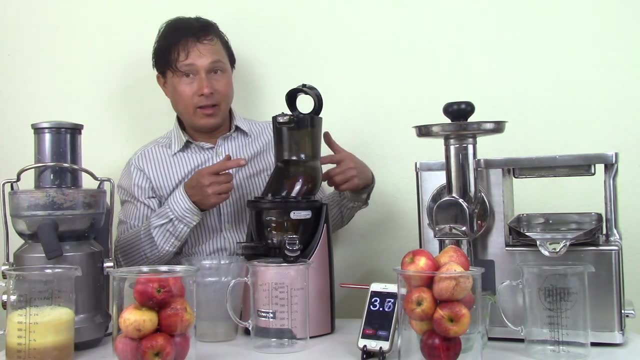 So next, let's go ahead and reset the stopwatch and we're going to go ahead and juice in the Kuvings, hit the start, turn it on and just drop in one apple at a time. We're going to let the machine process one apple and wait for it until we put in the 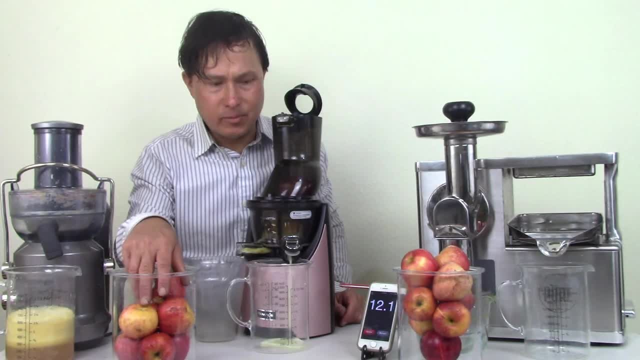 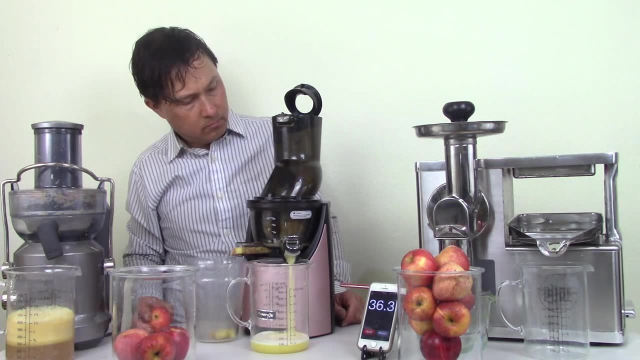 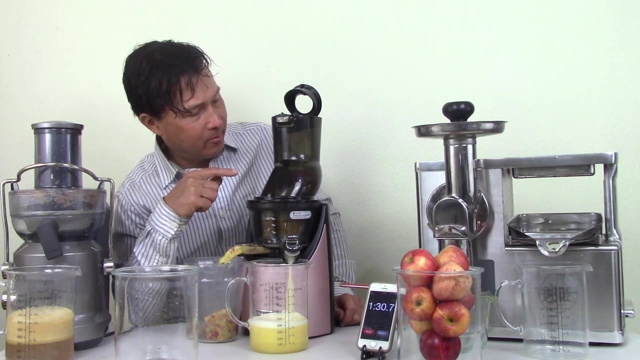 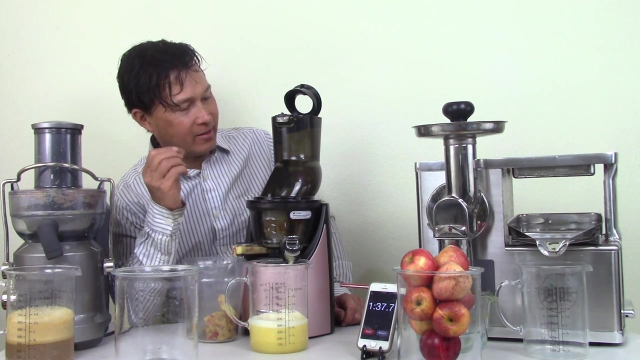 next apple. Once again, I will speed this up for you guys And alright, So come back at you when we're about finished. Alright, we just put the last apple into the Kuvings, and sometimes the apple will sit on top of the auger and kind of like not go in until it finally kind of hits a little. 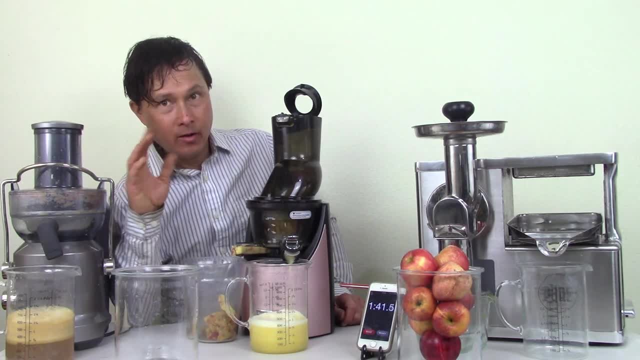 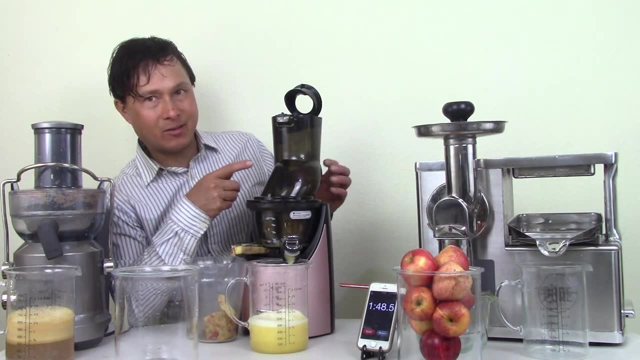 bit and then it starts getting chopped up, and then it'll get chopped up more and more. Now, one of the things I don't like about the wide feed chute machines on the slow juicers is that there will always be some kind of excess pulp. 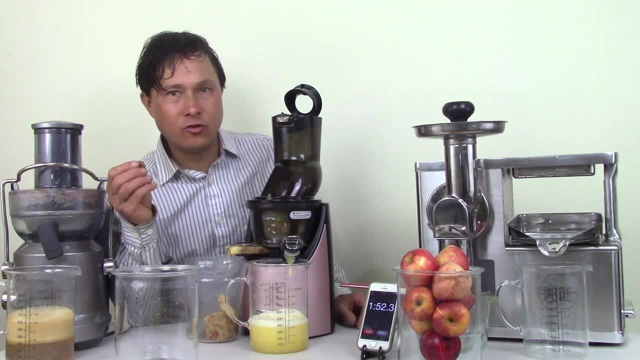 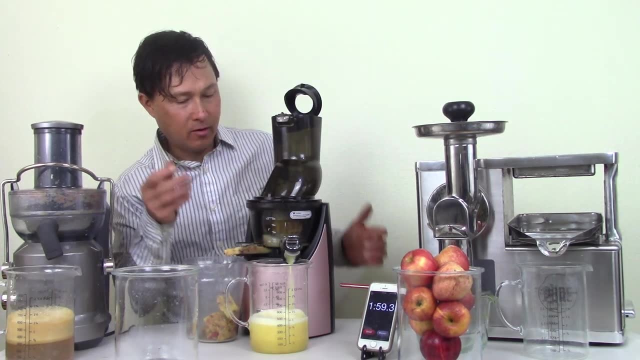 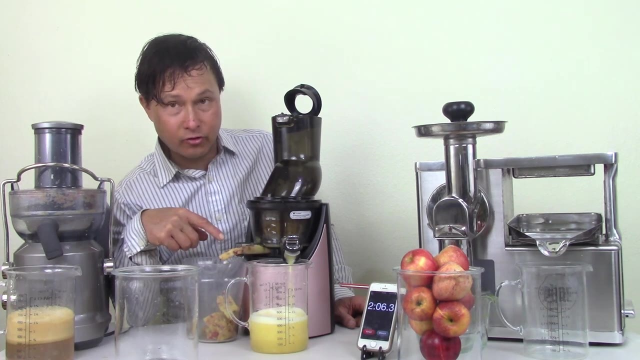 Stuff in the top of the mechanism that does not get juiced, and this is a trade off you know that you're going to have- for having the wide feed chute that you can dump in large apples too. This has worked a lot more slowly, created actually a fairly dry pulp that I'll show. 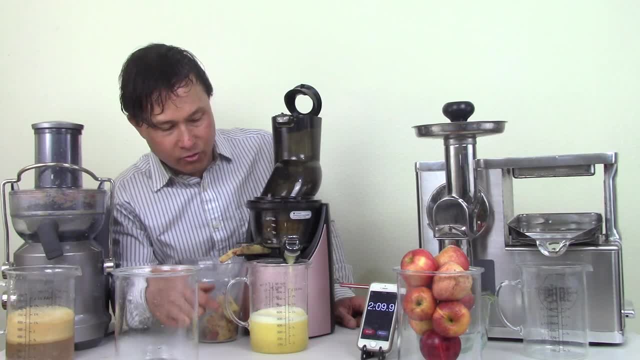 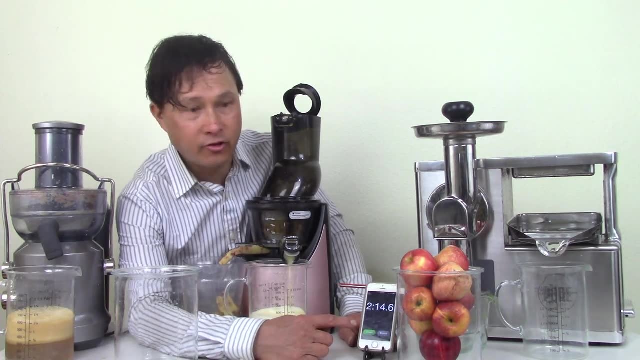 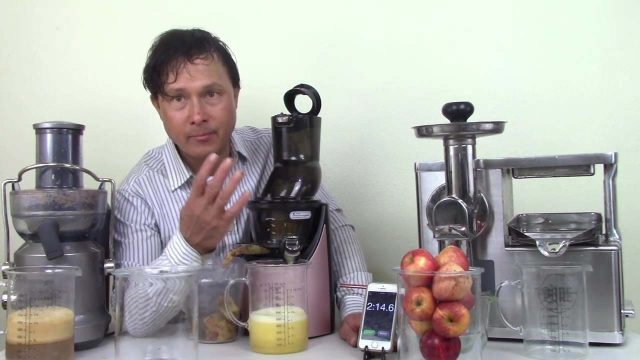 you guys at the end and actually we've created a lot of juice, So we're just going to go ahead and maybe stop this. and it took actually a wee bit over. It took 2 minutes and 14 seconds. so say it took 2 minutes. you know that's 4 times. 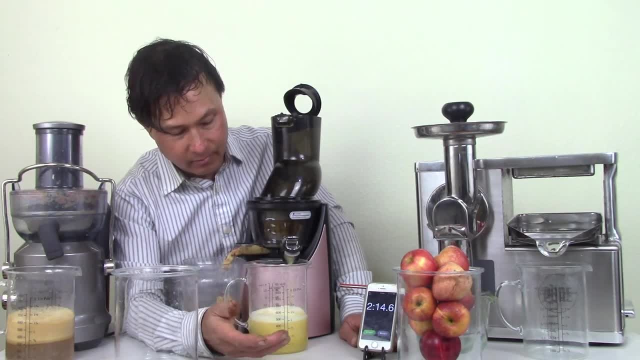 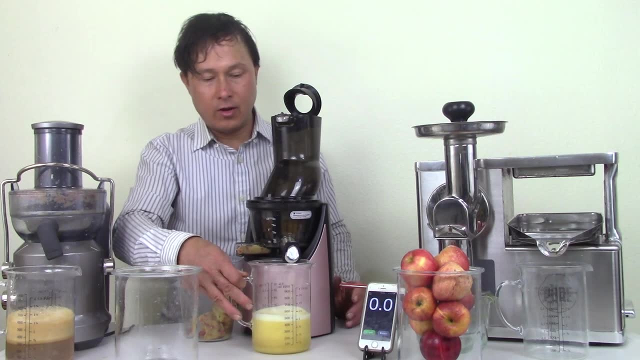 longer than the Breville. but you know, looks like we got. you know something a lot different. you know with the Kuvings. So let's go ahead and shut this guy off, and I want to show you guys what this juice. 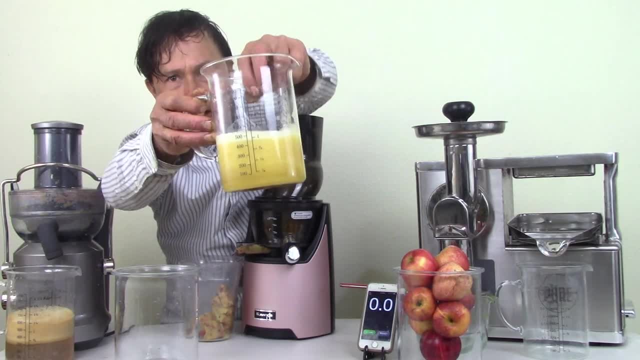 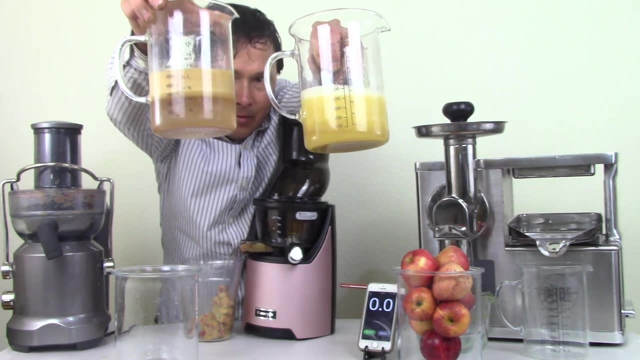 looks like. So you guys can clearly see this juice. yes, there is absolutely some foam in there, but if we hold this up and due to the high speed you know, all the apple juices will oxidize. but you can literally see on the bottom of this juice. 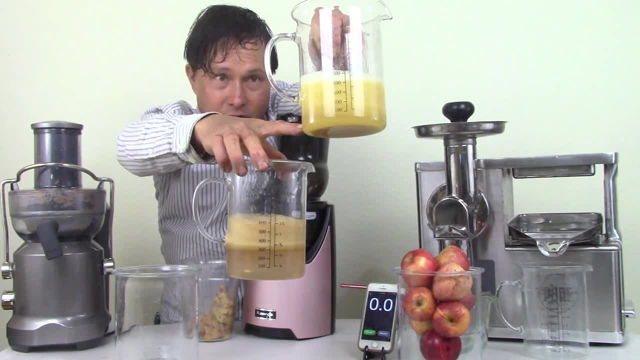 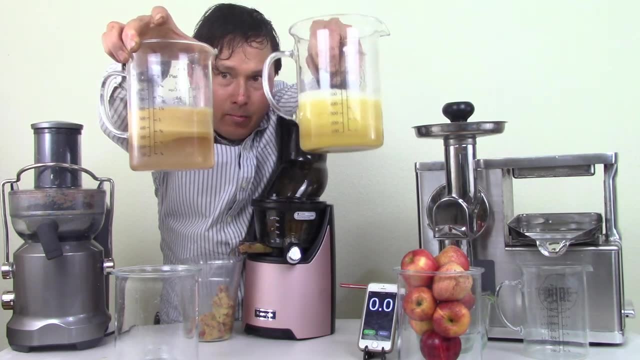 It's almost it is. it's almost see-through. bottom of this juice is actually quite cloudy. This juice is already browning. this juice will start to brown probably in a little bit, but there's significantly more foam in the Breville juice, you know, than the Kuvings. 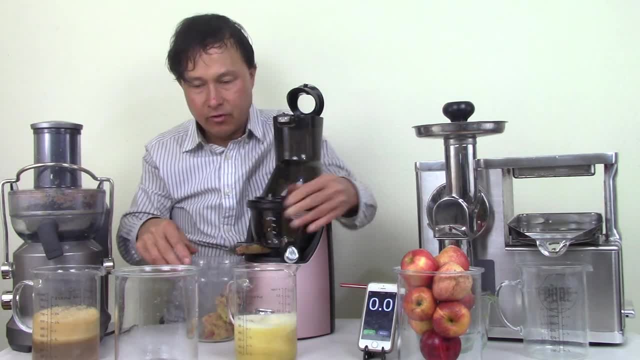 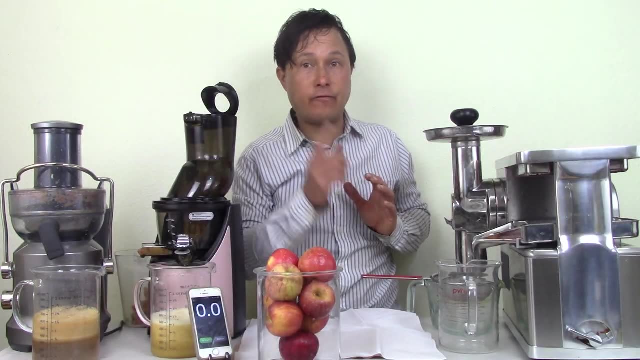 juice. So this will be very important. you know, aspect of the juices that I'll be talking about in just a little bit. Now I'll be juicing in the pure two-stage juice. The first step is grinding, the second step is pressing. 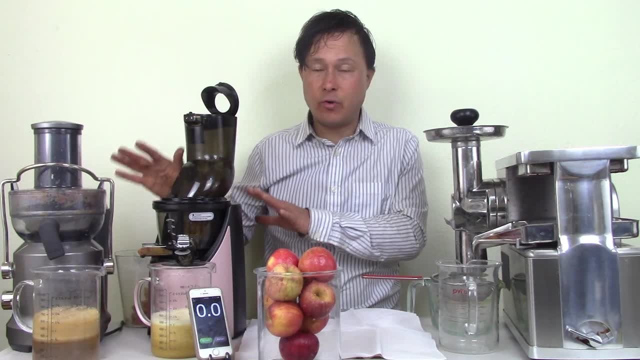 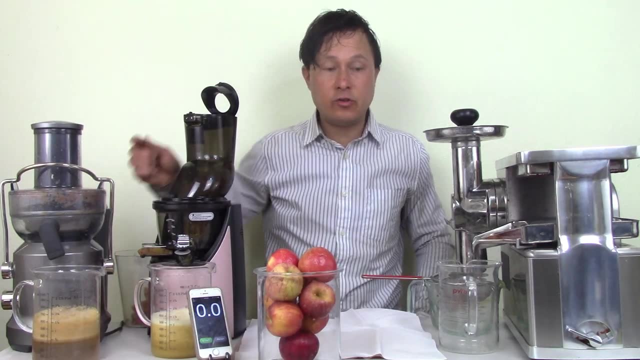 You know These are single-step juicers, whereas they are continual, so you can keep putting produce in it until the pulp bin gets too full. You can continue to juice. This is more of a batch juicer, so you got to like: put produce in, press it out and 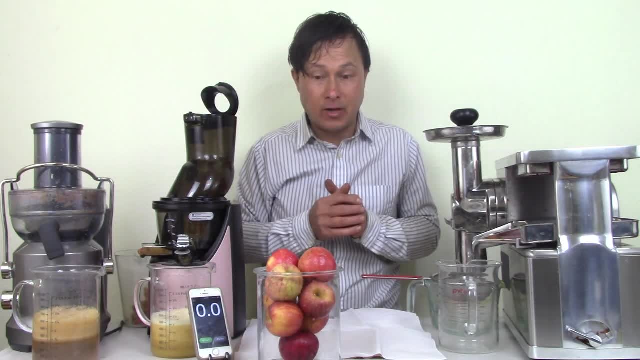 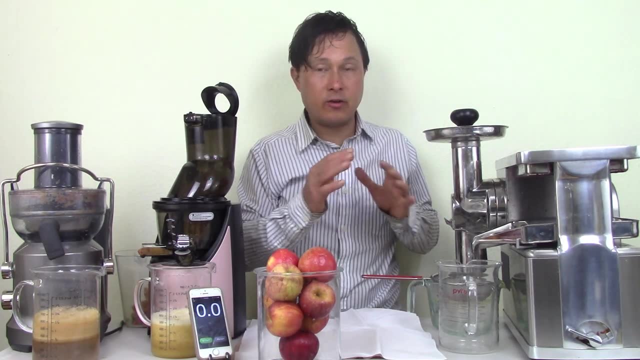 then you got to do more. You know this can also take some time, so we're going to learn how much time it takes and also see how much yield we get, And meanwhile I'm going to fast-forward all this because I'm not going to explain the 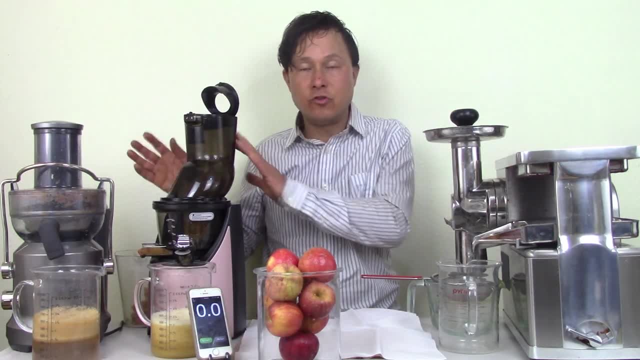 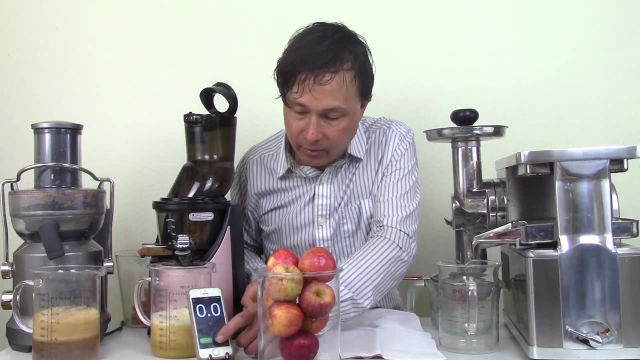 process. I have other videos in-depth on each of these juicers. I'll post links. I'll put links down below. if you want to learn more about each of these specific juicers on their own, All right. So with that, let's go ahead and hit start and let's go ahead and turn this machine. 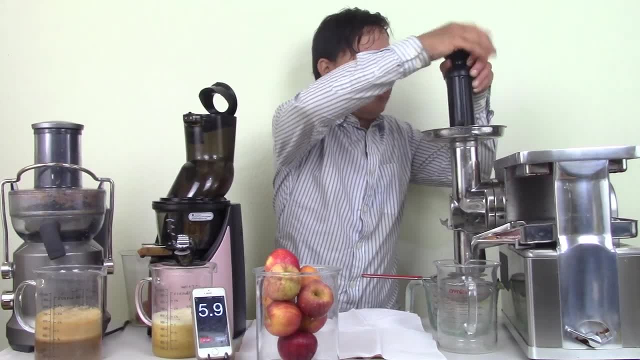 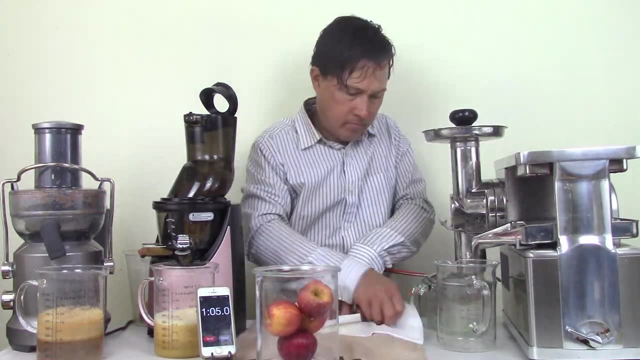 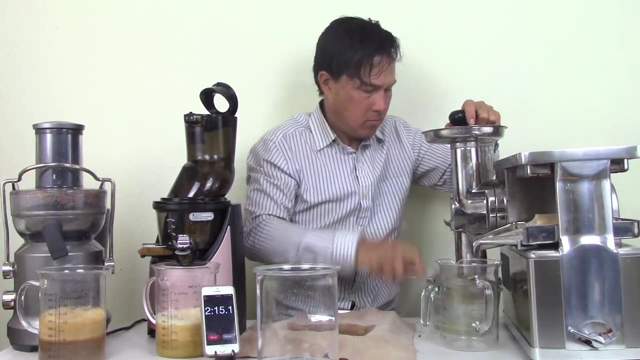 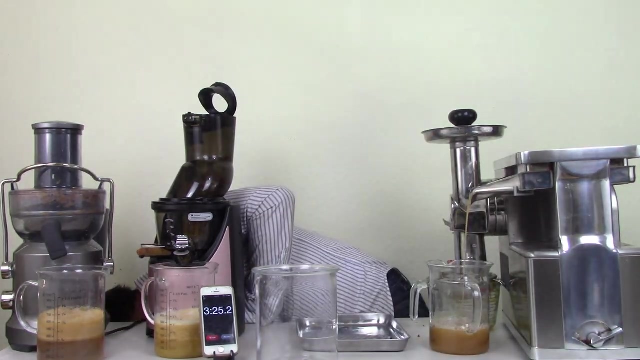 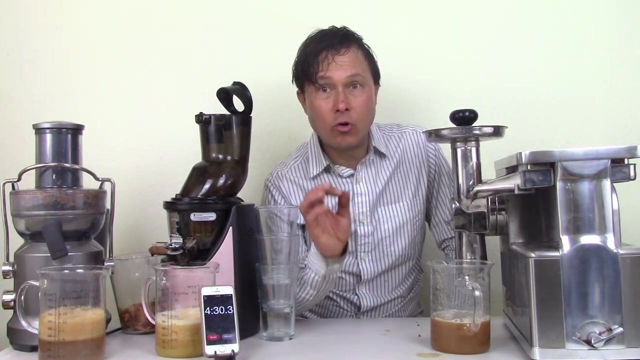 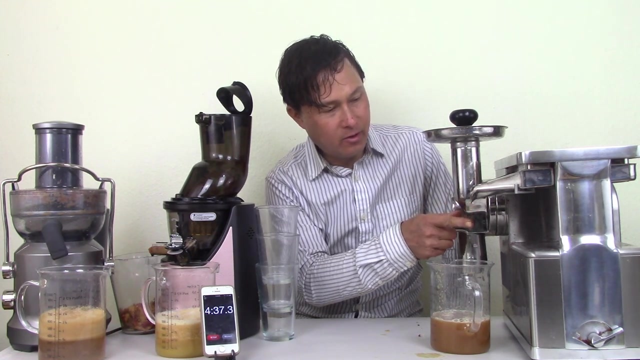 on and let's go ahead and put the apples right into the machine. All right, so we're almost done juicing in the pure. We basically pressed out the apples and the goal is to wait until the stream breaks. Oops, So now it's dripping, so it's pretty much about broke. 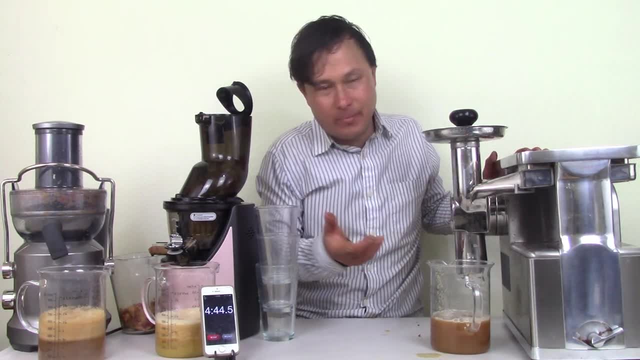 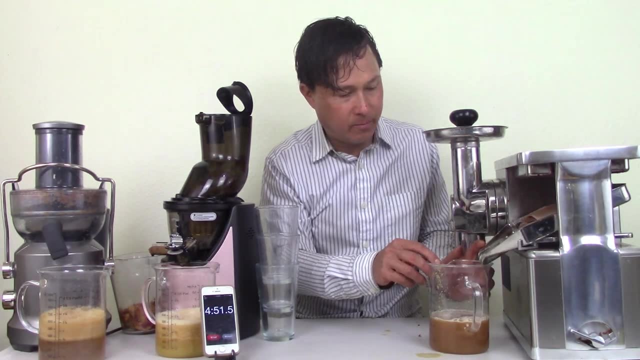 You can let it run basically another five minutes to get a few more drips. I don't think it's definitely worth it. The stream is broke. You're not going to get significantly more juice Once it comes down. I like to tip this up and then you know, wait for some of the juice. 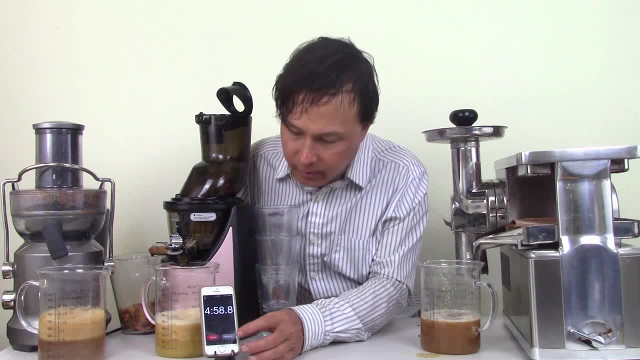 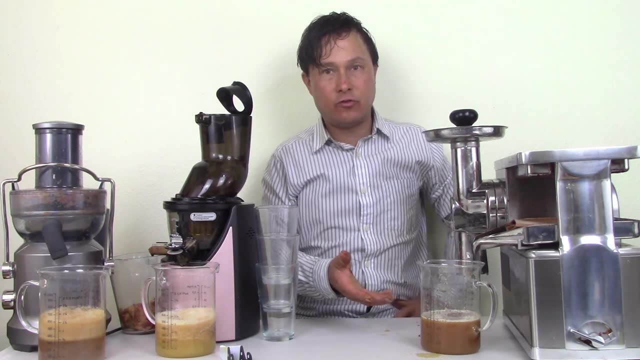 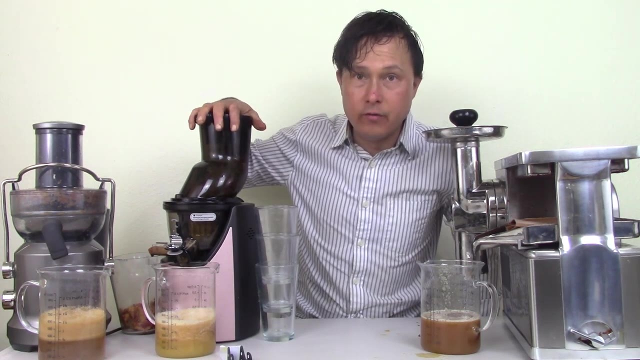 to drip out. Now let's go ahead and hit stop. Wow, look at that. That took nearly five minutes. so the pure juicer, to make this much juice, took, you know, twice as long- a little bit over, you know, 2.5 times as long- as the Kuvings did. and 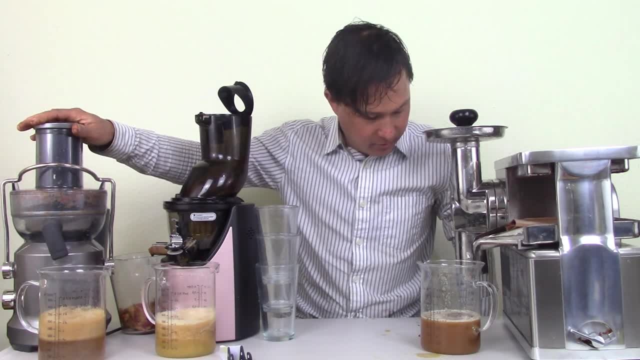 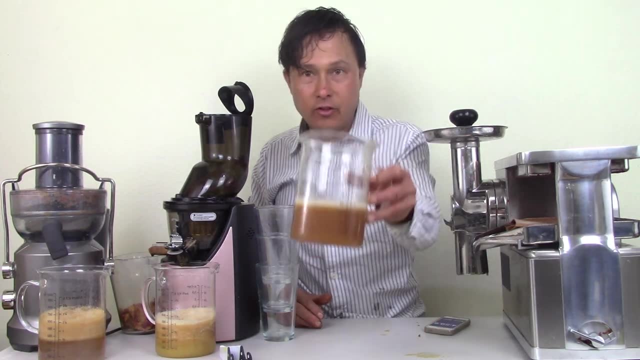 you know, still a lot longer. Was it five minutes? Five minutes versus 30 seconds, 10 times longer than the Breville. But let's take a look at what we got here. So look at this juice. As this juice immediately came out, it was a lot more brown. 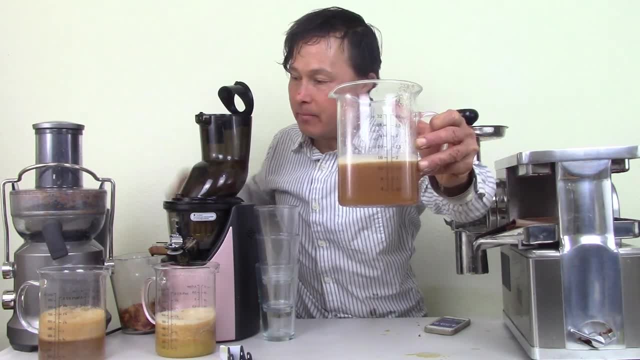 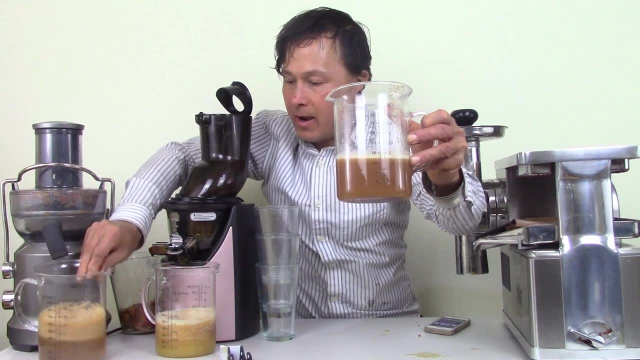 You know, browning is some oxidation that's occurring. You know, this juice wasn't that brown, but it turned pretty brown, but it's actually also very clear at the bottom, You know, whereas the Kuvings juice I showed you guys right when it came out, it was pretty. 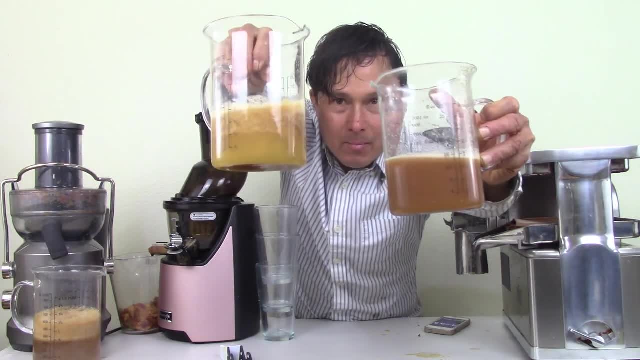 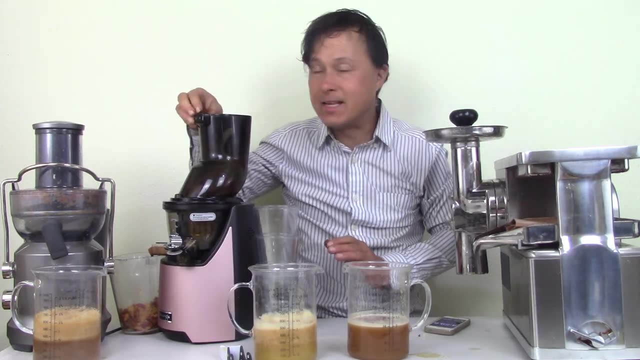 much looking nice And even now the bottom is still looking kind of nice, You know. so, comparing the oxidation, you know the slow juicer actually did the least oxidation. The oxidation is due to the, primarily due to the high-speed grinding. 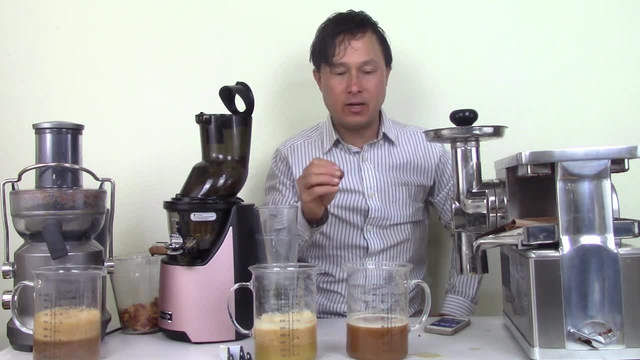 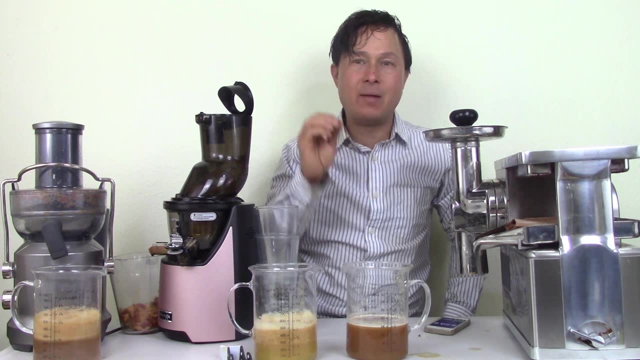 At the same time, you know it has been shown through published studies that the pure juicer will create more enzymatic activity in the juice, if enzymes are important to you. That being said, you know the enzymes in the juice are reacting with the antioxidants. 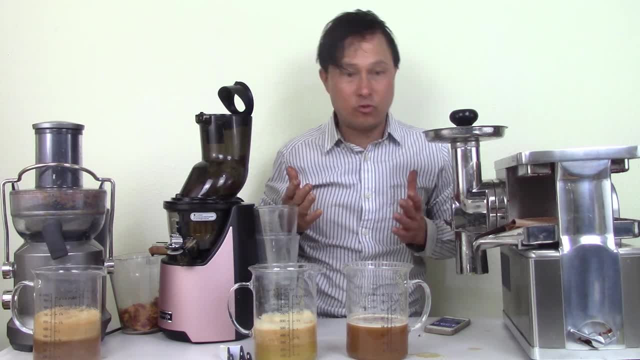 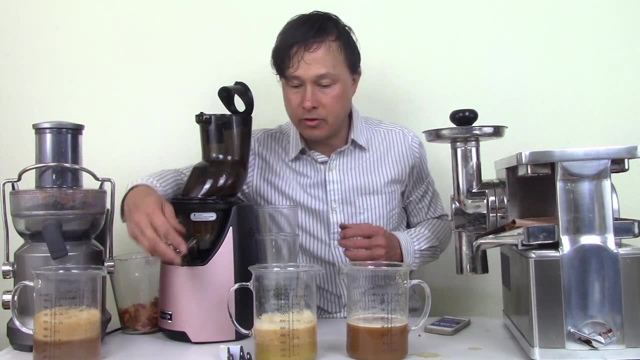 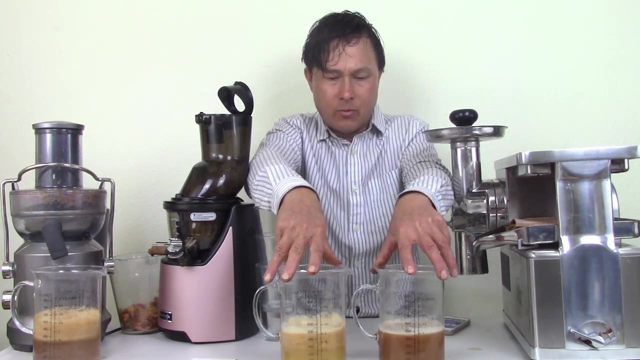 in my personal opinion- and lowering those at the same time. So you're going to trade off enzymes for some phytonutrients. To me, the phytonutrients are more important, all right. So, anyways, let's go ahead and put these up front and center for you guys, and we're 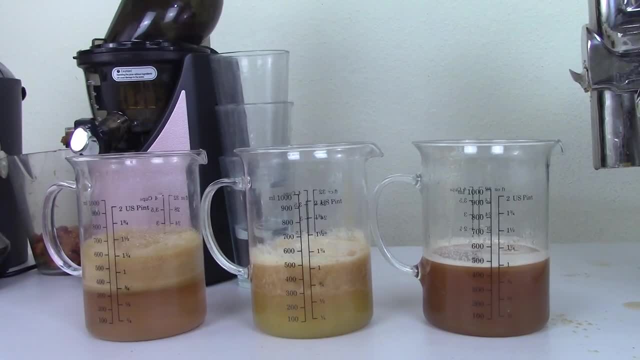 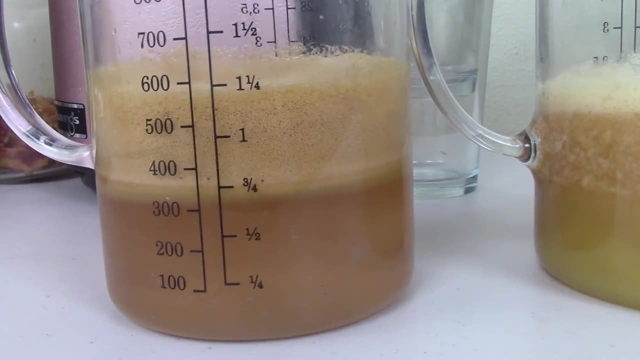 going to go ahead and do a close-up on the yields. All right, so here are the three juices. Let's go ahead and zoom in on each one. over on the Breville, It's fairly easy to see the yield on that one. 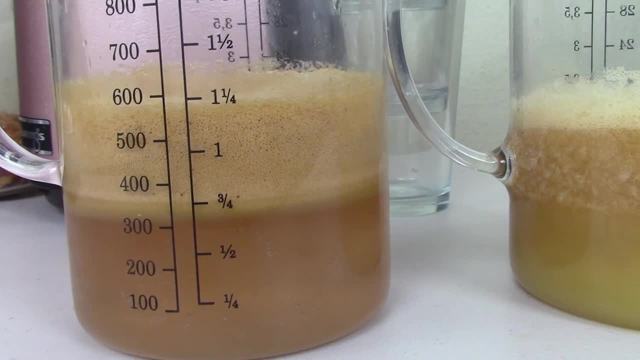 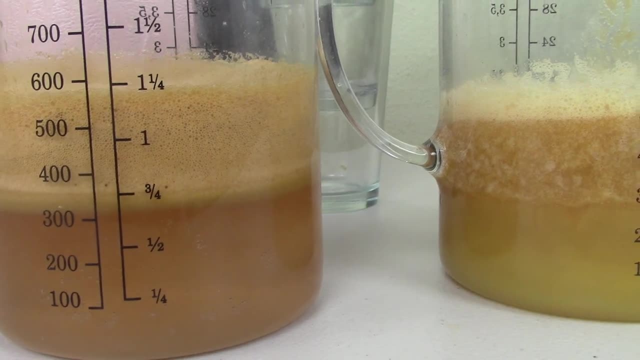 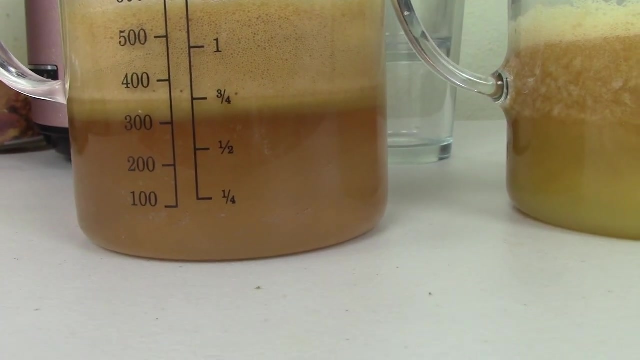 It's basically about a little bit over 300, you know, because I'm seeing like basically it starts getting into a foam layer. maybe 325, I don't know, maybe 350 at the absolute most, but then there's significant foam and also the browning that has occurred. 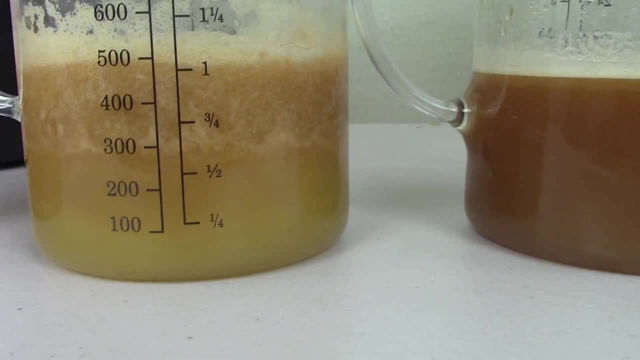 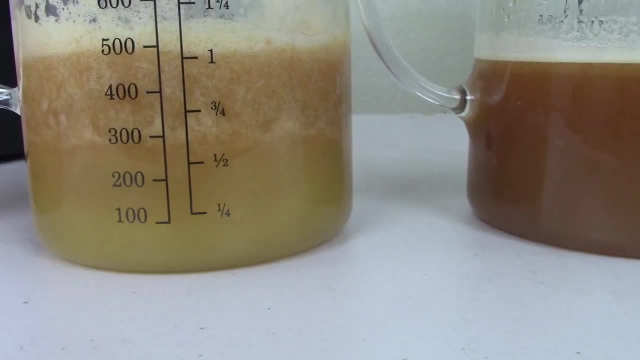 Over on the Kuvings. this is actually quite difficult to determine the overall yield. If you just look at the overall yield, it's 300, but I want you guys to pay attention to that. there are two distinct foam layers. There's the 300 layer, where you got more juice. 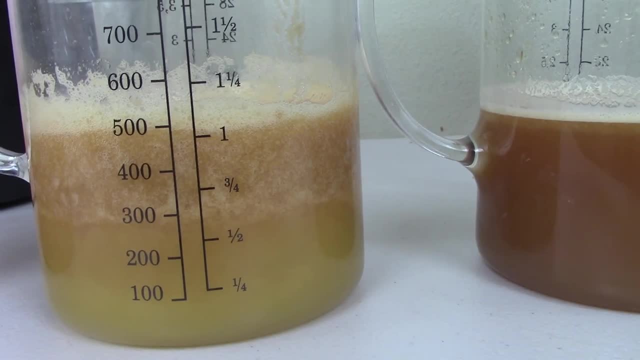 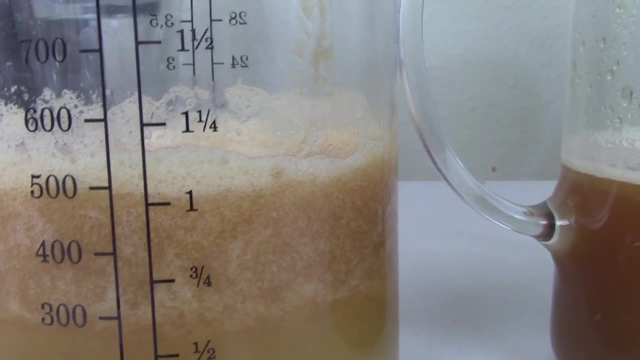 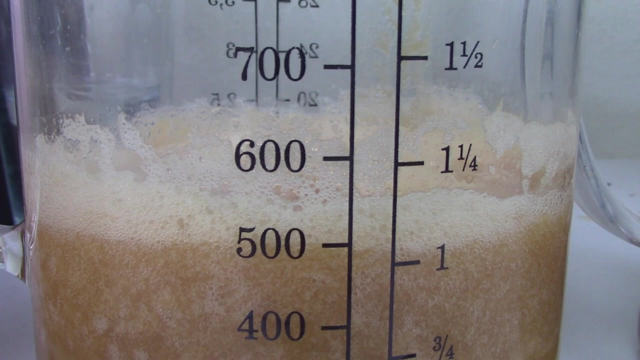 And then you have the… If you look to like 500, what you could see is the dark like foam stuff, right? So that's actually probably some fiber in there, so like some insoluble fiber. And then if we look above 500, then you know you clearly see the light foam layer. 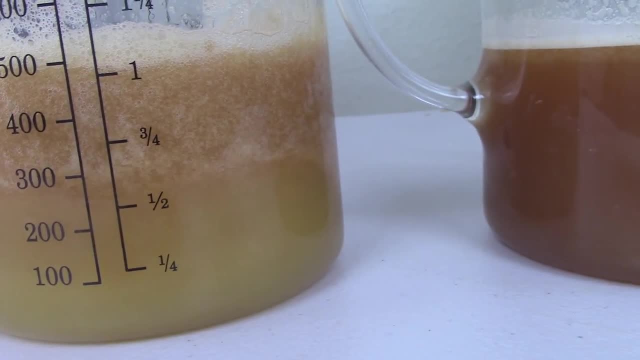 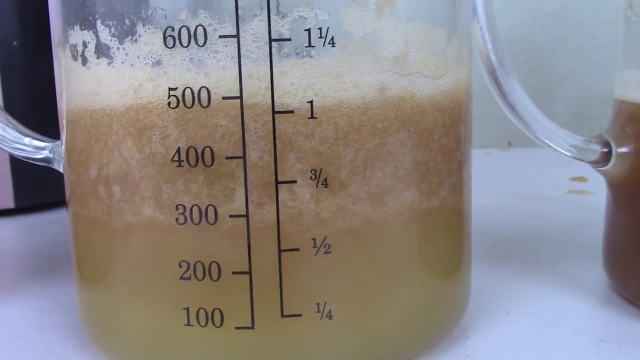 So I really…. It'd be difficult to call that one. Maybe if I stirred it up I could see more clearly the yield. but you know, I guess I'm going to say that it's… Okay, Maybe around 500 is the yield. 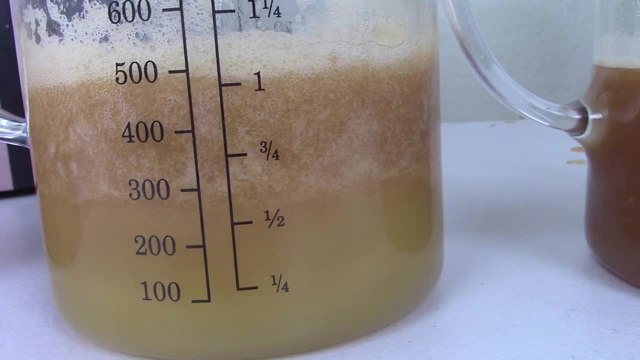 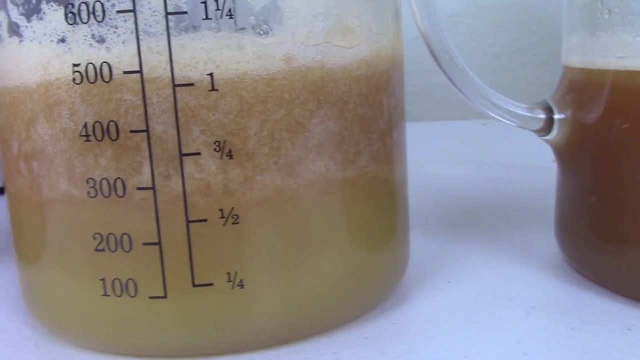 But the other thing that I'm also going to tell you is that this is actually a really thick, you know juice, kind of more like a… Not like a smoothie, but more like a nectar. It's more like a nectar juice. if you've ever had nectar juices, that are like kind. 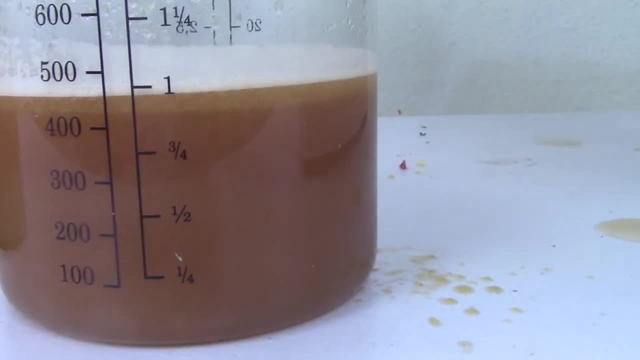 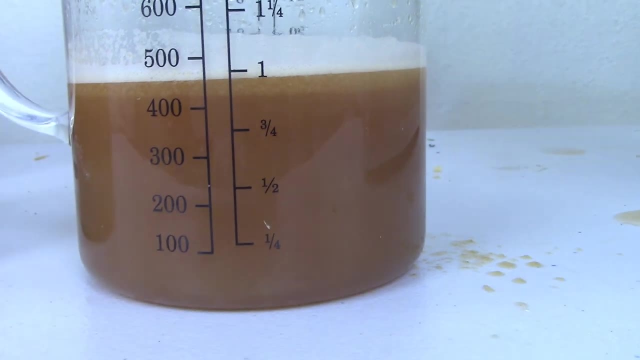 of thick and rich And then over on the Pure, Pure. no hassle, no screwing around. That's, like you know, about 460 milliliters and that is straight juice. But I want you guys to look at the color. 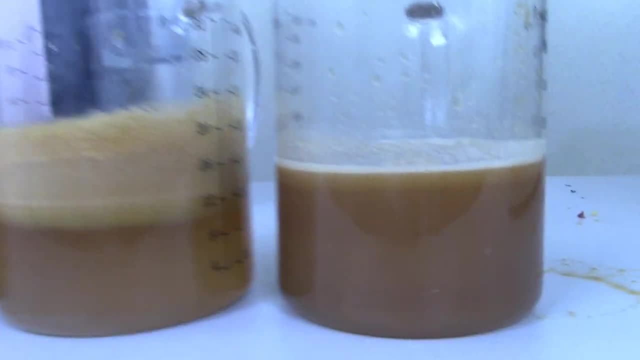 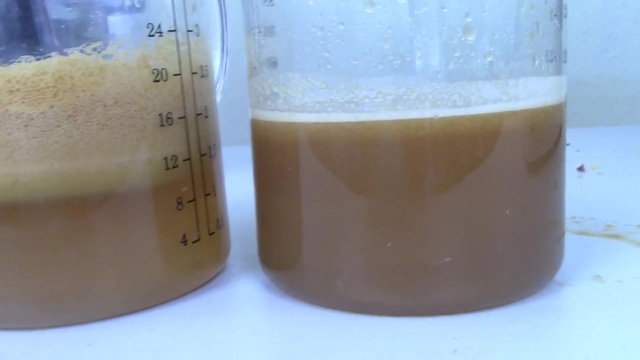 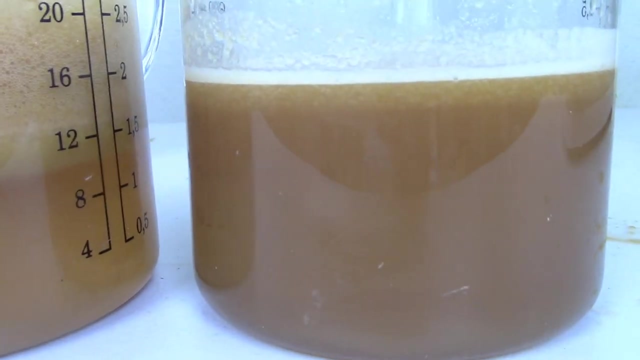 In terms of least to most. So the most color, you know, the most browning happened in the Pure. you know, My opinion is because of the enzymes. There's more enzymes and more oxidation that's happening in the grinding process. So, yeah, that's really dark. 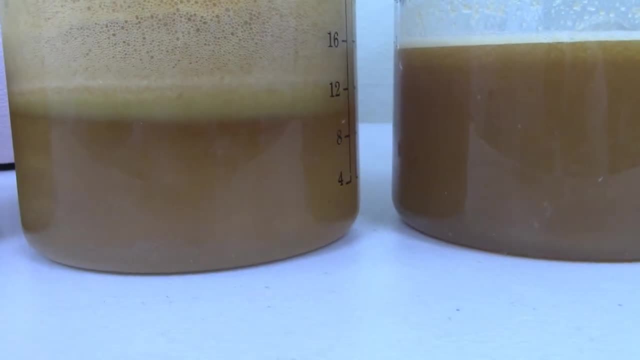 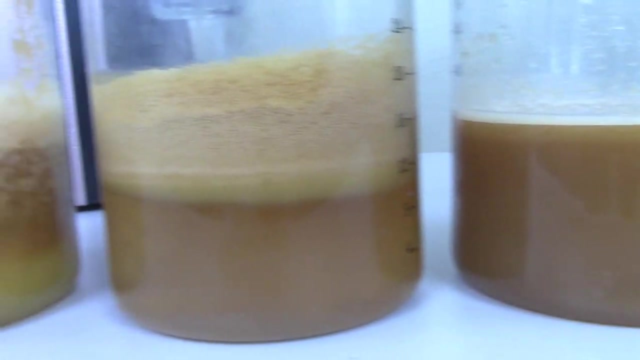 And then if we go over to the Breville, you know, yes, there's some oxidation in there as well, but it's, you know, a tad bit lighter than the Pure. And also we did the Pure juice last Meanwhile. 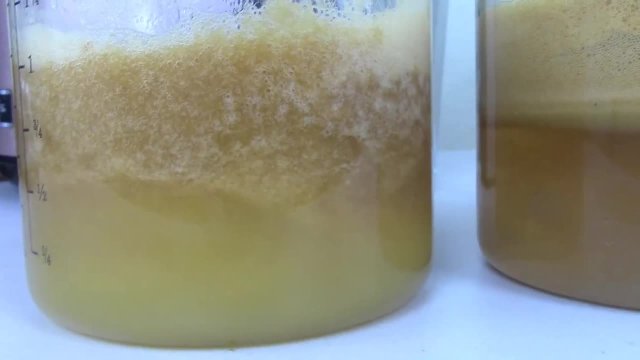 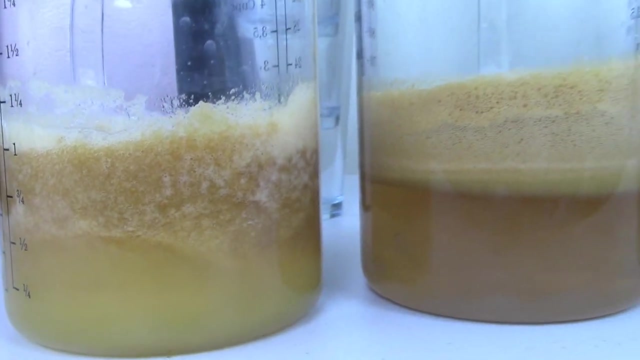 If we go over on the Kuvings. you know that's definitely darker, you know, than it was when it came out, But it's still significantly lighter than the others, You know. I believe this to be due to less oxidation, due to the slow juicing process. 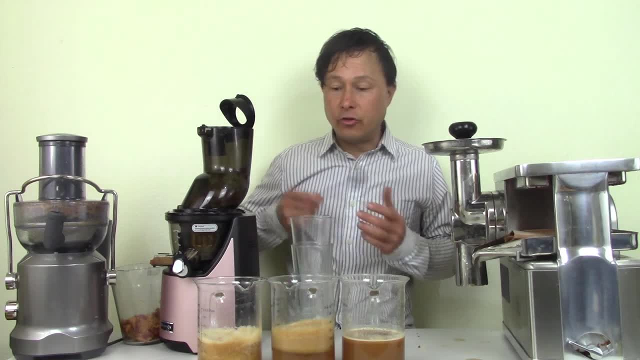 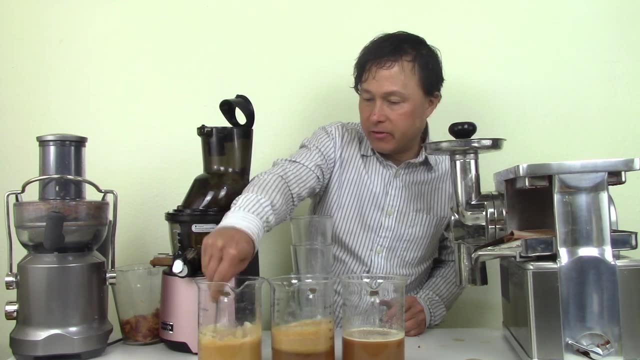 All right. So you guys got to clearly see a close up on the juices. What I want to do now is I'm going to stir these juices up, So maybe we'll start by stirring the slow juice up first. You know, I'm feeling definitely some resistance. 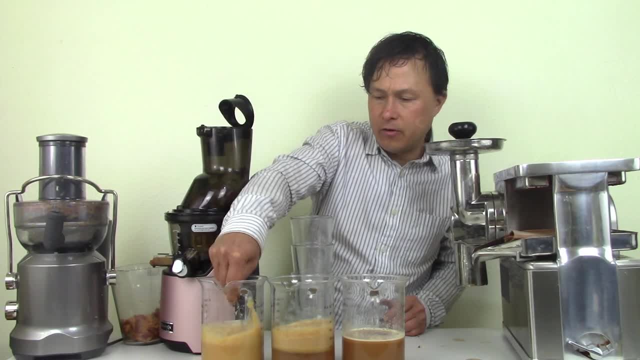 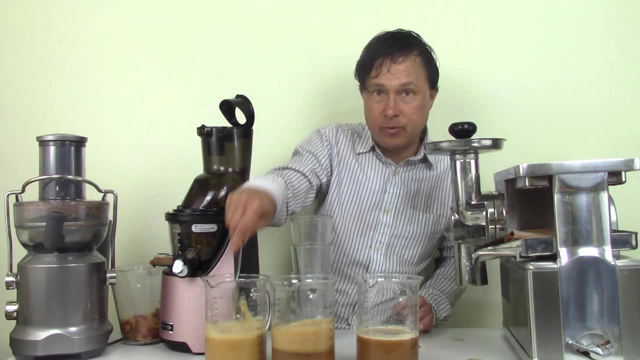 It's definitely thick, More like a nectar. for sure, Yeah, For sure, Versus a thin juice. If you want the thinnest juice, of course that's the Pure. This is going to be the thickest juice, but also it will contain more fiber in there. 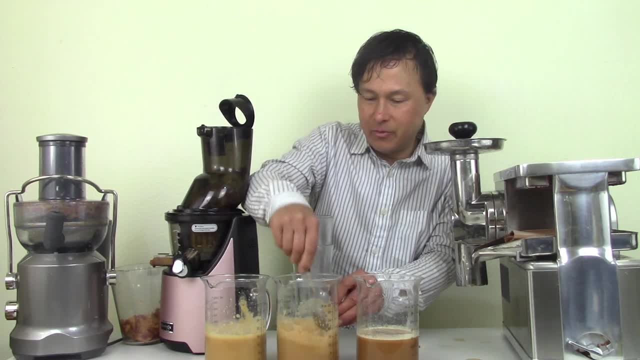 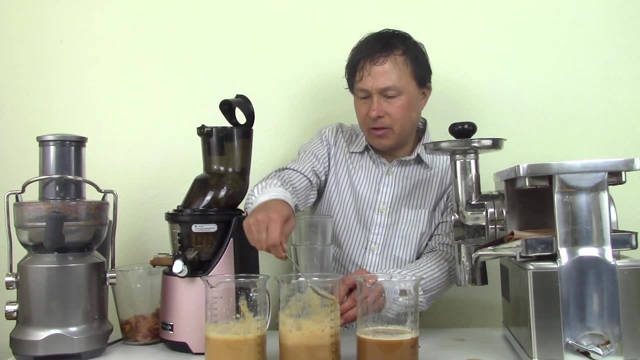 We're going to go ahead and stir the Breville juice up and stir those bubbles into there, which I normally don't like to do, And there's lots of foam still happening in there And you know, this is kind of- oh, there's like kind of like, there's like big chunks. 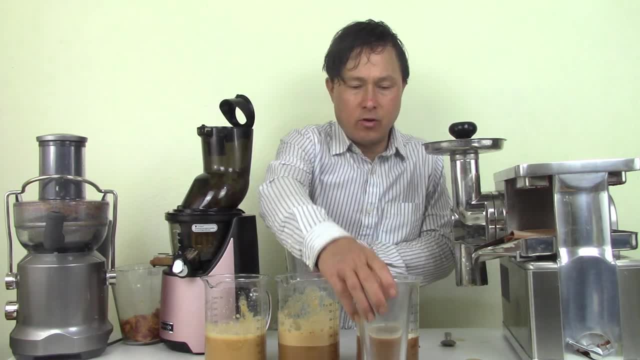 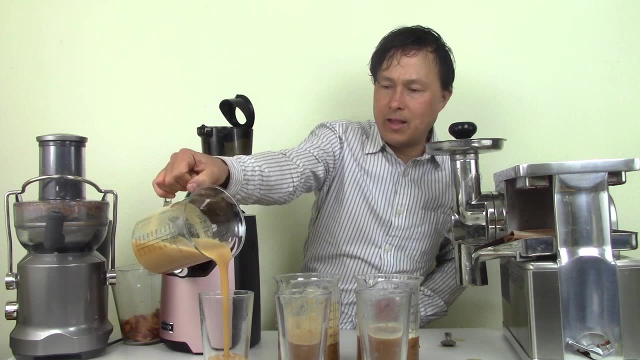 and whatnot in here. So then we're going to go ahead after stirring, we're going to go ahead and pour it out into three glasses So we could see the texture, The texture difference. So that's really like a nectar, right? 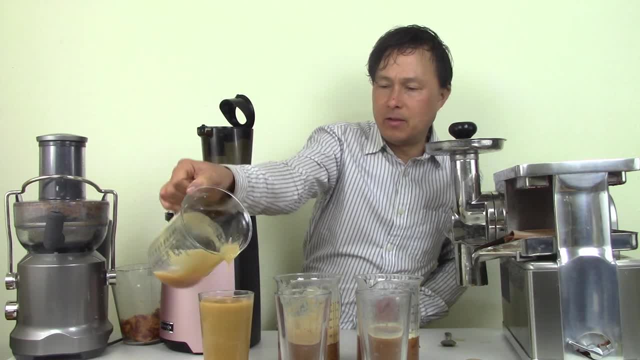 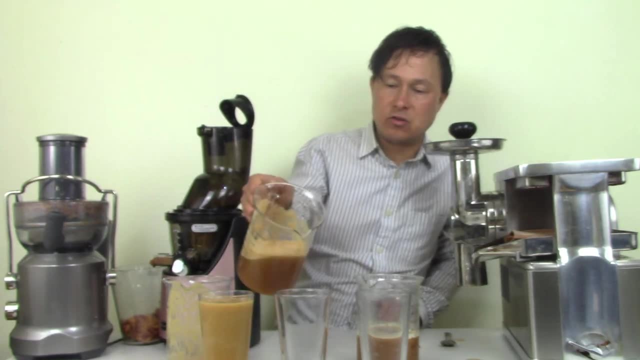 If we used a harder, firmer apples, you know it'd be a bit less, But you know this is what the slow juicers do. They will give you more fiber. you know, in the juice the sible as well as the in sible. 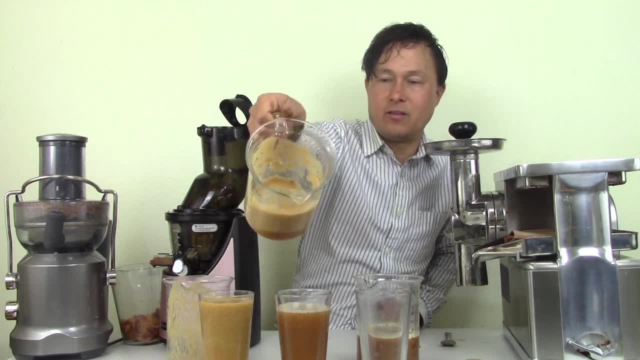 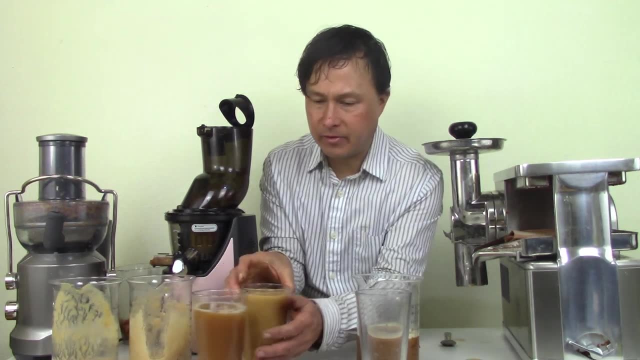 Here's the Breville juice. Luckily, as I'm pouring it, a lot of the particulate, the thick, you know frost stuff is staying in the jar. Okay, So for practical purposes, let's go ahead and put these in the right order. 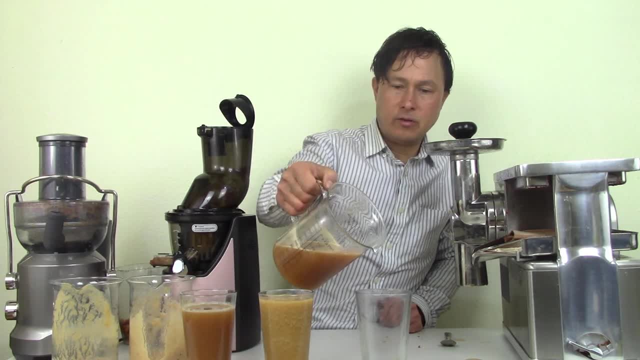 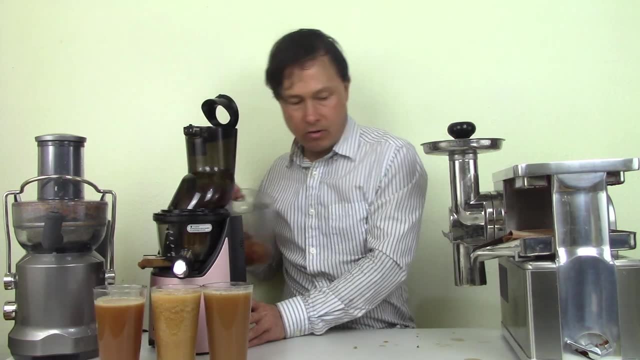 And then over here is the pure juice, you know, and let's go ahead and pour this out. Now, what I want to do is I want to share with you guys, actually, what the pulp looks like that came out of each of the juicers. 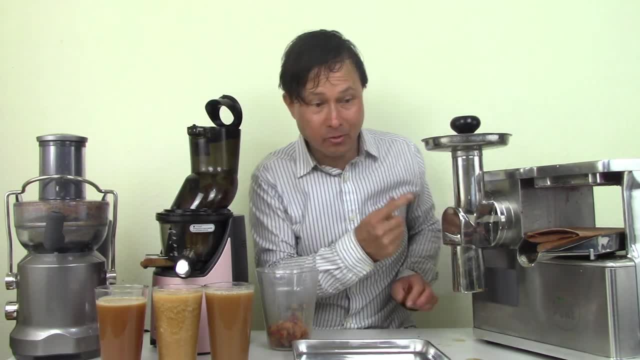 So we have a little tray here and I want to say that the pure juicer was absolutely the messiest. You know. while juicing it did splatter a few things everywhere. The other juicer: it did splatter a few things everywhere. 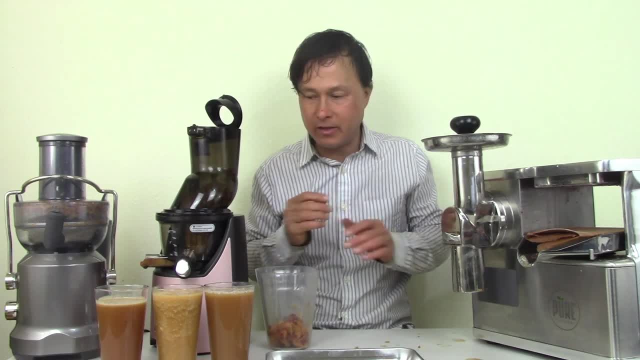 The other juicer: it did splatter a few things everywhere. The other juicer: it did splatter a few things. The other juicers were much, much cleaner, especially the Kuvings with a little flap, so they don't get the drips. 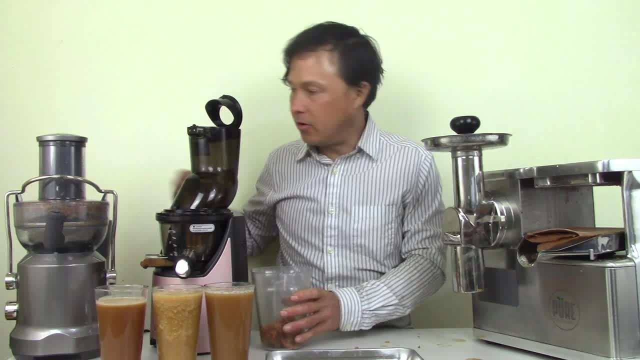 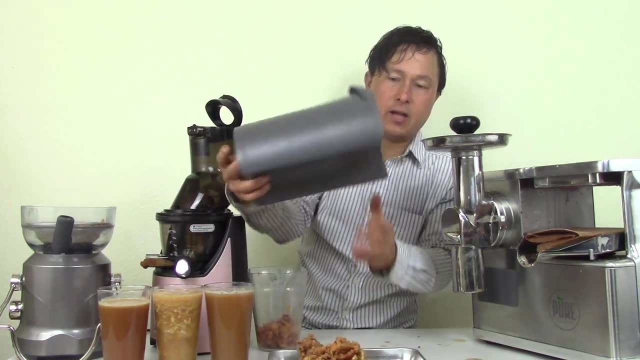 But I want to show you guys the pulp, so maybe we'll start over on the Breville pulp first. So taking the Breville pulp out, putting it on this little tray right here, there's lots of pulp that came out of the Breville. 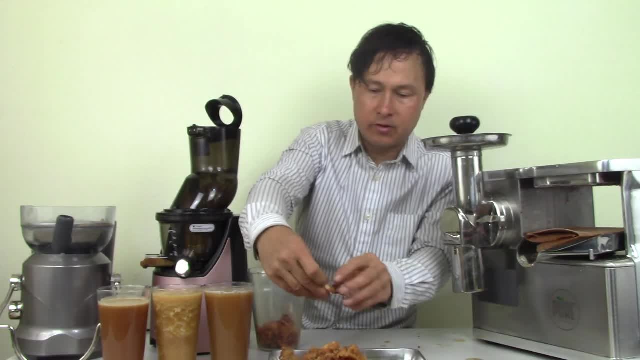 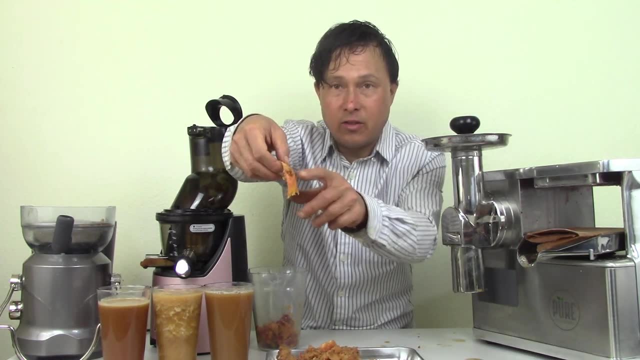 Okay, And what we're going to see in the pulp is that we will see literally chunks of apples that did not get juiced. I mean, here's the whole. you know skins, And this is one of the tests they've done in the science. 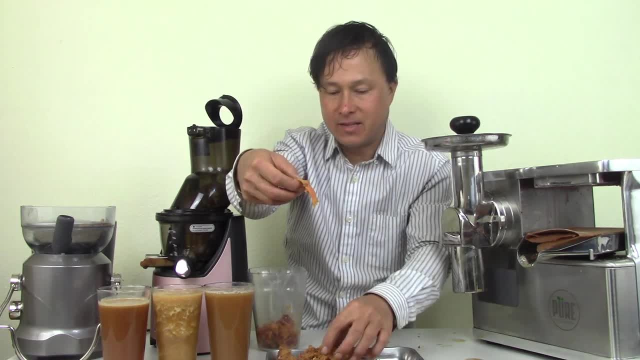 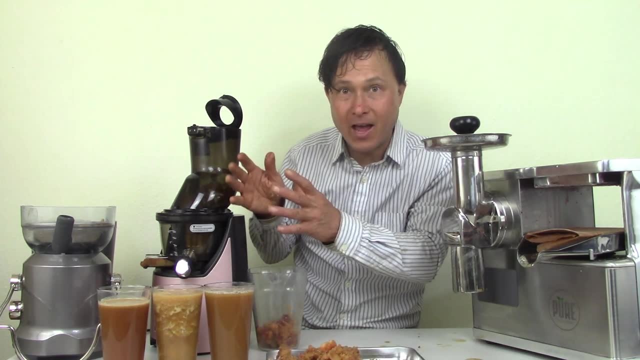 science that the high speed juicers don't grind up the seeds effectively or the skins, so you get less polyphenols in your juice. So you've got to ask yourself: is it worth doing it fast so I can have juice versus not doing it? but you're going to miss some of the different polyphenols, and those are the. 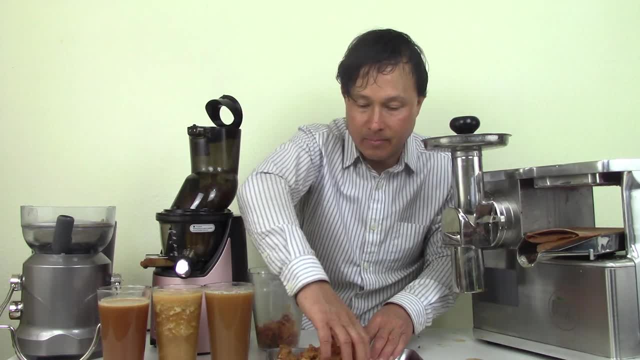 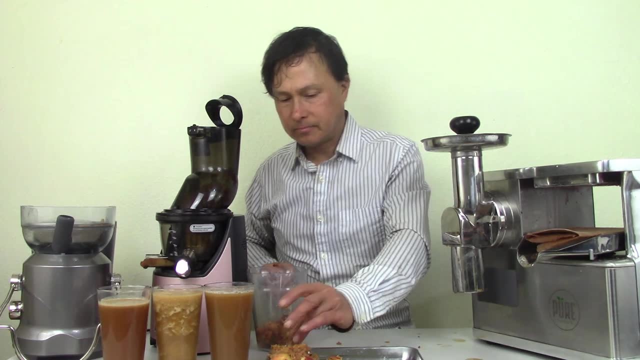 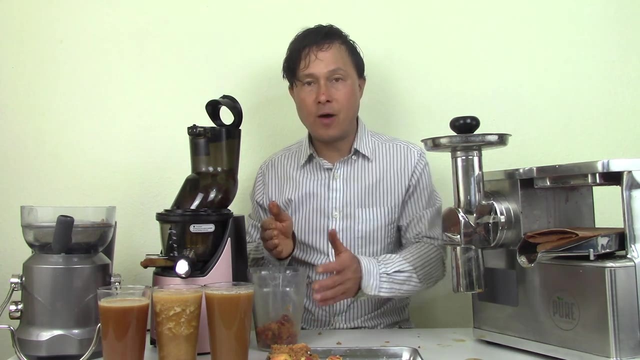 healing compounds and juices. in my personal opinion, Meanwhile there's also lots of pulp here. the volume is so much because it also is quite wet still and if we press that out, like if we put that in the pure, we could surely press out more out of that pulp and it will compact the pulp a lot. 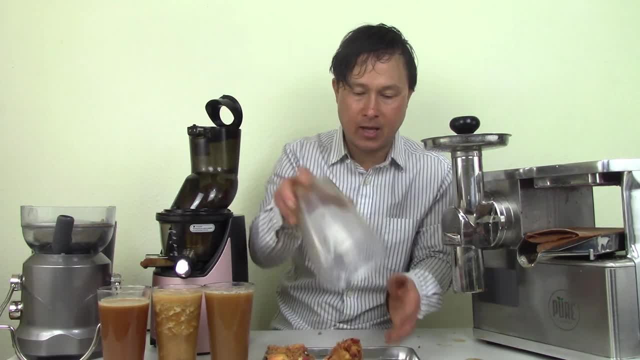 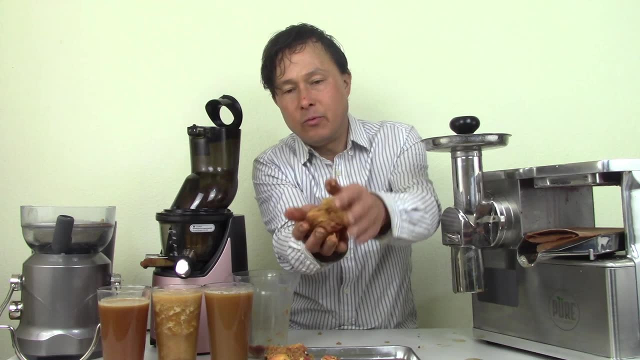 Meanwhile on the Kuvings there's some still pulp left in the machine. but the pulp that came out of the machine is a lot more small, it's a lot more compact, it's a lot more ground up. you know there's no big chunks in here it's. you know, it's pretty ground up pretty. 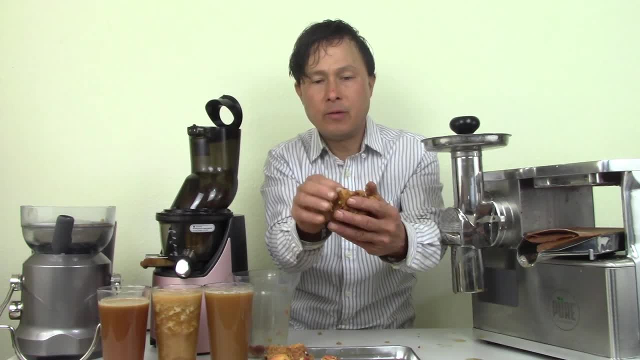 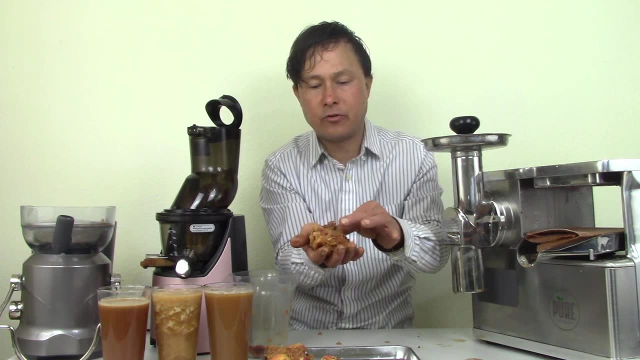 well, I see a seed that actually went through their hole. you know, depending on the slow juicer, Some slow juicers better grind seeds up than others. the Kuvings has more of a coarse grind, in my personal opinion. alright, yeah, I'm seeing a few, you know, large pieces of skin that just 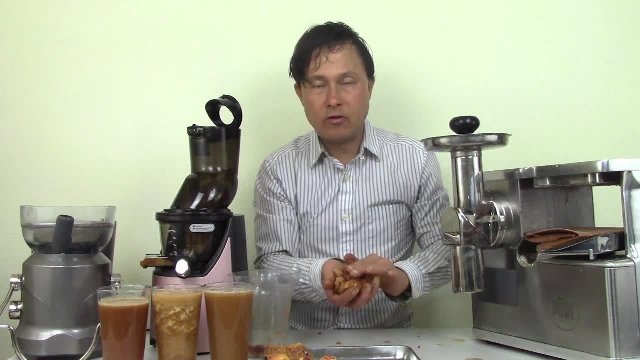 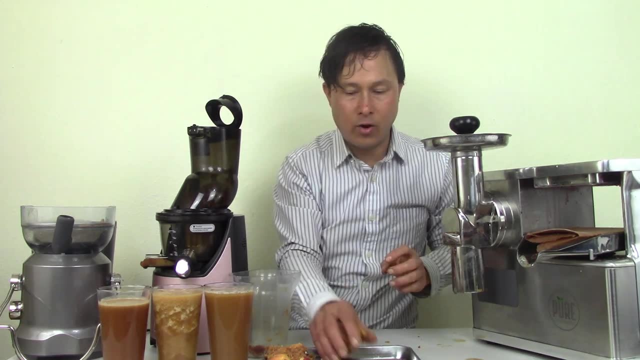 kind of just went through the Kuvings. you know, if you get a juicer that grinds better, it's going to extract more nutrients out of those skins and seeds that are quite beneficial for us. alright, Here's a little bit more pulp from the Kuvings. 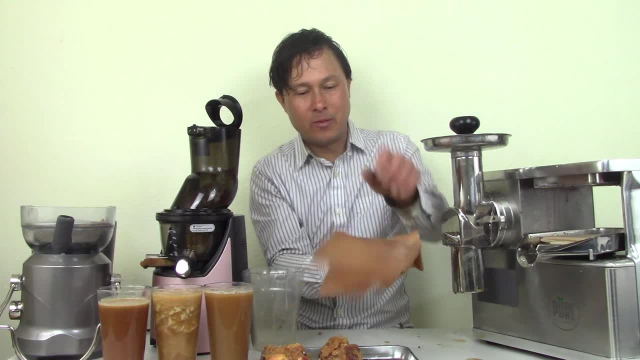 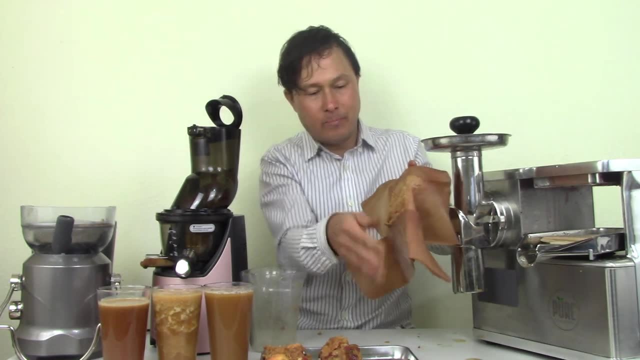 Finally, let's check the pulp on the pure. This always amazes me, the pulp in the pure, you know. so basically, we're going to open this press cloth and the press cloth, you guys can see the pulp and it's kind of hard. it's stuck on there. so you got to clean this when you're done. and you know, I'd rather actually 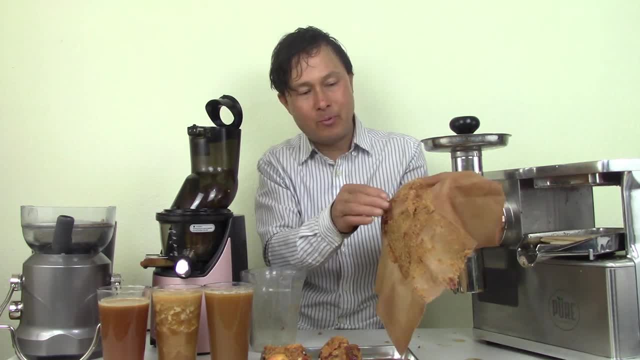 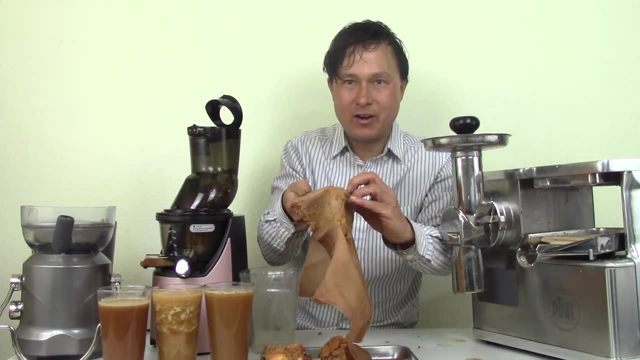 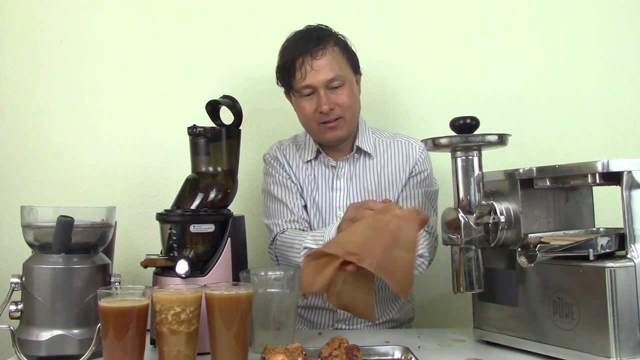 clean a juicing screen personally than apples on this press cloth, because it's literally just ground in. it's like you got kids, they, you know they- get a grass burn. this is like ground in. It's like kind of not just ground in, It's not separating quite easily and yeah anyways. so I got to use my nails to scrape. 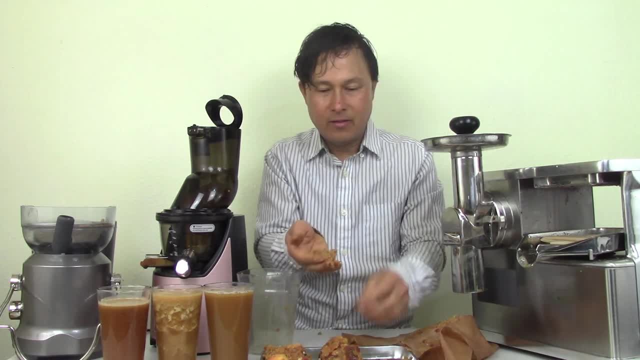 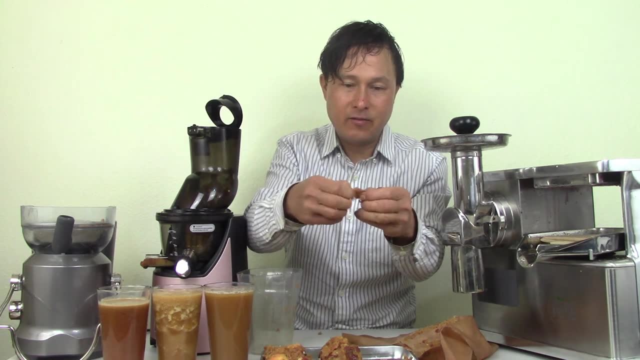 this stuff off. but if we look at this, you know I mean this pulp is a is drier than all the other ones. you know there are some, still some pieces of a, of skin that actually didn't completely get ground up and, I'm sure, over. and you know we got another, another press. 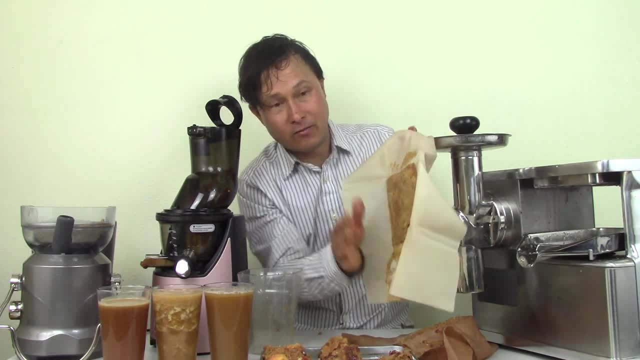 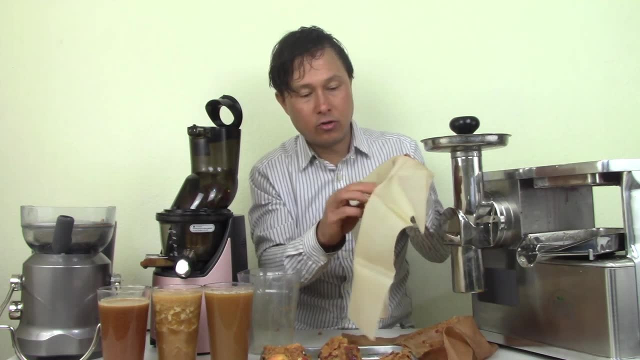 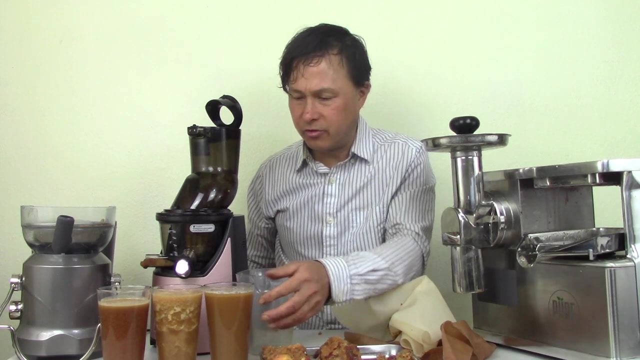 cloth full of the pulp here. I mean, this pulp is impressive. it is super dry. so if you want the most yield, Yeah, Hands down. the pure is the juicer to go with for sure. okay, so I want to talk about now. you know, all the juices have pretty much oxidized, similar since I've actually mixed them up. 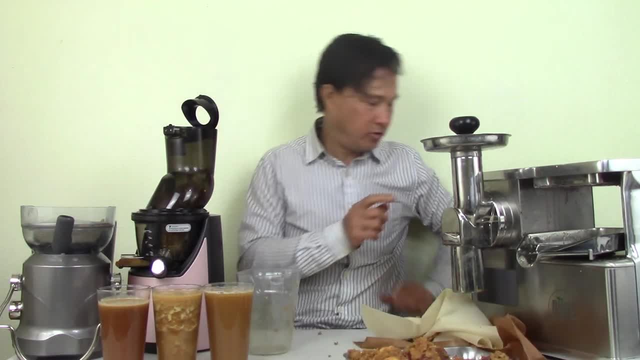 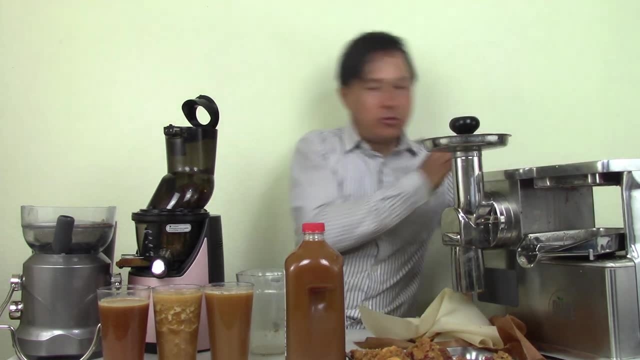 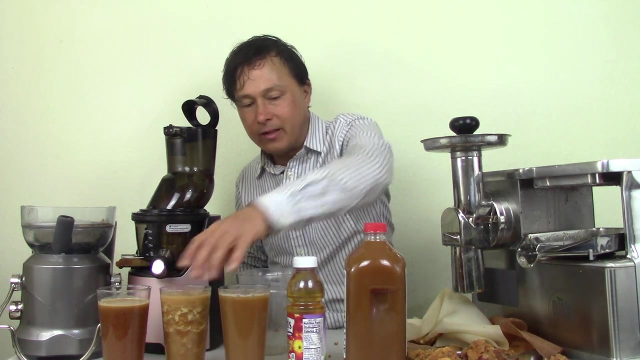 I want to go ahead and bring out the commercial juices, including that, you know, the HPP juice that's cold-pressed, and the Welch's juice. that's completely clear. so you know, none of the juices that we made- They're stirring up, you know- are completely clear like this, you know. so they all contain. 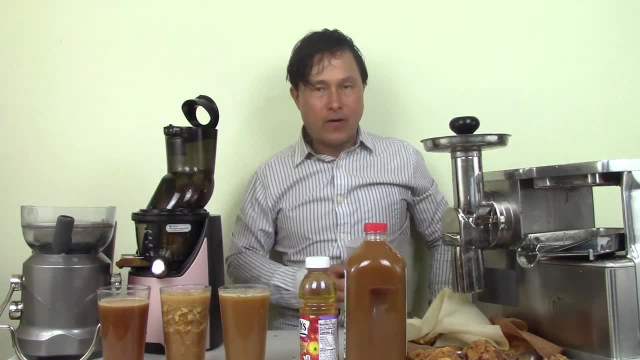 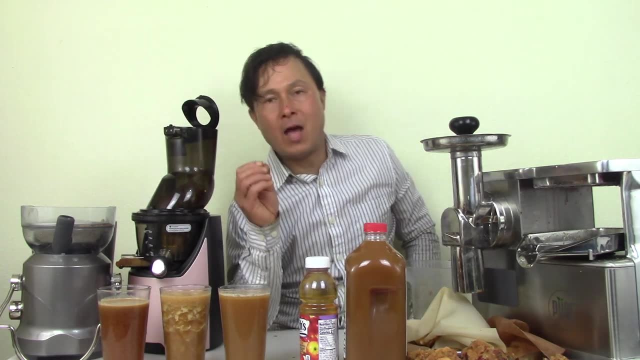 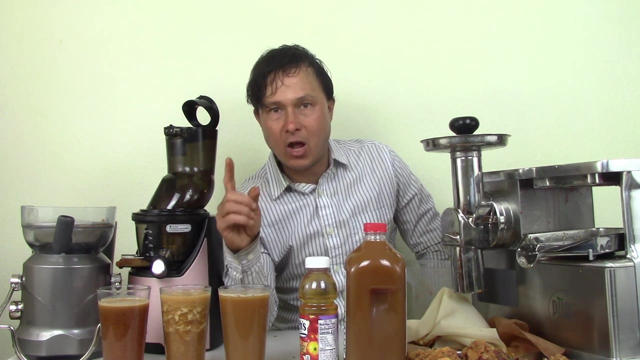 some levels of soluble fiber, although the soluble fiber levels are different in each juice that was created, and the whole point of this video is how much soluble fiber, which is this fiber that dissolves in water, is going into each juice. because a soluble fiber matters. that you know if you watch my last episode. I made a site. I looked into the science of 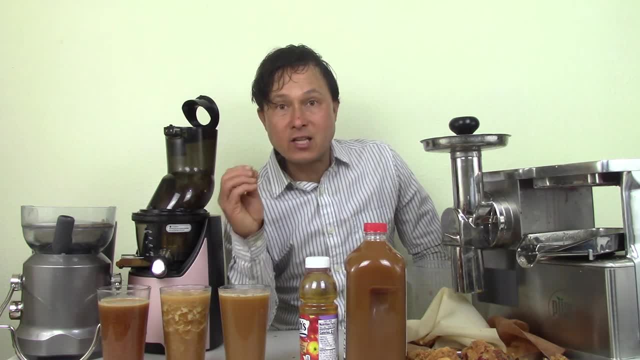 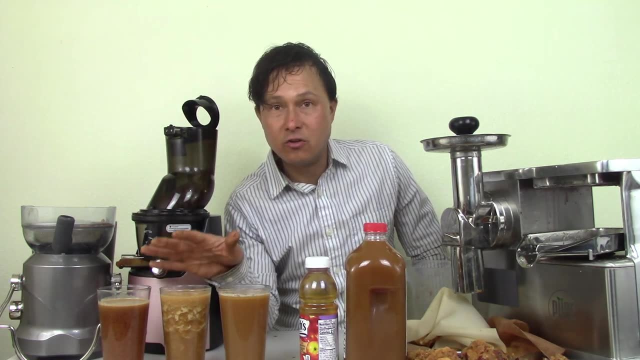 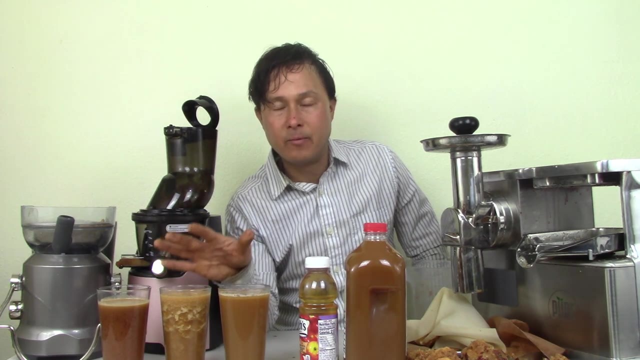 the soluble fiber And, according to science, juice has soluble fiber. so when people exclaim juice has no fiber, well it depends on how the juice was made. home juiced juice depends how the juice was made. juices that are made at home will always have some soluble fiber and, in my opinion, 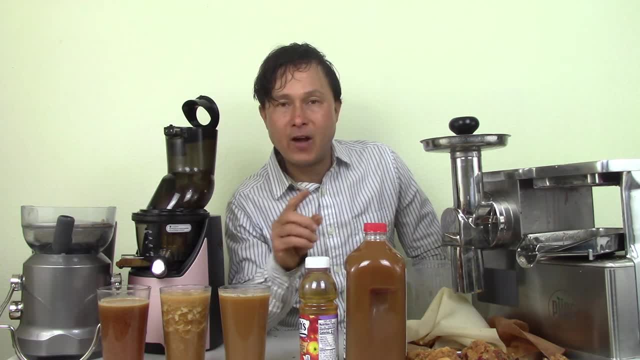 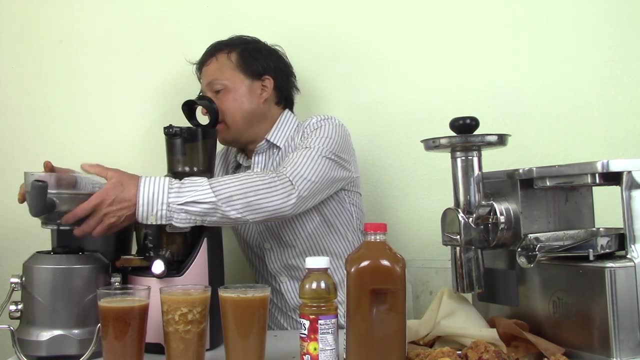 the more filtration you do, the more soluble fiber that can be removed. So, for example, on the Breville, on the Breville, here you know, the filtration that's happening is a hundred percent due to the soluble fiber. Yeah, It's a hundred percent due to the juicing screen here. this juicing screen has very small. 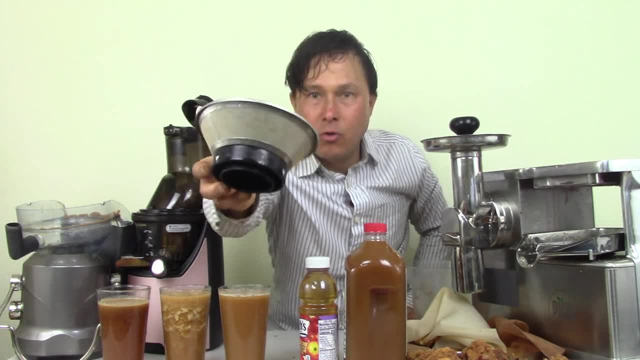 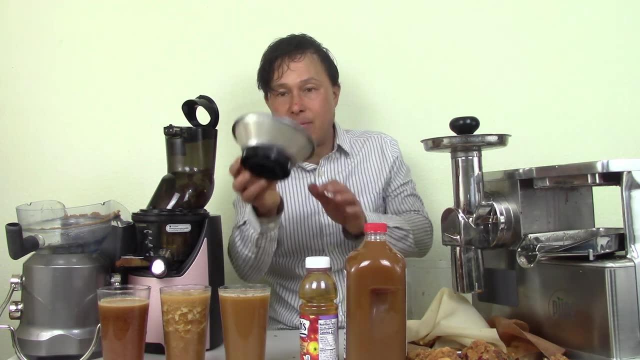 holes I can kind of see through there, but they're micro fine holes. so this will leave a lot of the fiber behind the in soluble and let not- maybe not as much soluble fiber through. you know, even even after that we got the covings. let's go ahead and take this apart. I want 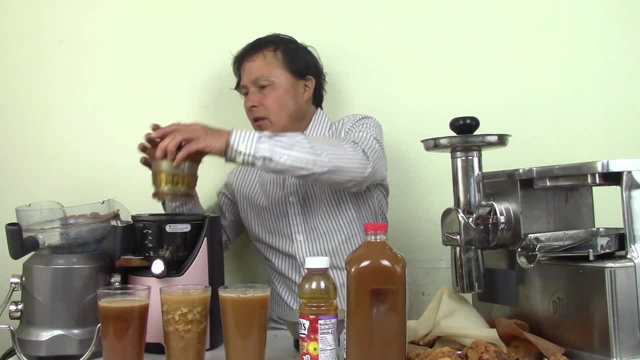 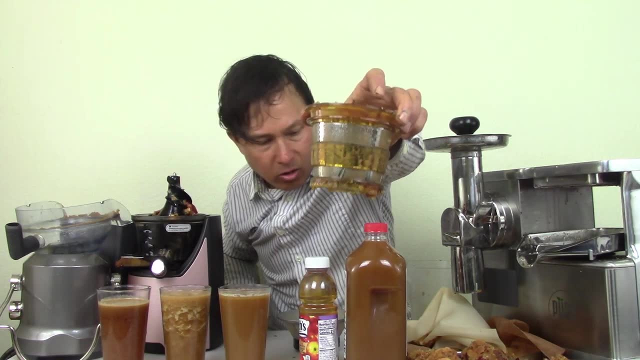 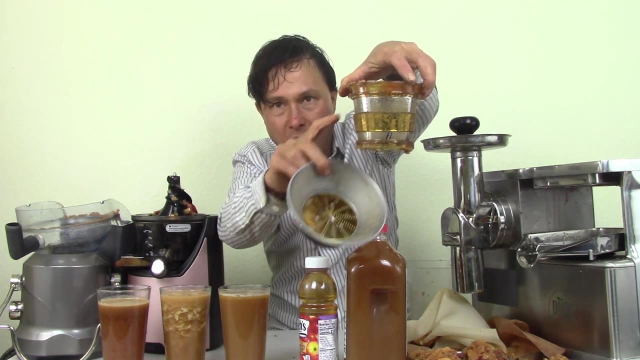 to show you guys this juicing screen. this juicing screen also has holes in it, but the holes in it are a lot larger than the holes in the Breville. you know, some juicers even come with coarse screens with even larger holes, if you want to keep more of the fiber. 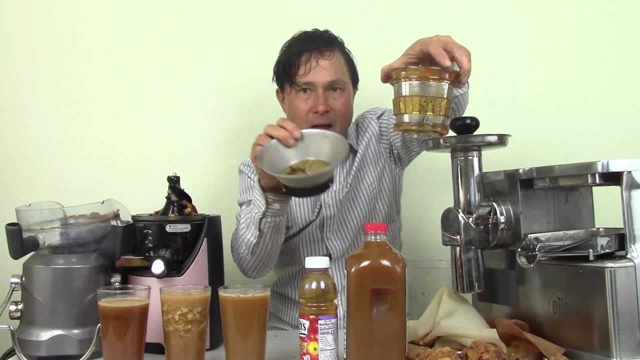 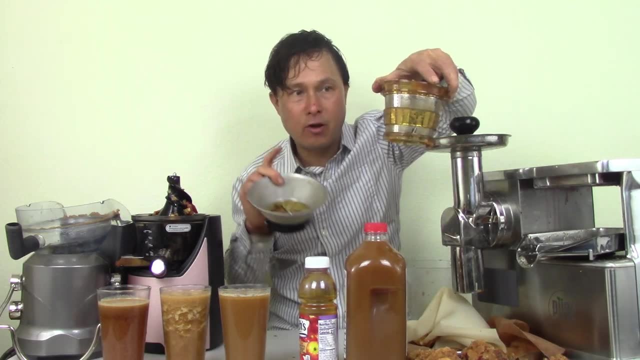 in there. you know, mostly it's keeping the in soluble fiber, but also, in my personal opinion, it'll let more soluble fiber through because the holes are bigger and more importantly, and also my personal opinion, it'll let more- you know- phytonutrients, polyphenols, through. 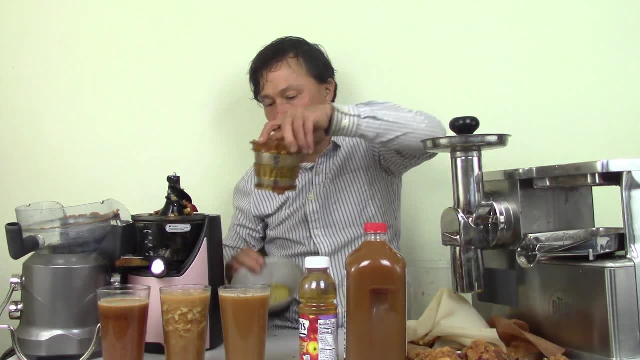 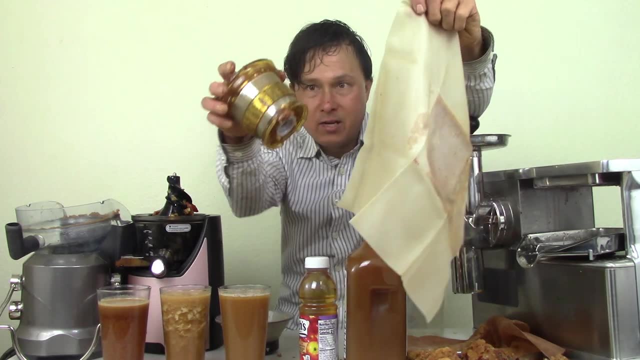 because of the larger pore size. Yeah, Yeah, Yeah, Yeah, Yeah, Yeah, Yeah, It's very important. right to discuss, Finally, the pure juicer. you know, when you have to go through the pure juicer, you're not even going through a screen, so the screen holes. once again, covings has the largest holes. 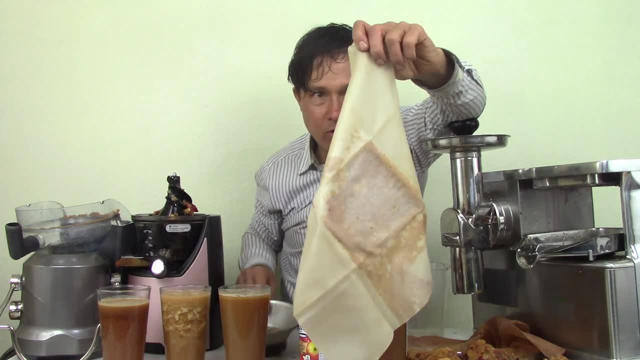 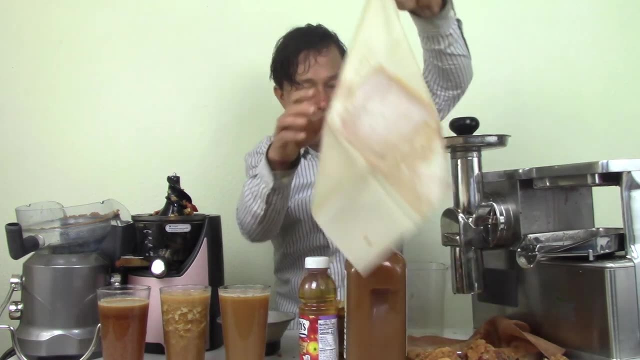 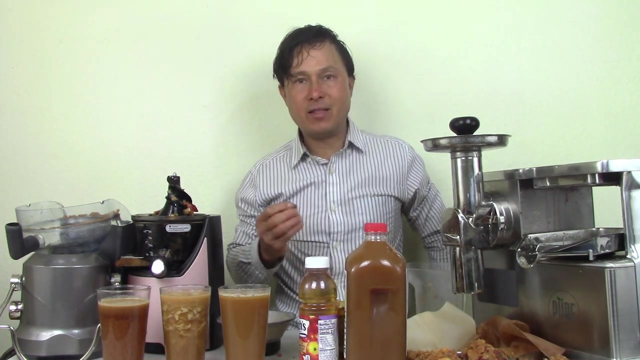 the Breville has the smallest holes and the pure doesn't even have holes. you're going through a nylon press cloth that has a much smaller pore size, so you're going to hold back, like virtually all the in soluble fiber and, in my personal opinion, keep less of the. 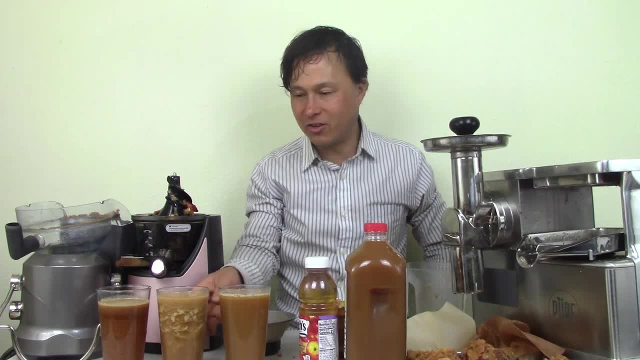 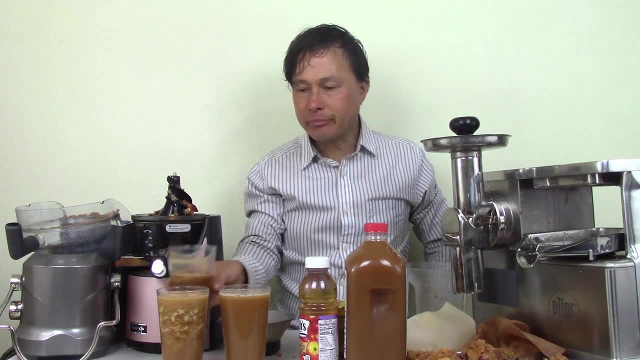 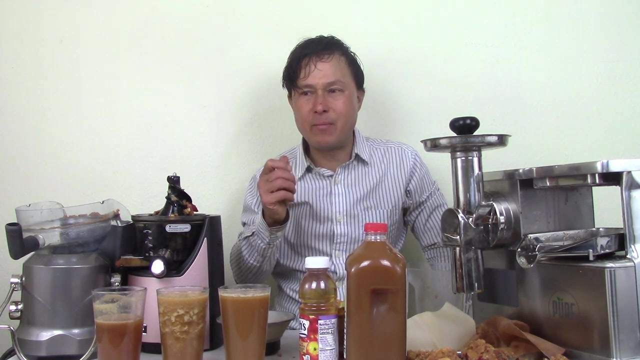 soluble fiber. So how does this equate when we taste the juices? So let's go ahead and taste the Breville juice first. That's a pretty smooth juice. I feel a little bit of fiber particulate in there, not much. 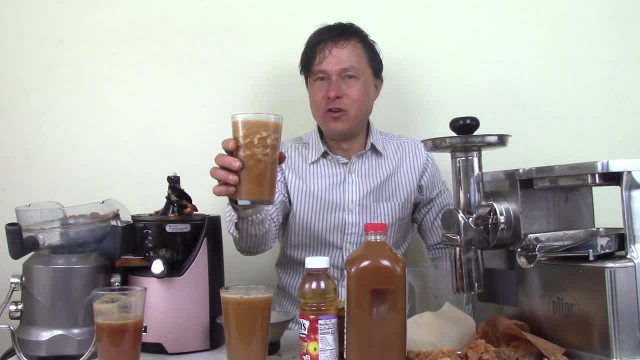 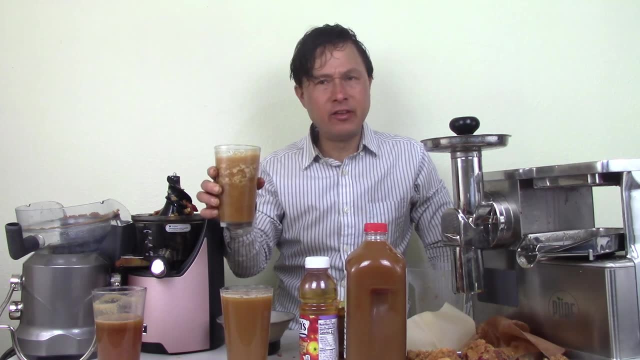 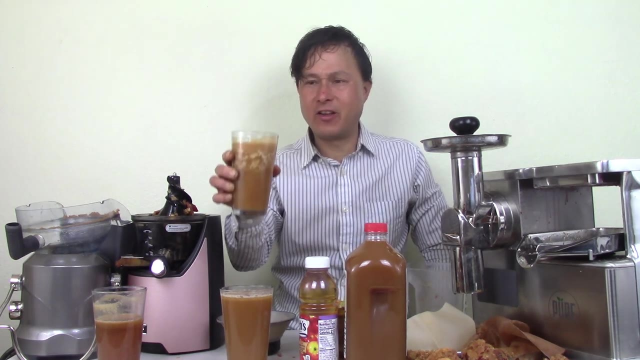 Tastes pretty oxidized. We're going to go ahead and try the Kuvings juice. This is thick guys. I mean, this is definitely, you know, a nectar- nectar of the gods- not a juice. So don't expect slow juicers to make really good fruit juices. 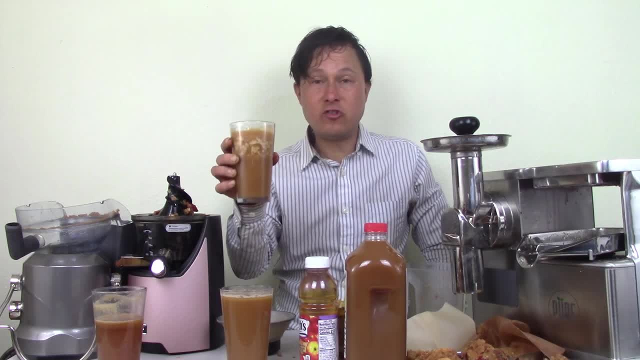 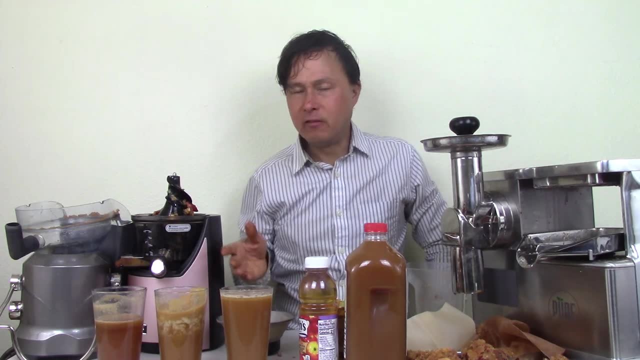 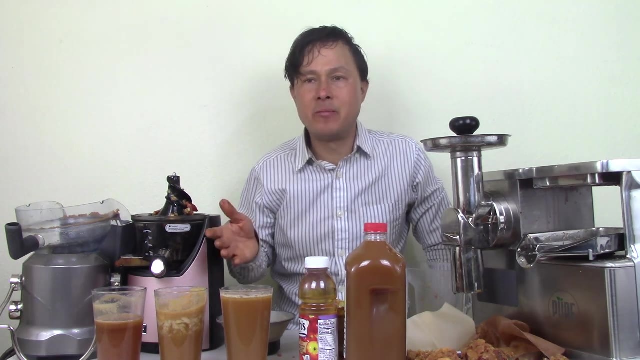 It will give you guys more fiber in there, which, in my opinion, can be of a great benefit. Okay, The way to reduce that is to juice it with other items that'll give the juice more liquid content. So, for example, jicama and apples or carrot and apples, and juice a lot of carrots with. 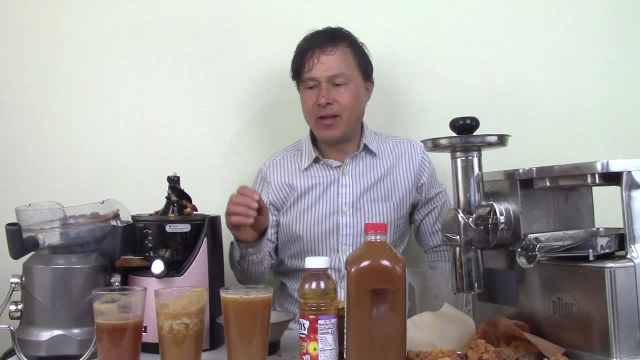 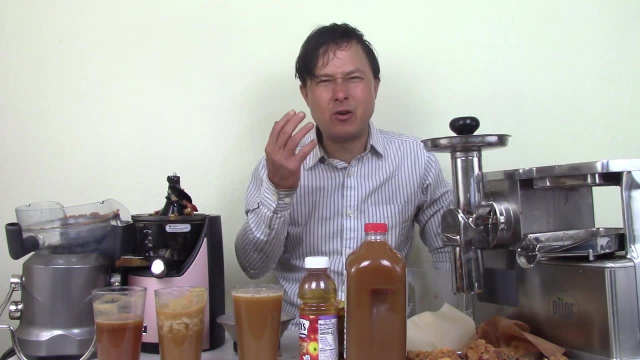 a few of those softer apples and it'll kind of blend in a lot nicer than making it super thick. Finally, we're going to go ahead and taste test—oh and that—actually this juice tasted better. I didn't have like the bitter overtones. 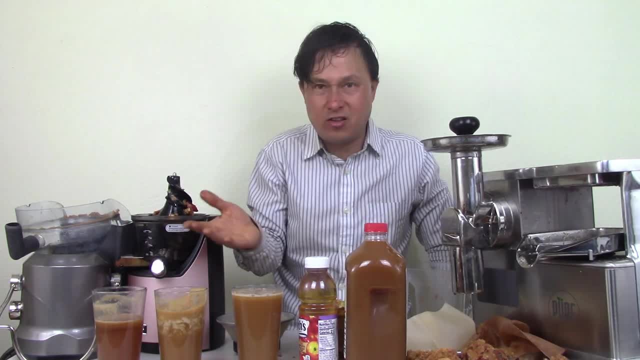 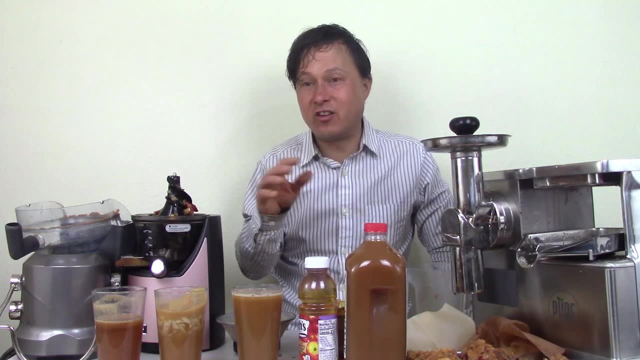 With the Breville juice, I had kind of like bitter overtones. This actually just kind of tasted like a thick, kind of like, you know, nectar slash smoothie. Not quite a smoothie, because it's not that thick, because smoothie keeps 100% of fiber. 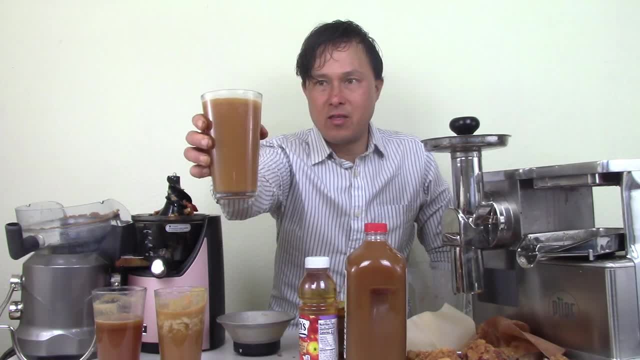 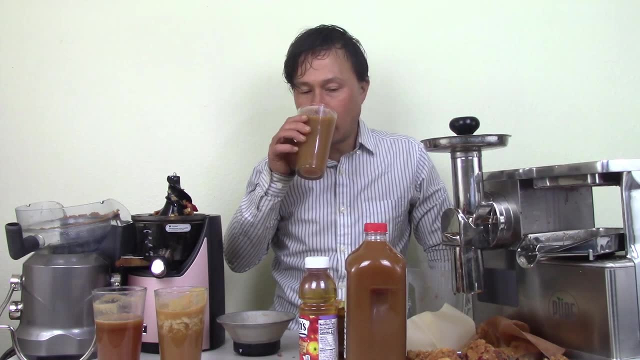 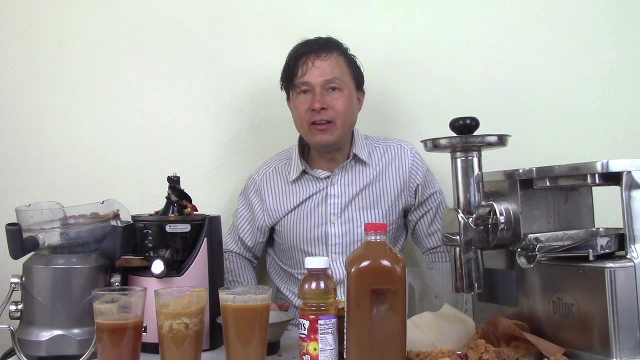 We did remove some of the fiber. Finally, we're going to go ahead and try the Breville—finally, we're going to go ahead and try the pure juice. Let's go ahead and see how this tastes. Mmm, yeah, so that's actually quite clean. 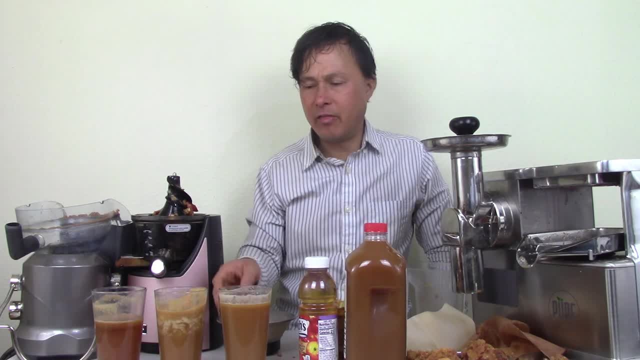 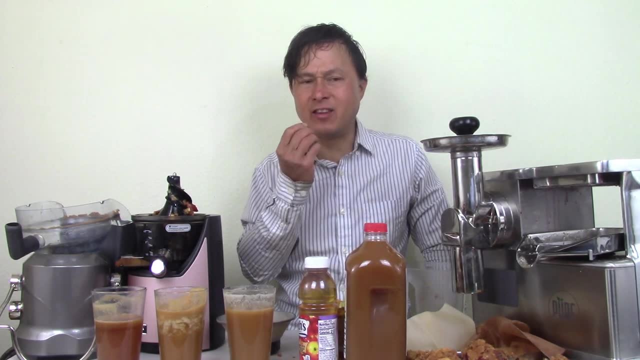 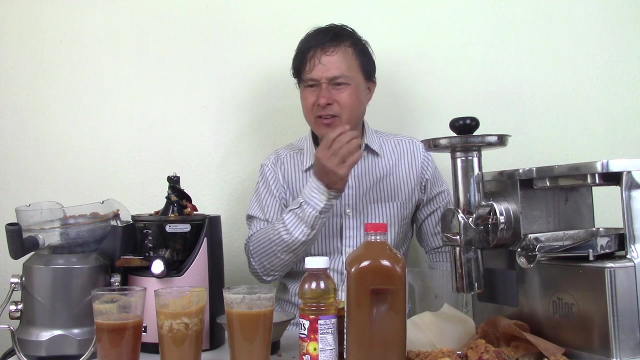 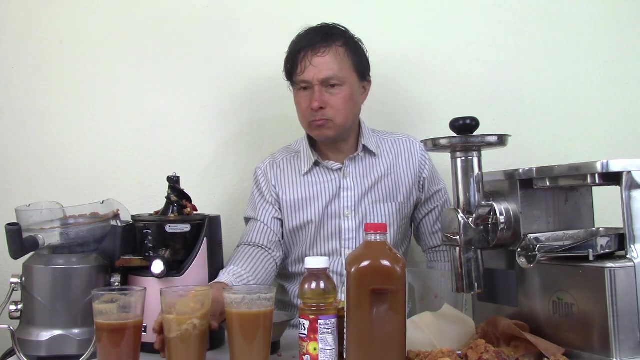 Less particulate than the Breville, surely less particulate than the Kuvings. It still kind of tastes a little bit hard. Maybe that hardness that I'm tasting kind of like bitterness is kind of like the oxidation that's occurred, because when I drink the Kuvings juice it's more smooth. 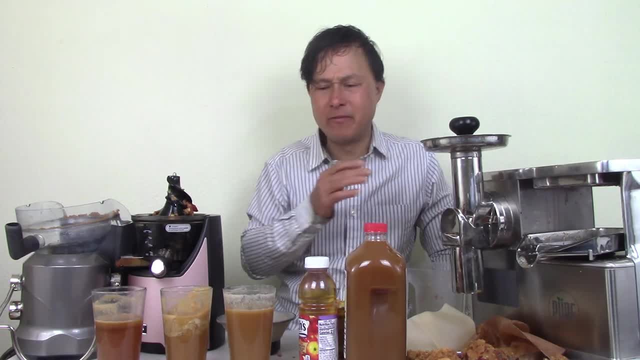 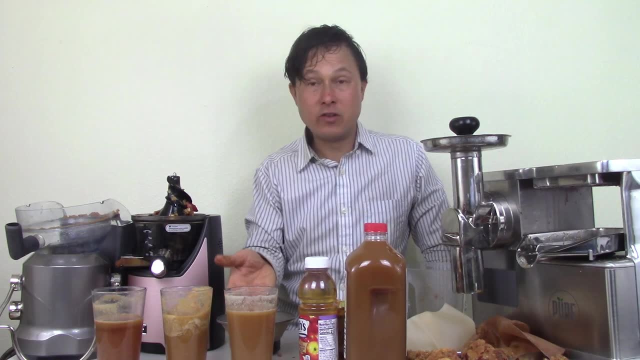 I get like sweetness. I don't get this kind of like bitter stuff. Okay, I don't get this kind of stuff. I personally believe the bitterness is due to the oxidation, because the juice did oxidize—you know, was oxidized the most out of all these three juicers. 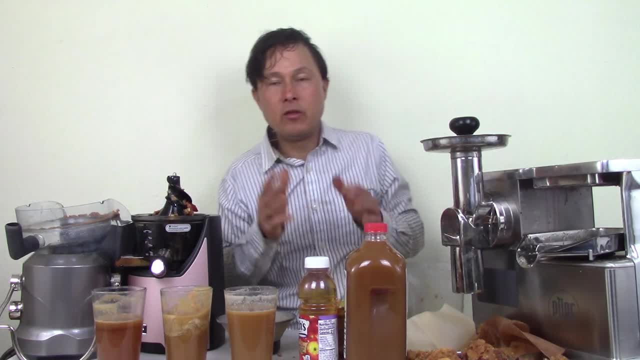 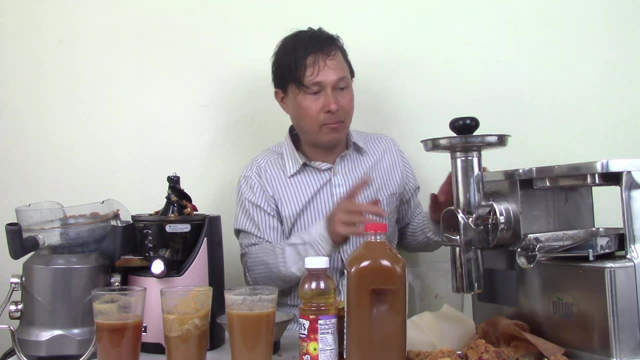 And you know people will. tout the pure is the best juicer. You know, hey, it's the best juicer in terms of yield. You're hard pressed to beat the pure. in most, all cases, There will be few exceptions in terms of yield. 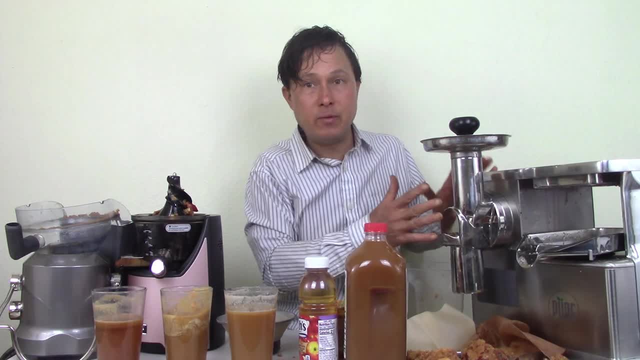 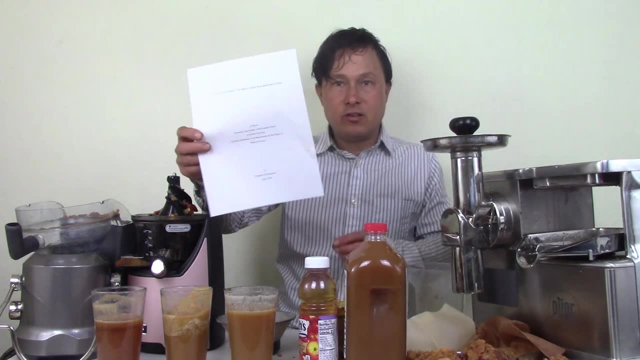 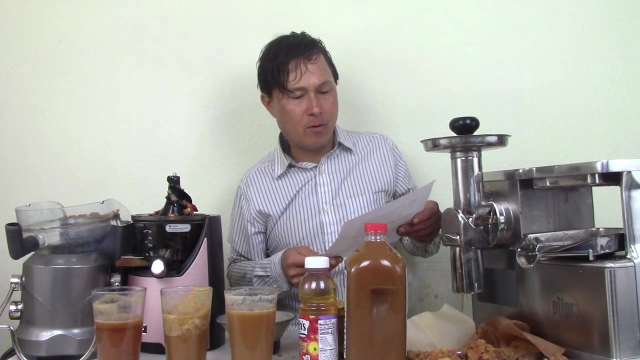 But in the terms of oxidation, in my opinion, you could definitely beat the pure, you know, using a slow juicer. Now, the final thing I want to talk about is I want to talk about this master's thesis that was actually from—it's titled Quality and Stability of Shelf-Stable Pulp-Rich Fruit. 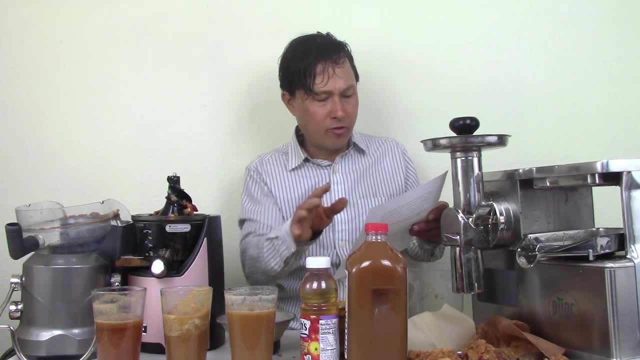 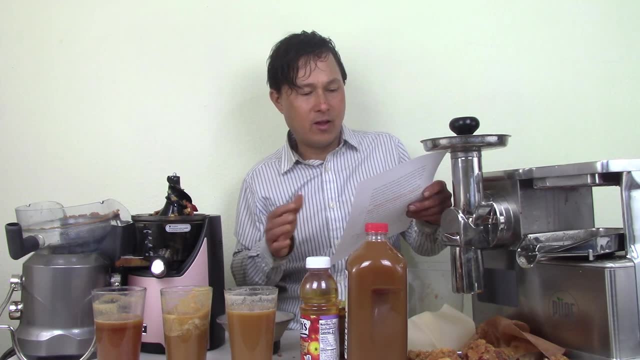 Juice. So they're kind of probably talking about like juices like these that are commercially available, And it's presented to the faculty of the Graduate School of Cornell. So somebody actually had to, you know, write this to have a master's degree in science. 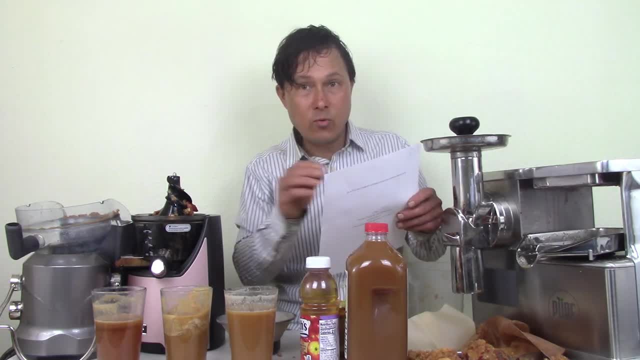 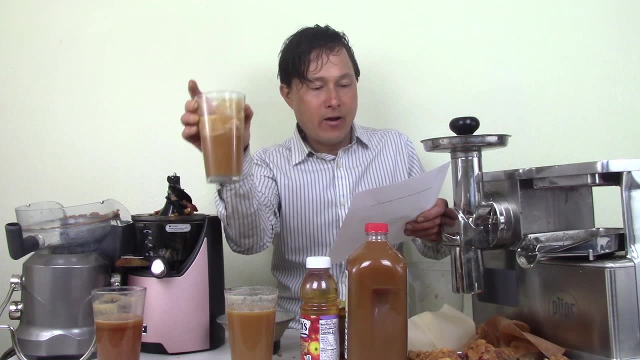 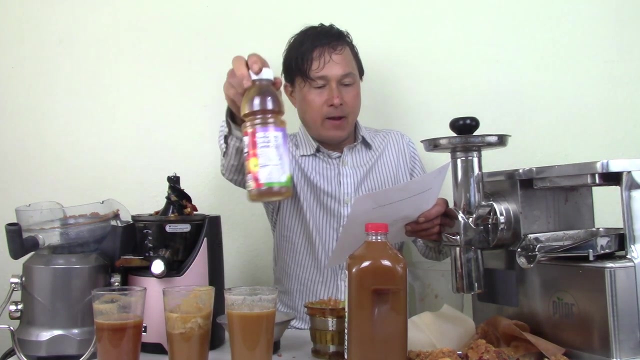 So I'm sure it's fully vetted and legit. Okay, So I want to read a couple of highlights that I've highlighted. Okay, Pulpy juices had a higher phenylonic and anthocyanin content and antioxidant capacity than clear juices of the same fruit type. 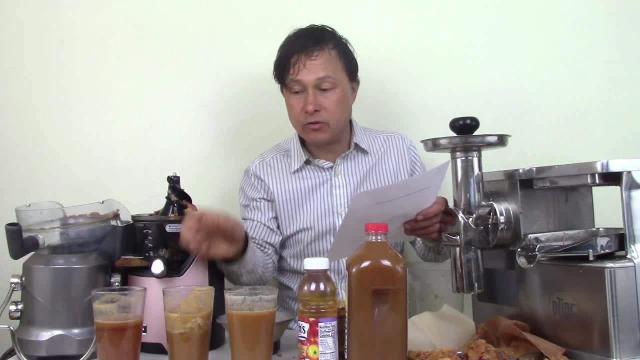 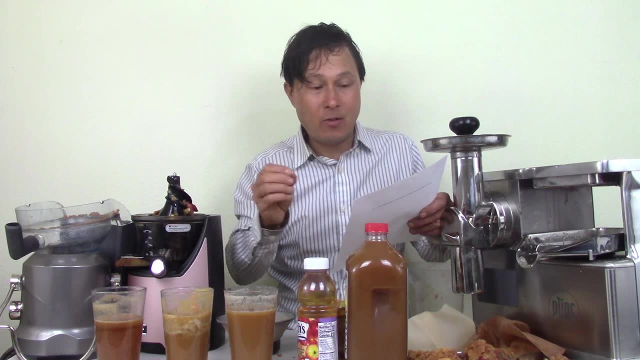 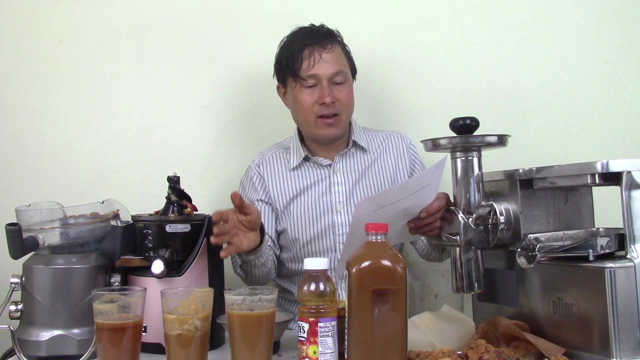 The content was comparable to that of whole fruits. Surely this juice, because it is a nectar- it is thick, you know- has more sible and insible fiber in there. Okay, And this paper? it says there's higher phenylonic and anthocyanin content and antioxidant capacity. 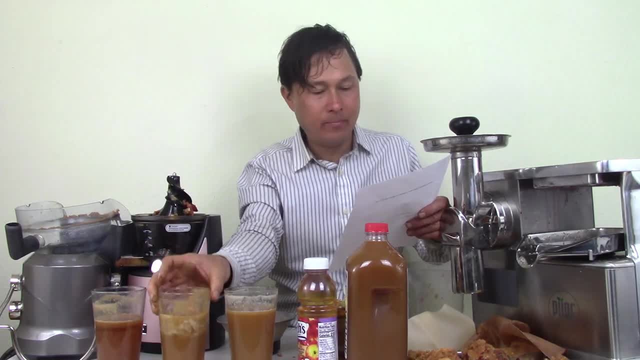 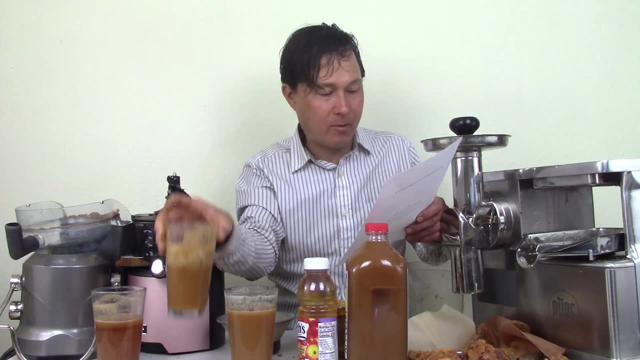 So what does that mean for you guys? That means it's healthier for you guys to drink, right, Let's go ahead and move down Pectin content of pulpy juices—pectin is a sible fiber. It may regulate the absorption of the blood sugar into your bloodstream. 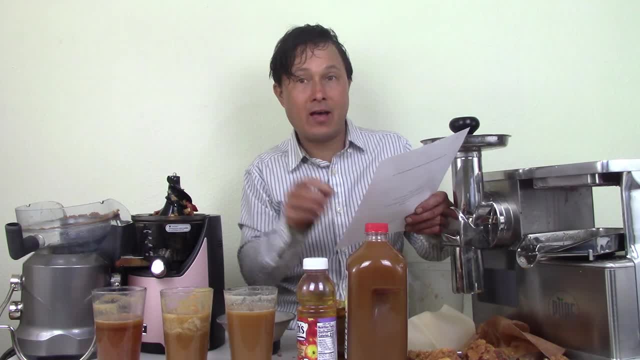 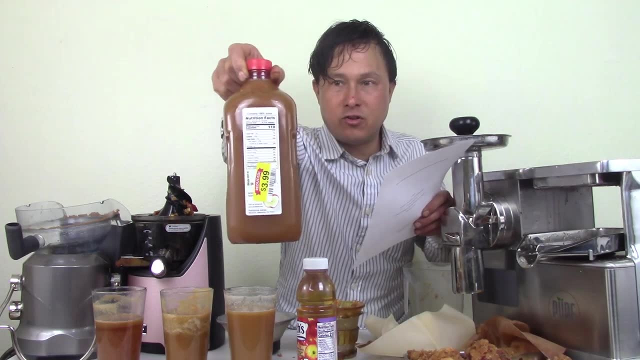 So pectin content of pulpy juices was comparable to that of whole fruits, So the pectin was very similar In the pulpy juices—so this would be more considered a pulpy juice, which is still rather thin, because this juice is actually really close to what the pure is, if you you know. 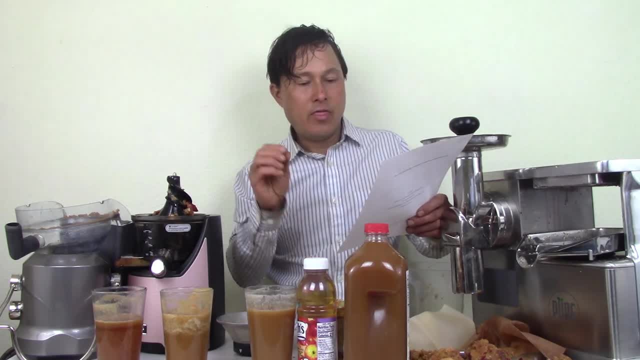 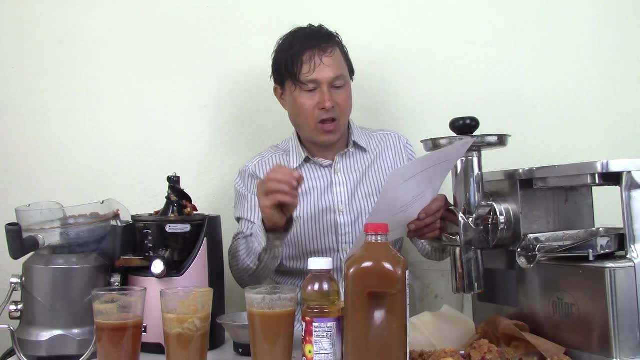 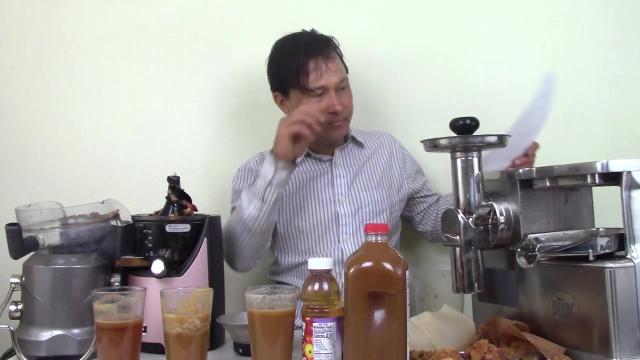 process this even further. Okay, I'll go on. There was almost no pectin in clear juices. Pulpy juices represent a rich source of sible fiber, and one serving contains 0.7 to 11.6 grams of pectin. 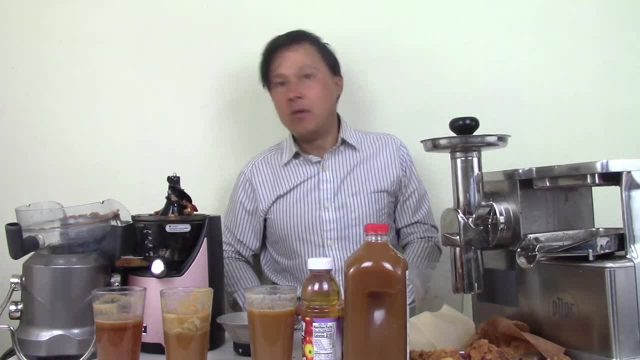 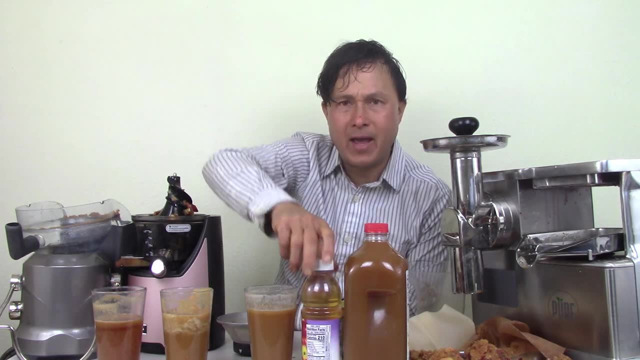 Alright. So what are we learning? You know, Maybe the reason why the apple juices that you buy and the tests that they've done, and why this stuff is so bad and why it's so bad in some of the studies, is because, number one, they might be using a diluted apple juice that still has corn syrup in there. 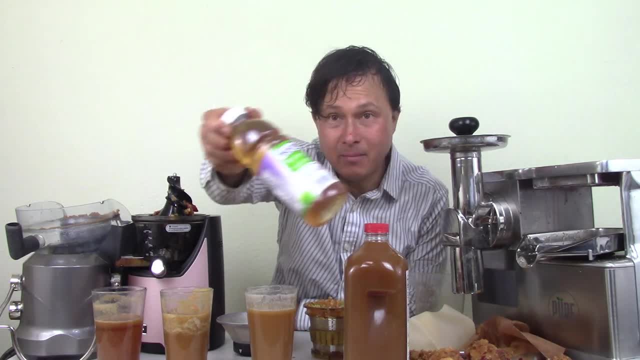 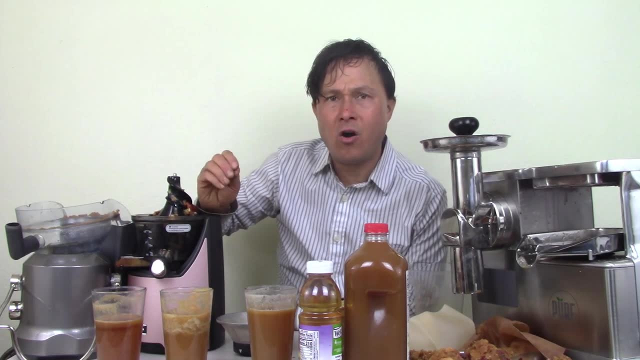 Number two. it is ultra-processed, It's clear. It looks like pee to me and to me it's more about as worth as much as my pee. My pee is probably more valuable technically because they are removing all the sible fiber in there. 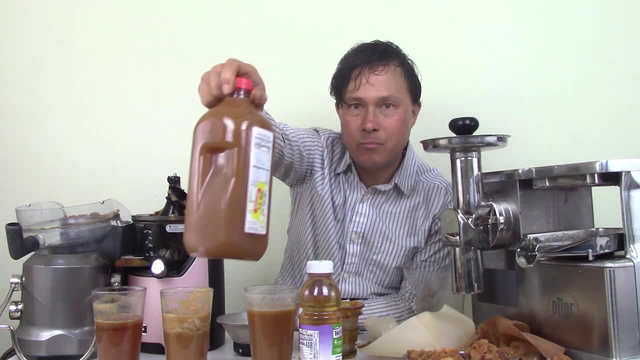 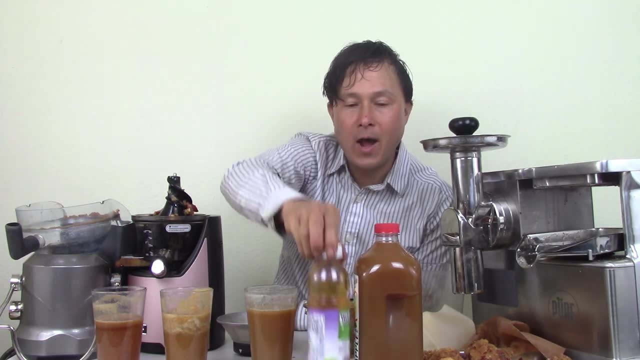 Meanwhile, this juice, you know, is more. It's more rich, more thick, more delicious, has more pulp and polyphenols and pectin in there than this juice. but why not take this juice to the next level? How do you take it to the next level? 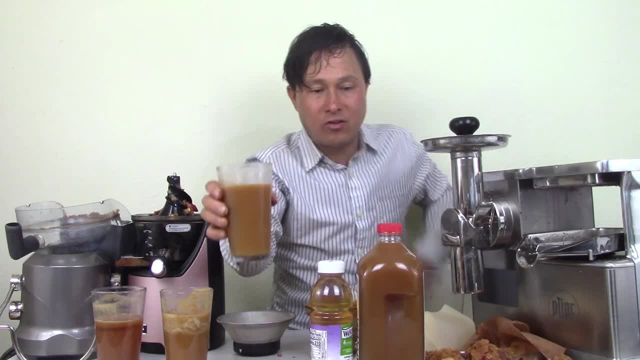 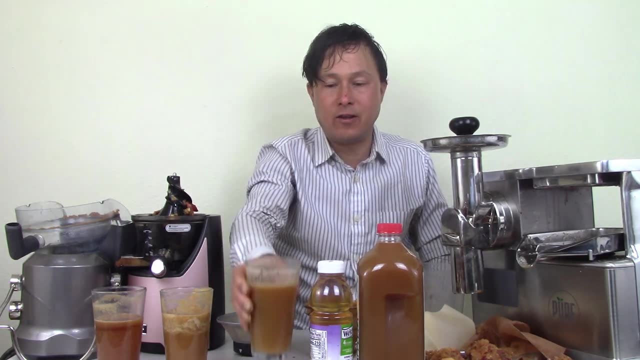 The next level is the pure juice, because basically it's made through the same grinding and pressing process, but you are not pasteurizing it and not ultra-filtering it and you know exactly the process. But if you even want to get better than that, in my personal opinion you're going to have 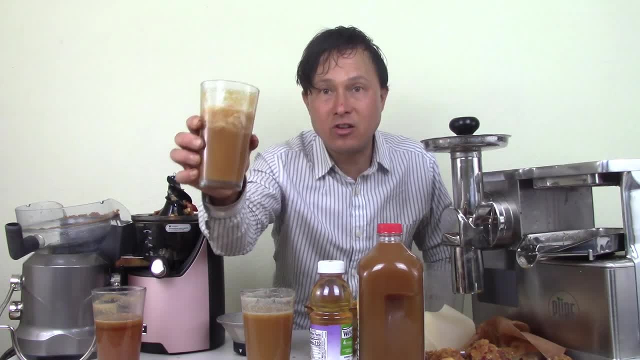 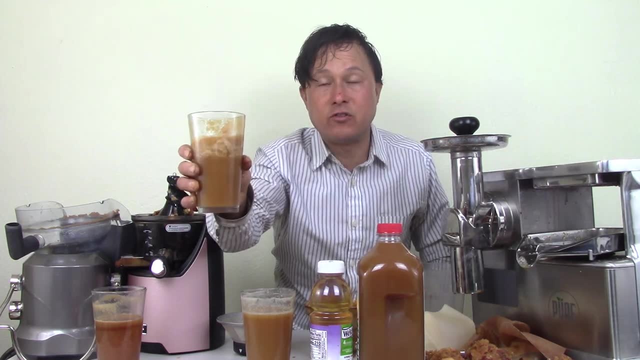 to go through the same process. Okay, Number three: you want to go with a slow juicer. The slow juicer, this is a thick juice. If you want a thick juice, don't get a slow juicer when you're juicing fruits. 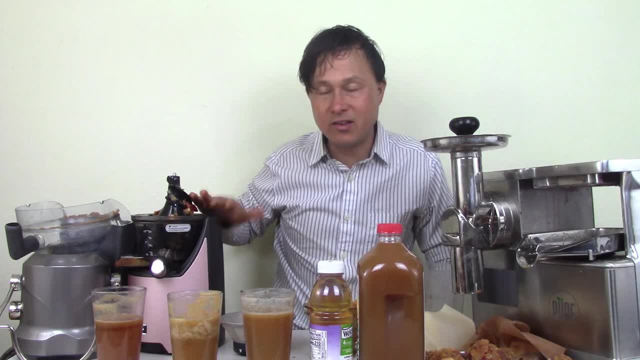 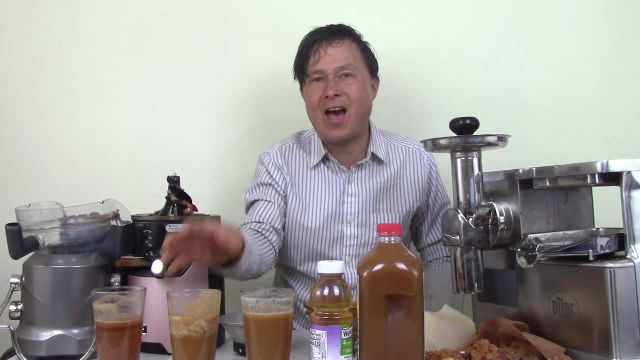 Now, if you're juicing vegetables and greens and celery, this is not going to be that thick. Apples have lots of the pectin and that's what's causing this thickness, and especially as the apple gets softer, this juicer is more effective at extracting it out. 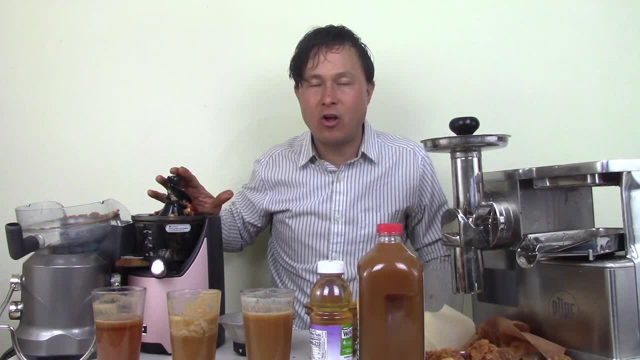 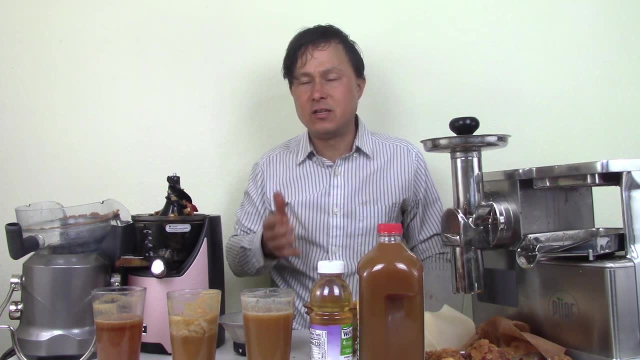 In addition, in my personal opinion, you know, this juicer style is also more effective at liberating some of the different polyphenols and nutrients from seeds than other style machines and maintaining, you know, more of them, due to the low RPM and minimal oxidative. 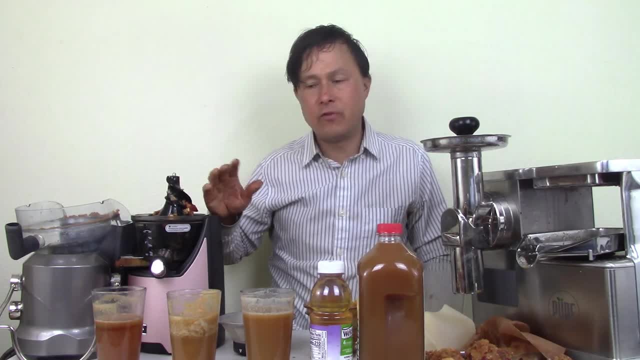 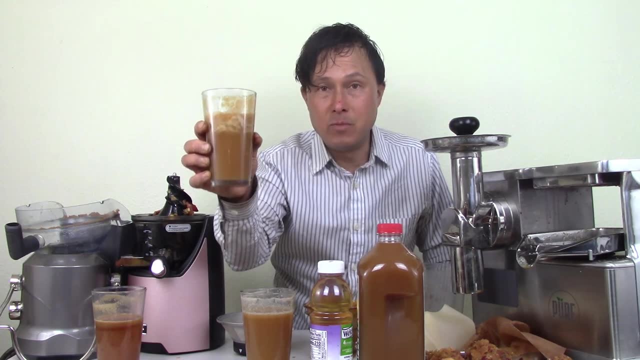 damage and the larger whole size. It's very important. So, yeah, this will give you the most fiber you know, soluble and insoluble. also, probably the most antioxidants and polyphenols you know, and it's these components that can help. 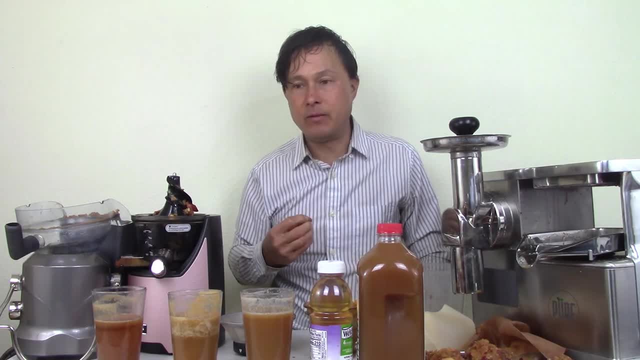 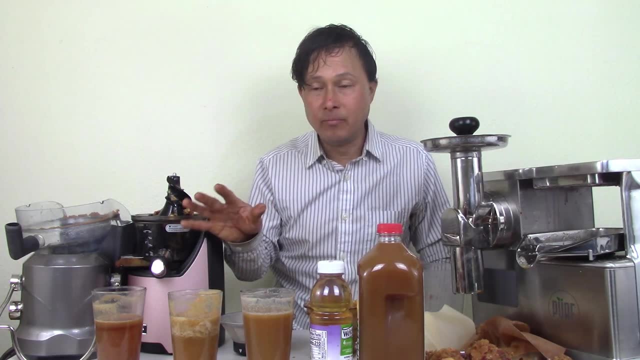 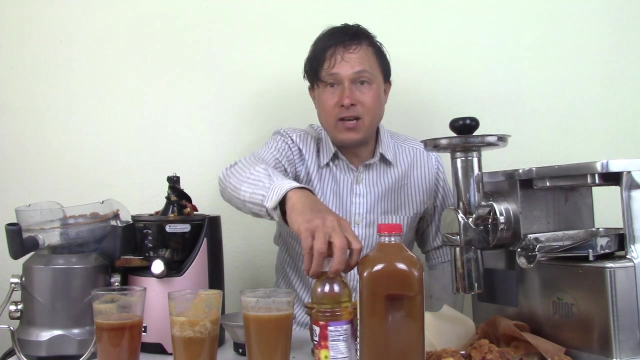 regulate the blood sugar, of the sugar in our blood. Not that I'm going to ever recommend drinking straight fruit juice, as I did today. You know, surely, if you know you have a child and they're drinking Coke, surely an apple juice made in the Kuvings is way different than the Welch's, way different than the 30%? 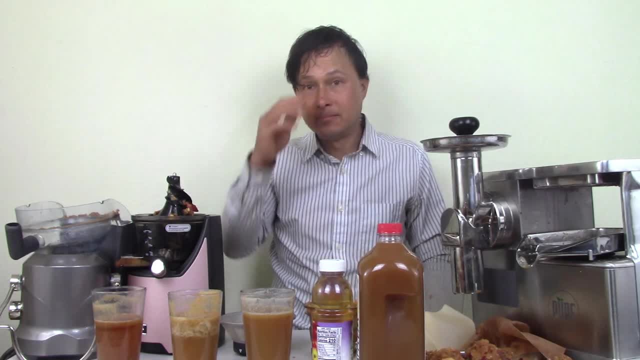 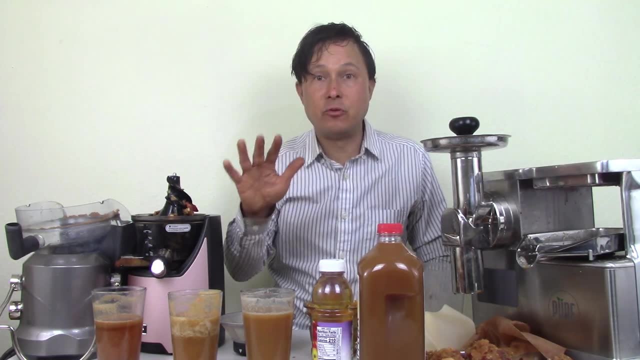 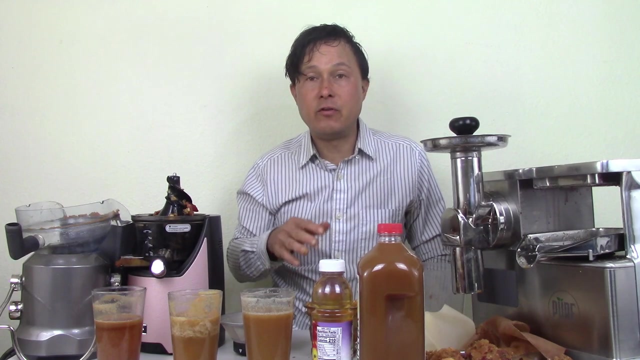 you know juice, drink or cocktail that's being sold, But you know my personal opinion- and I rarely juice straight fruits- is to drink vegetable juices. Green juices, including leafy green vegetables. you know, green vegetables such as celery and also even roots such as carrots, are highly nutritious and if you've got to juice those, 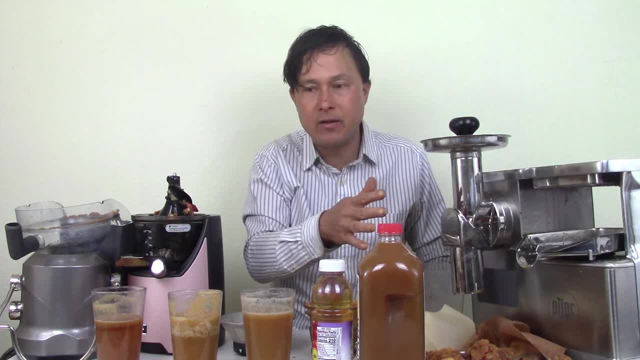 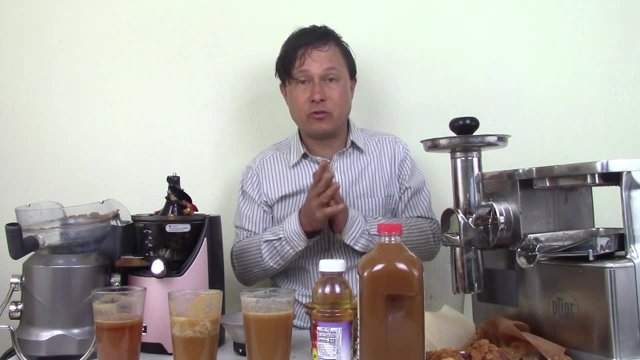 guys put a couple apples in to make it taste good, I wouldn't worry about it, But I want you guys to use the best juicer to make the best apple juice. So hopefully, after watching this episode today, you learned about some of the different studies. 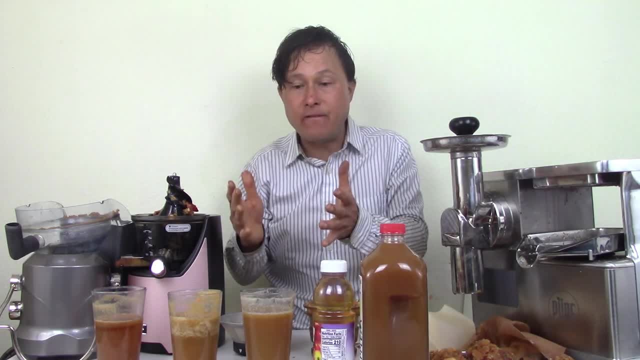 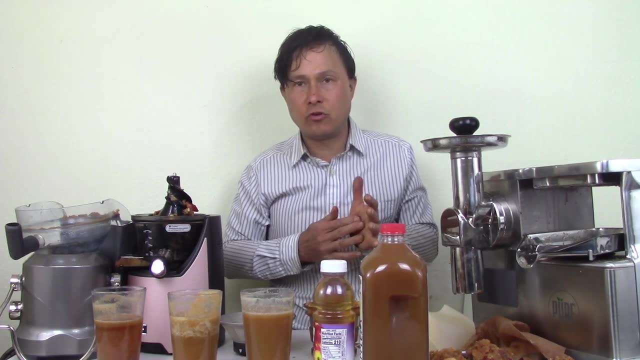 and some of the different fiber content in the juices, some of the different polyphenol content. Learned more about how long it took to use each of these juicers and some of the pros and cons of each juicer will make when juicing specifically these softer apples that I have. 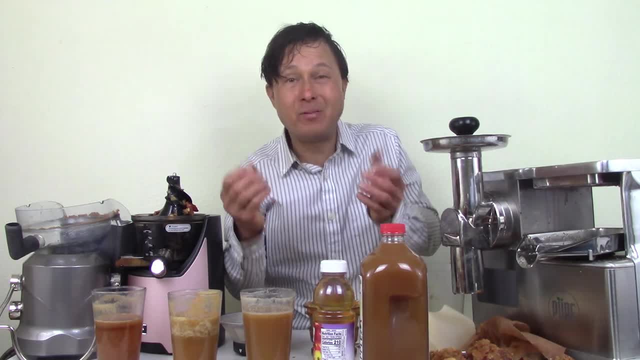 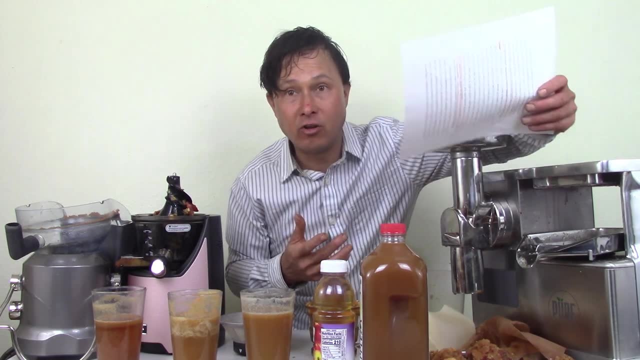 to date. If you guys enjoy my content and want to support me, please make your juicer purchase at discountjuicerscom. That allows me to continue to, you know, do the education to look up scientific studies that I do almost every day. you know, to buy my apples to make you guys these videos. so 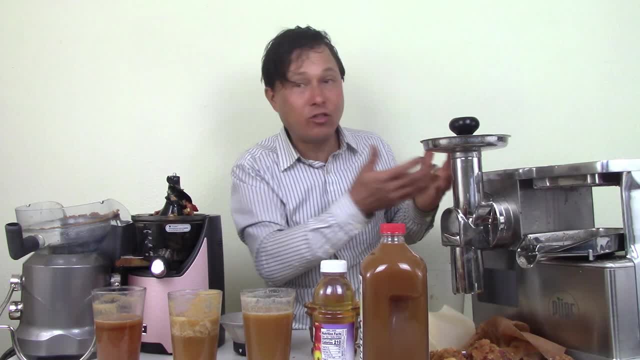 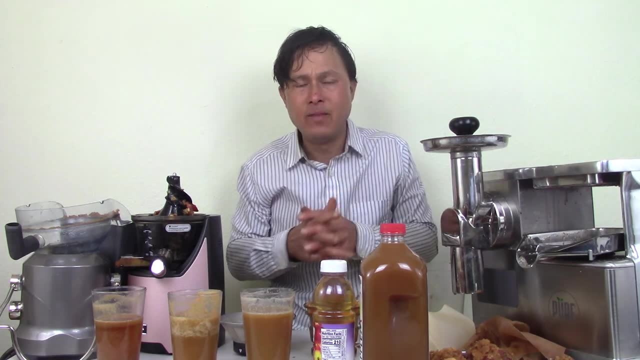 I could share with you guys knowledge- Literally- that you're not going to regret. You're going to find it unless you dig through journal studies and have been juicing for a long time and have all the experience I do. I'm the number one juicer expert in the world and I'm here to ensure that you guys get the 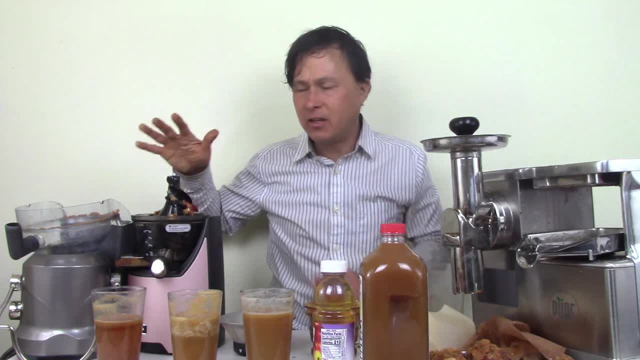 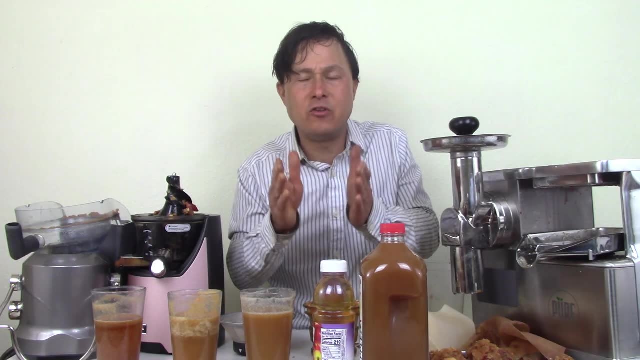 exact right juicer. I have over 500 videos on this channel comparing this juicer to this juicer, this juicer to this juicer, all different kinds of comparisons, so that you will get the right juicer style for you. I'm confident that I have the right juicer style for you, but you guys need to figure. 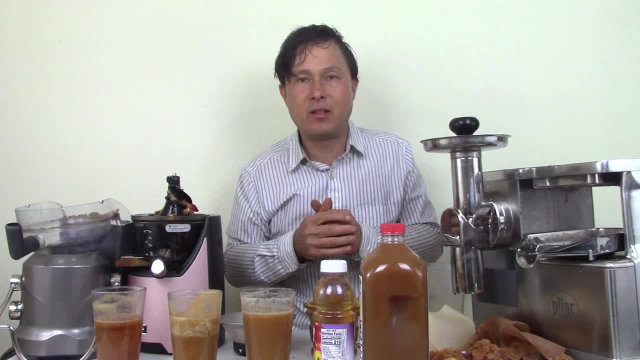 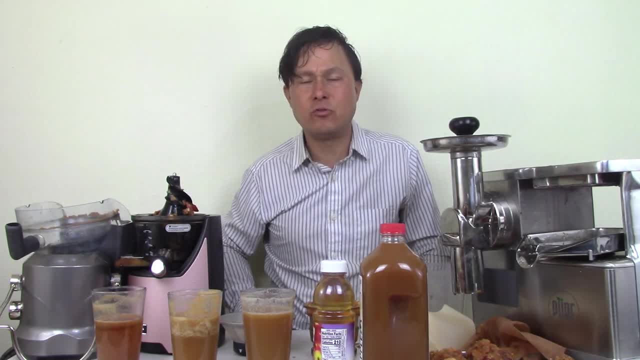 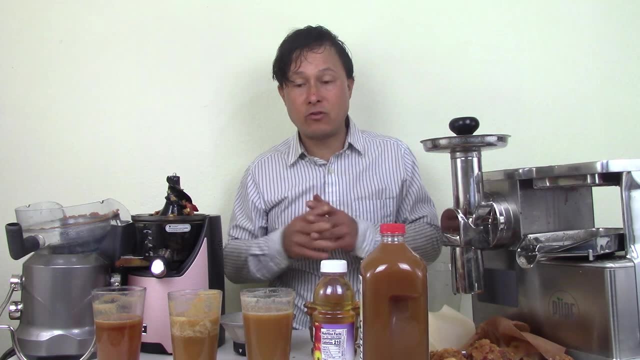 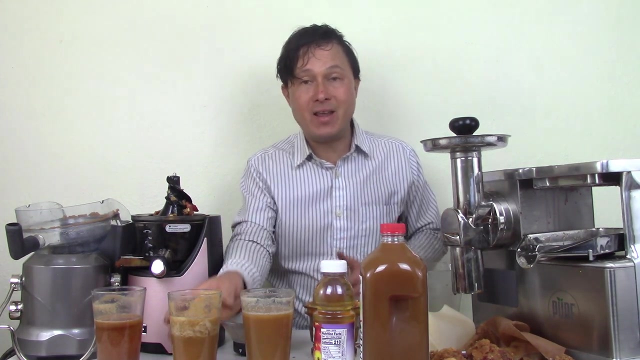 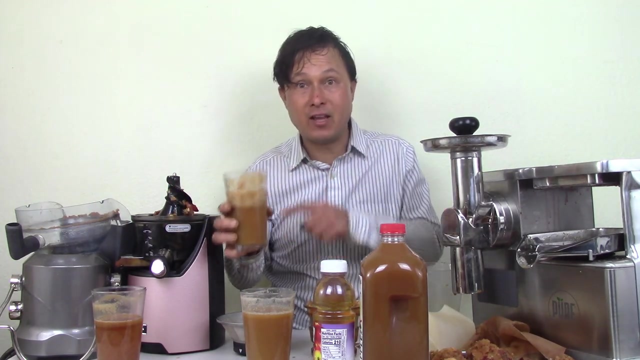 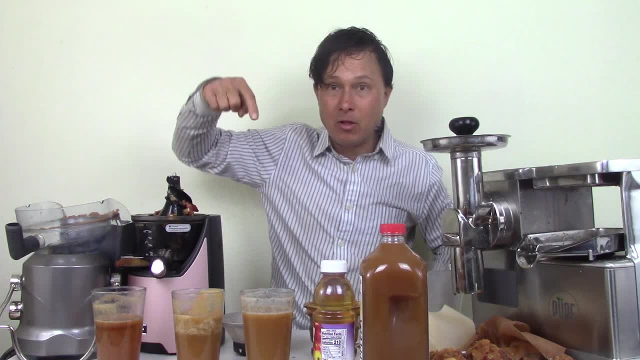 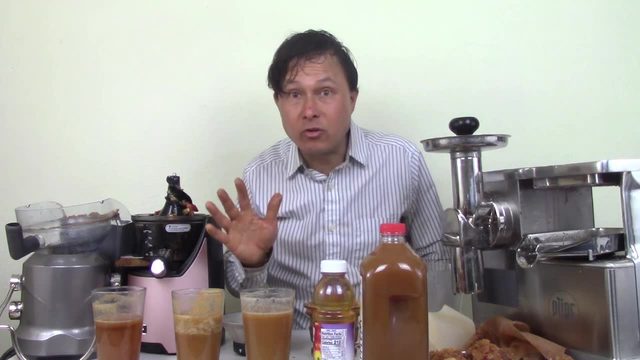 Bye, Bye, Bye. link down below if you want to get this exact machine that I used today: the Kuvings EVO820.. If you guys enjoyed this episode, want more videos like this, please be sure to give this video a thumbs up. 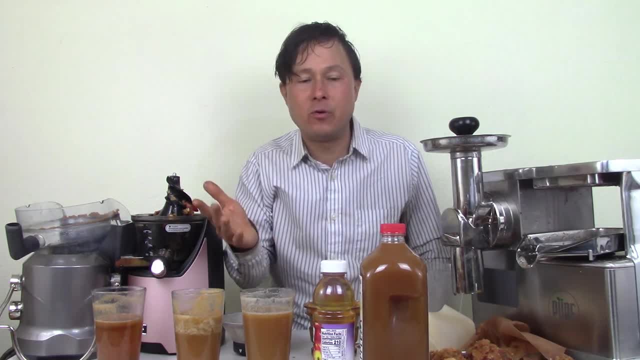 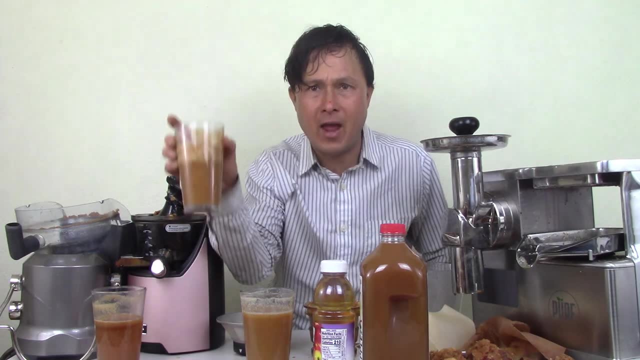 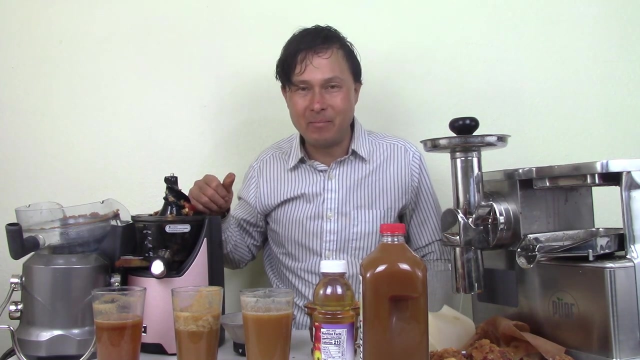 Also, please be sure to share this video with others so that they can be more familiar with the different kinds of apple juices and why some apple juices may actually not be that healthy for you and, more importantly, learn about the healthiest apple juice that you guys can make at home, you know, with organic apples like I used today. 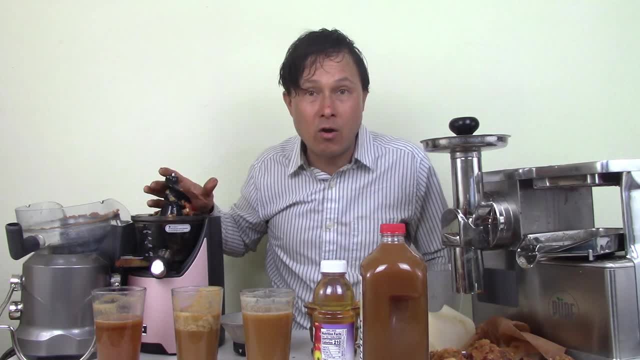 Also be sure to click that subscribe button, you know, so that you can be made aware of my new and upcoming episodes that come out every five to seven days. you never know where I'll show up or what you'll be learning on my YouTube channel. 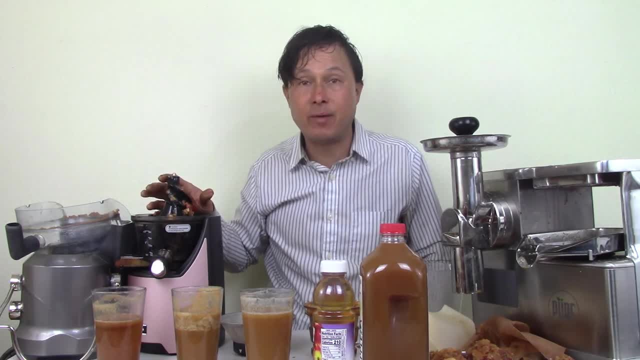 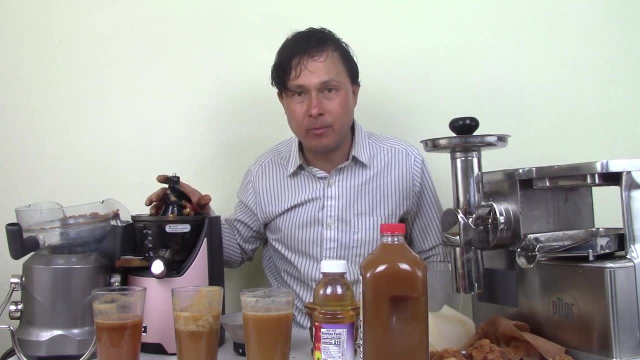 Make sure you click the little bell so you get notified as my new videos come out. And, finally, be sure to check my past episodes. my past episodes are a wealth of knowledge- over 500 episodes at this time on this YouTube channel dedicated to comparing and contrasting. 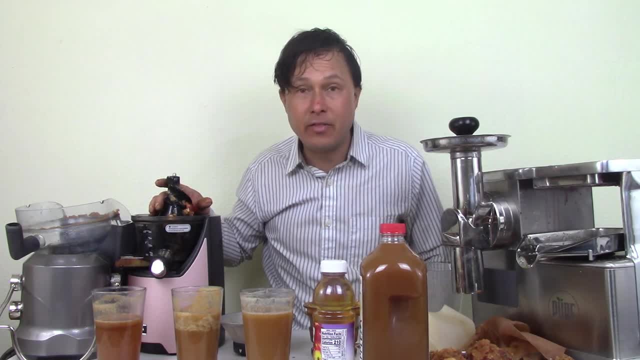 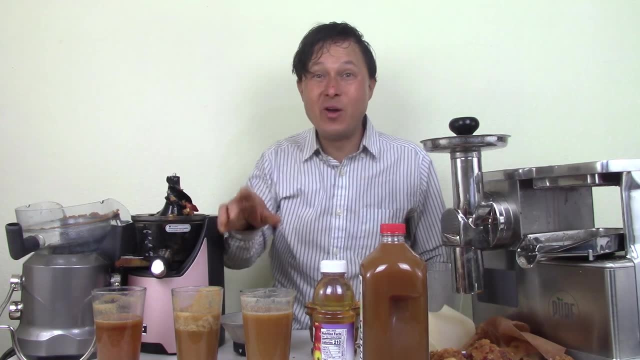 all the major juicer styles and juicers with you guys that are available in the United States, so that you guys can get the exact best juicer for your needs. So with that, my name is John Kohler- with discountjuicerscom. be sure to visit discountjuicerscom. 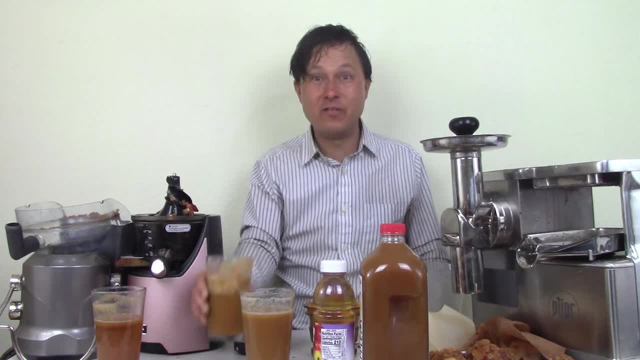 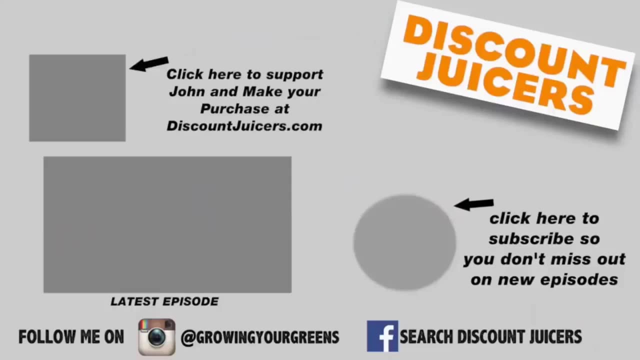 slash YouTube for special promotional offers for YouTube visitors. I'll see you next time. Bye-bye.